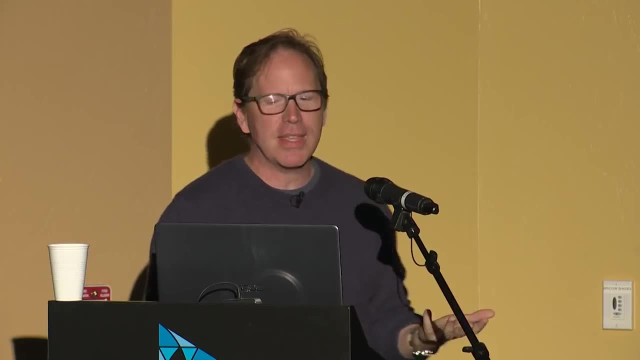 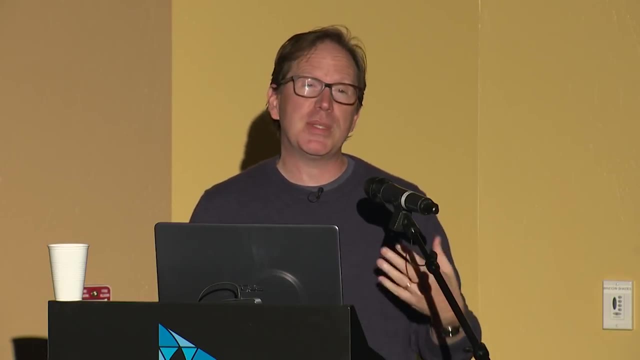 them from one to zero and then everything's good. and how could that possibly involve ethics? And part of it, I think, is about how we've evolved, how we think about cybersecurity, but, in particular, how I and my colleagues have focused on researching cybersecurity. So to kind. 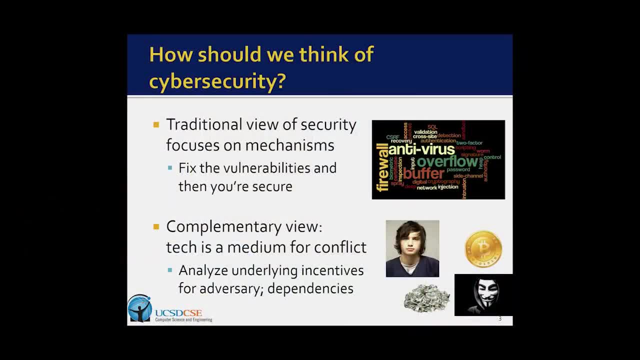 of give some context on that. traditionally, the way we've thought about computer security is in terms of mechanisms. There are some vulnerabilities in our systems and if we fix them then we're secure. It's kind of the equivalent of the holes in the dike, If you put your finger in all the 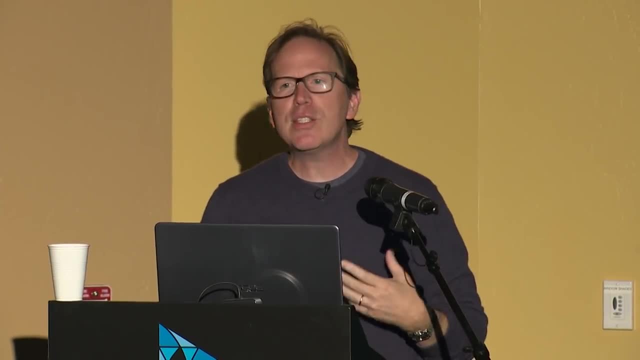 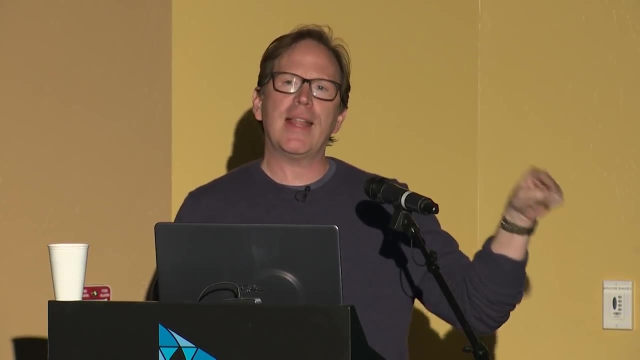 holes, then you don't have a problem anymore and then we'd be safe. And in a certain kind of banal sense, that is absolutely true Post hoc, after everything that went wrong, if we said, well, only that thing hadn't happened, then we would be fine, and that is absolutely correct. 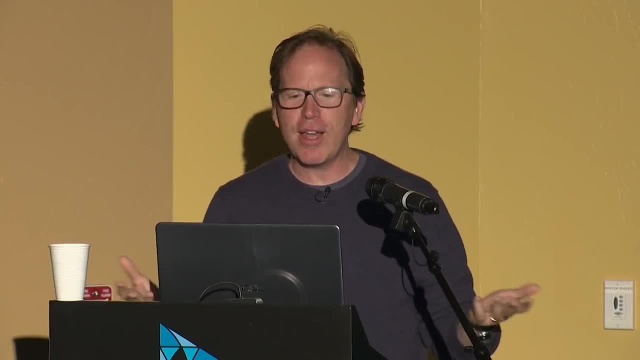 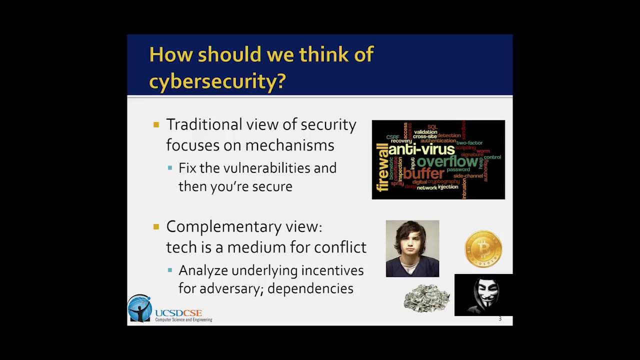 but does not capture the reality of what is going on on an ongoing basis, And that is that there is this complementary view. Yes, there are these mechanisms that have to be improved. We have to remove vulnerabilities, We have to make things more robust, We have to make. 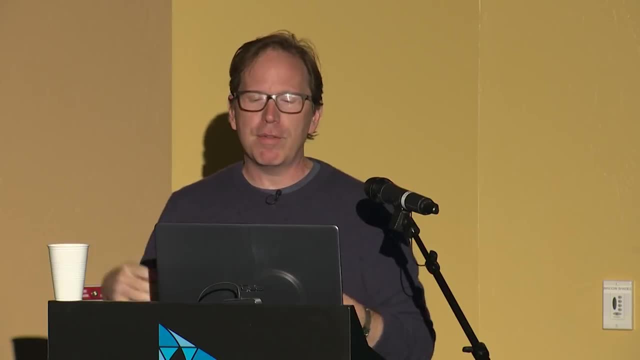 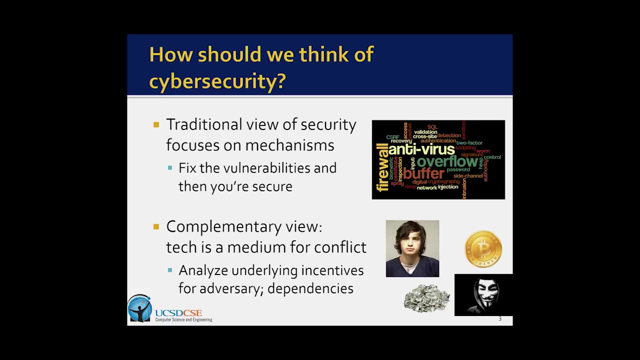 them survive certain classes of attack better. but the other complementary view is that the technology is simply a medium in which this conflict is taking place. right, The reason we have computer security problems is because someone is out to get us Bottom line. right, If they. 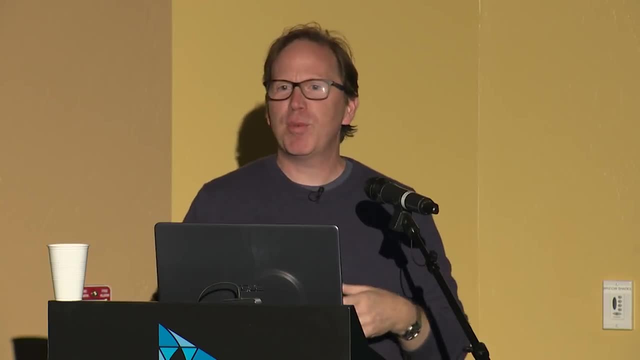 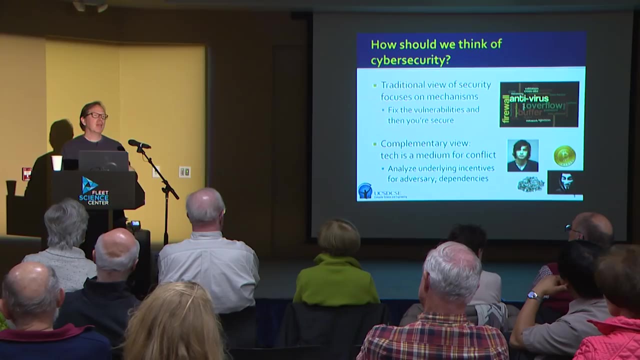 weren't, we wouldn't care, right Without burglars, we wouldn't care about locks on the door, right. So the reason we care is that there is a conflict. There's a lot of different kinds of conflict, but fundamentally there's a conflict and that means 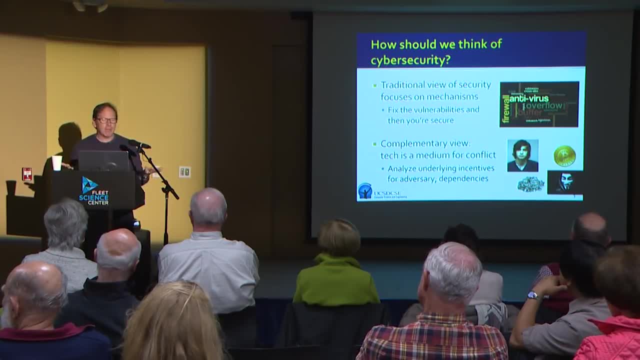 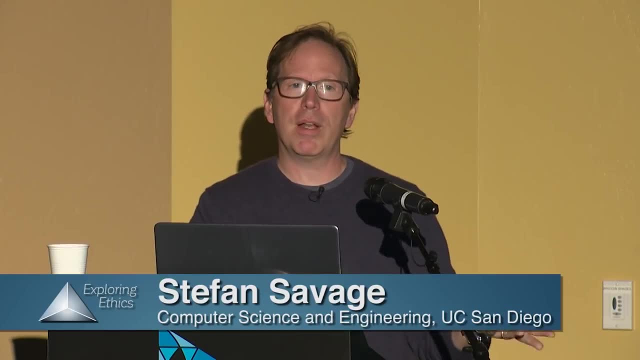 there's some other party that is interested in doing things that are adverse to us, and the technology is the medium that that plays out, and they can shift from one part of it to another, and so this complementary view of looking at computer security, which is one that we spend a 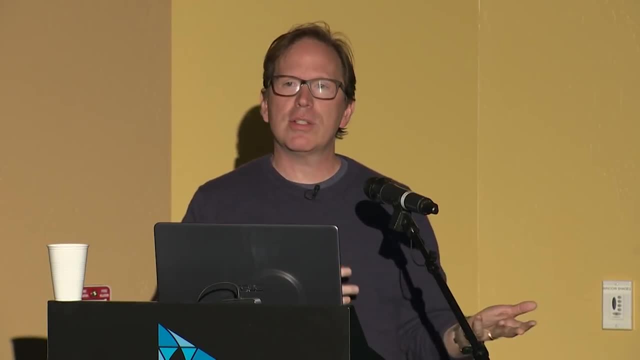 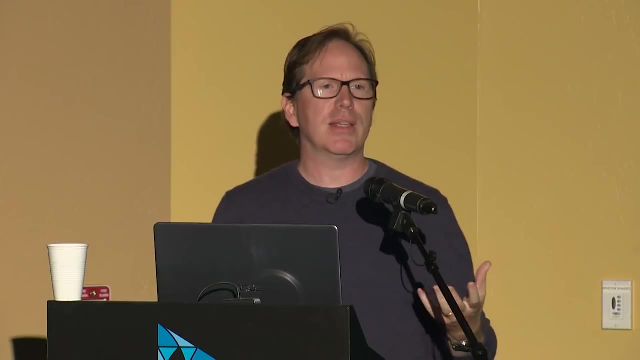 lot of time looking at is: can we try to understand this from the standpoint of the adversary and not just from the standpoint of the mechanisms, and what are their incentives and dependencies and how does that play into how we can all be safer? And so the core idea that motivates a lot of this: 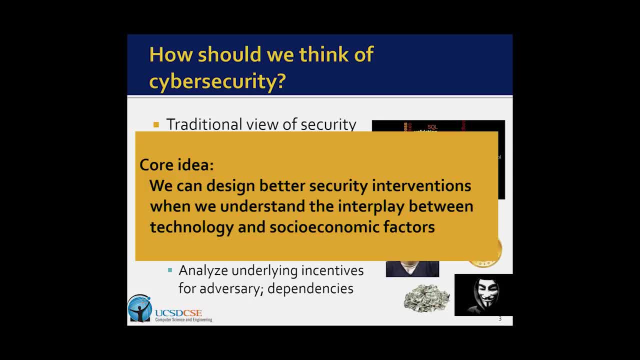 work, some of which I'll talk about today, is that, look, we could maybe do a better job designing security interventions if we understood what are the interplay between these technical factors and these socioeconomic factors, and that latter part, where you start touching people. that's where we 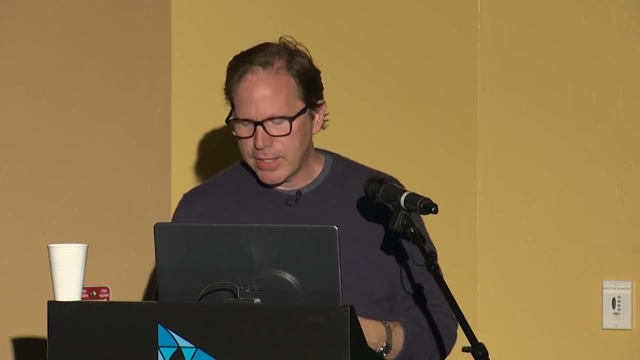 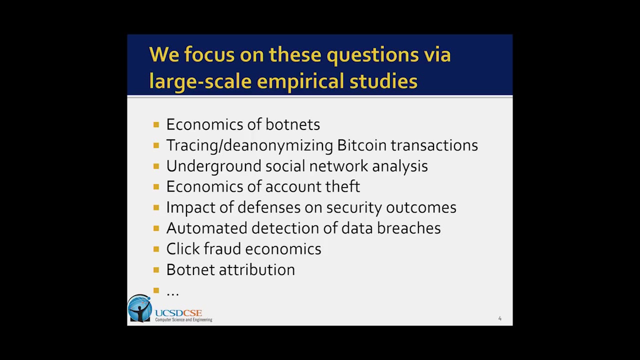 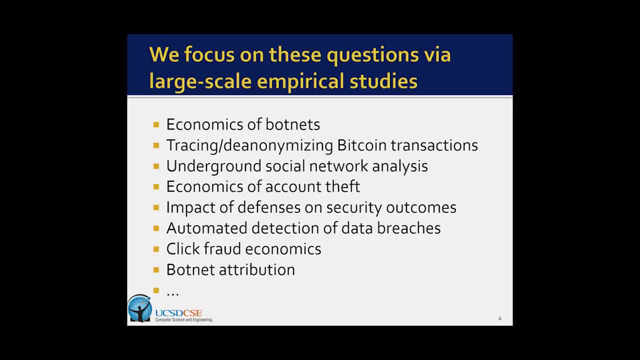 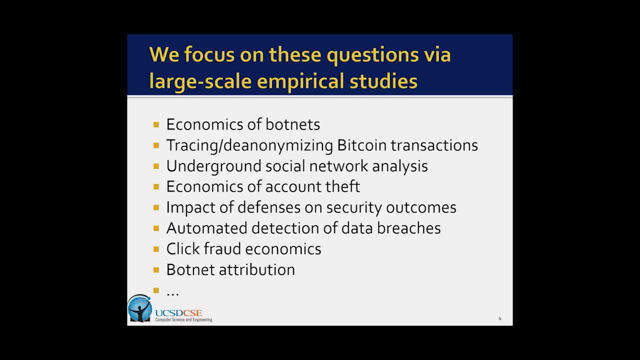 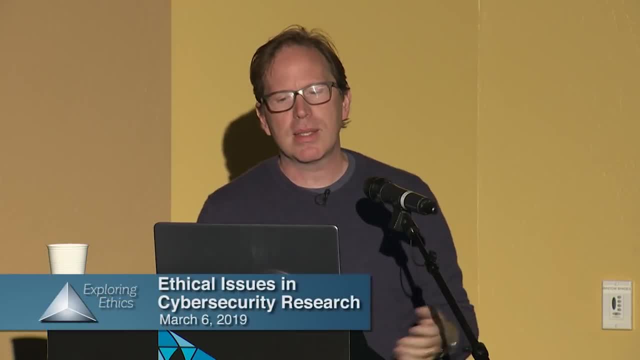 understand things like: okay, so like: what is the economics of malware? People who are writing malware, how do they get paid? How much do they get paid? What's the return on investment? How does that work as a business When someone steals your account or there's a data breach? well, how does 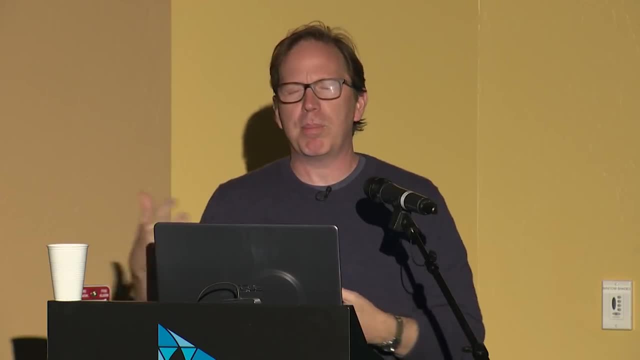 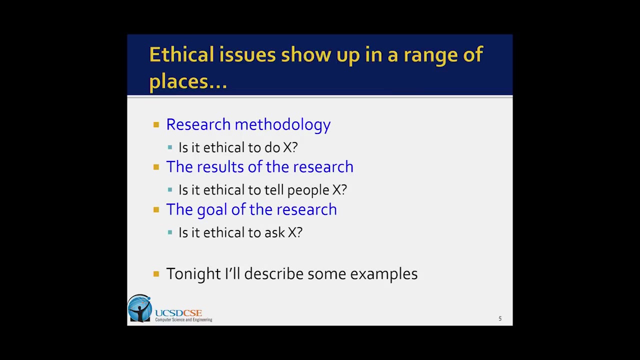 that work Like: who gives it to whom? How does it get handed off? Does someone contract for it? You know all of those kinds of things. So ethical issues show up in a ton of places it turns out, none of which I anticipated, and they have to do with. 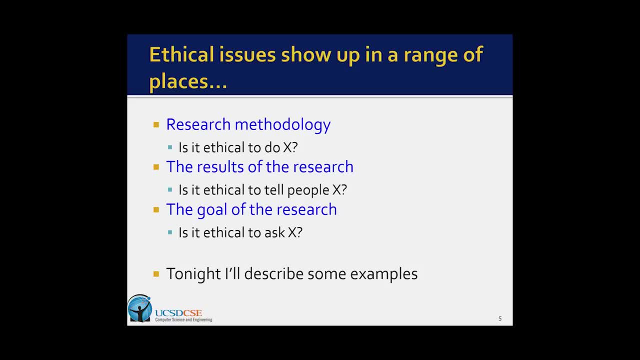 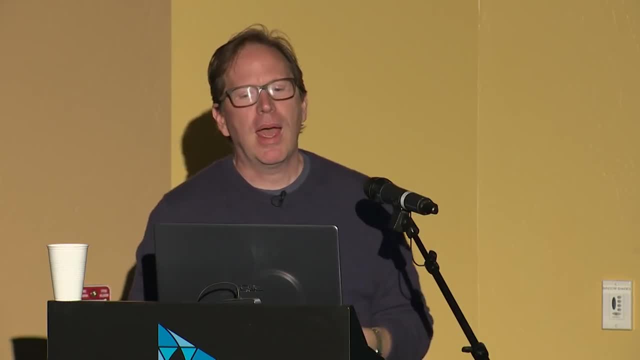 things like: is this thing you want to do to figure this thing out? is that an ethical thing to do That measurement you want to make? is that? can you do that measurement in an ethical fashion? Then sometimes you get results of research saying: would it be ethical for you to tell people the 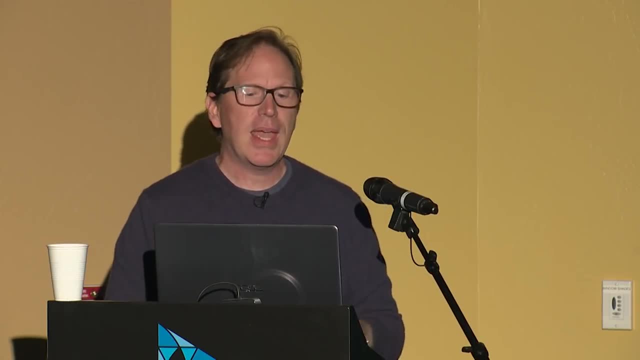 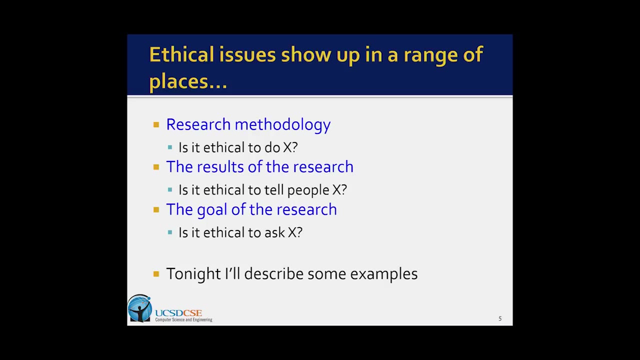 results, Are the results themselves potentially problematic, And sometimes it's the goal of the research. Is it ethical to ask the results? Is it ethical to ask the results? Is it ethical to ask the question such and such? And I'll touch on some examples of some of these. I will highlight: 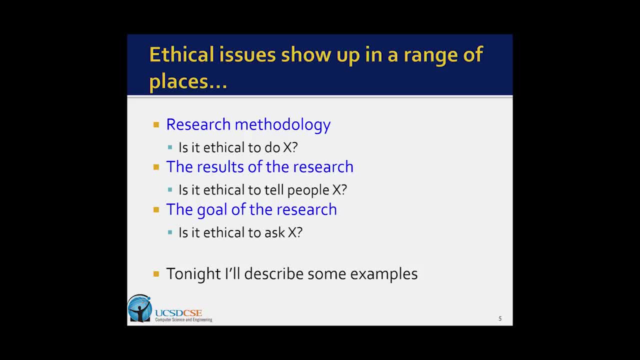 where there's an issue, but I will not necessarily talk about the issue here, and we'll do that in kind of the panel session, So I'll leave it open for you guys to think through what some of the other issues that I may not have considered are. All right, So I'm going to really talk about. 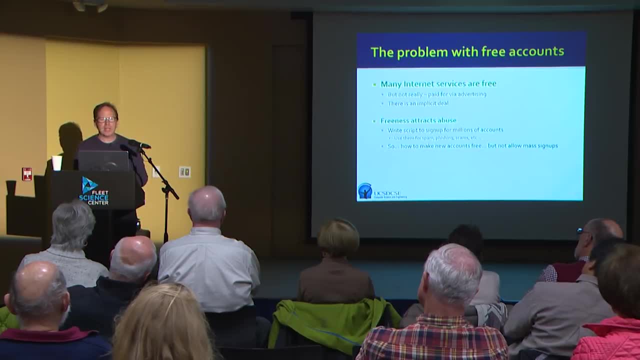 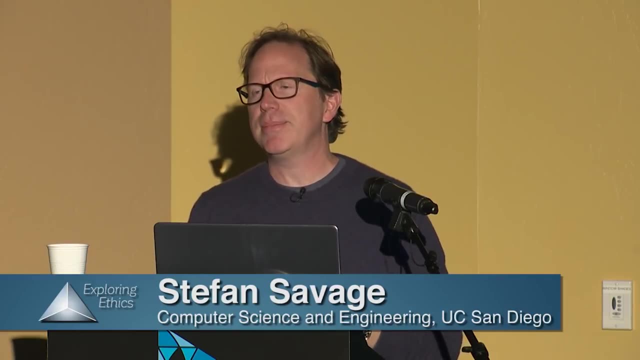 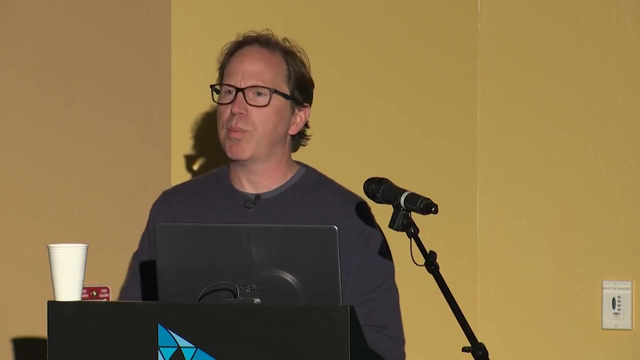 three different examples that touch on some of the different things we've run into. The first one is some early work that we did. That is about a particular mechanism that we use online that you're all familiar with, called a CAPTCHA, And CAPTCHAs are there to deal with the problem that we have with free accounts, Whenever you make. 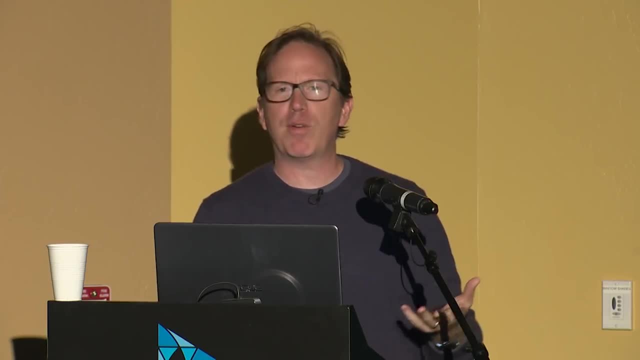 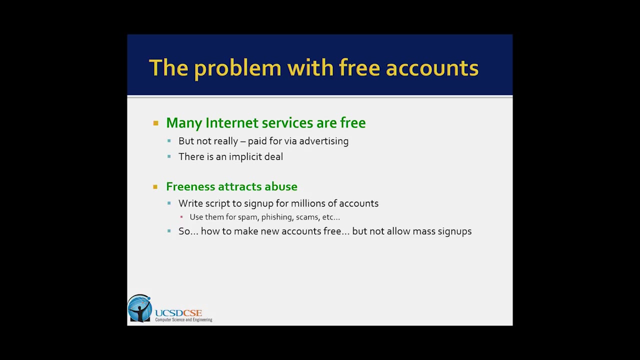 something free. it's not really free. It's being paid for with something else, and typically that's advertising, And so there's an implicit deal that whenever you get a free account, it means that you are a unique set of eyeballs that is being exposed to some advertisers who are ultimately paying for. 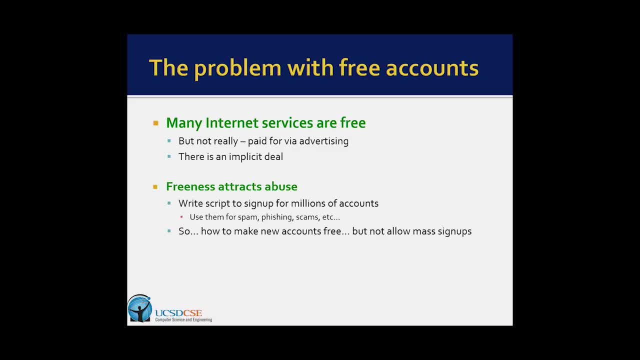 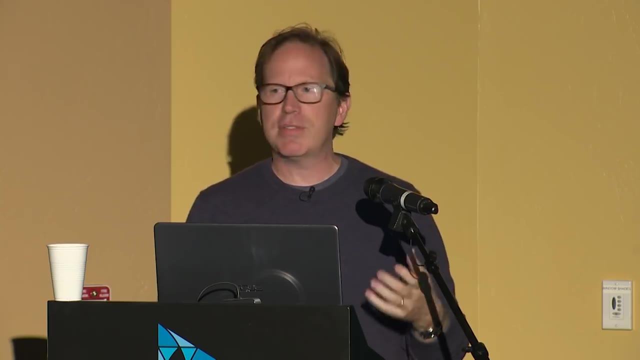 all of the computers and so forth that make this work. So this would work great. except that if people can sign up for millions of these things in an automated fashion, then it undermines that implicit contract that's going on, Because then if someone could sign, 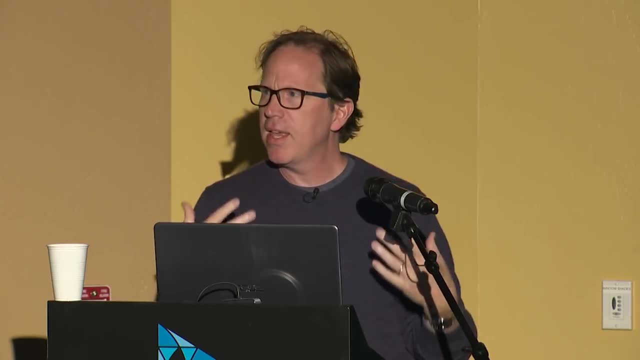 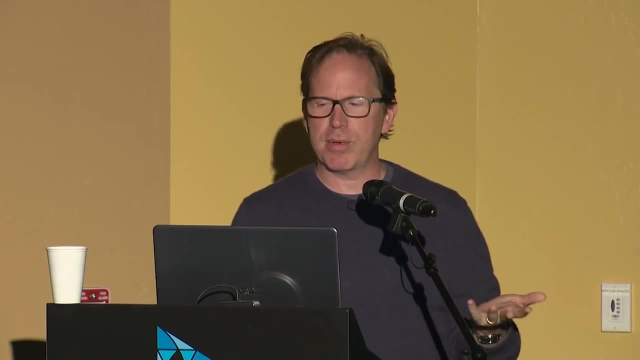 up for a million Gmail accounts and then send lots of spam for them. that no longer is. you know, you can't sell ads for spammers, Like no one wants to sell ads to spammers, And so the solution that one of the 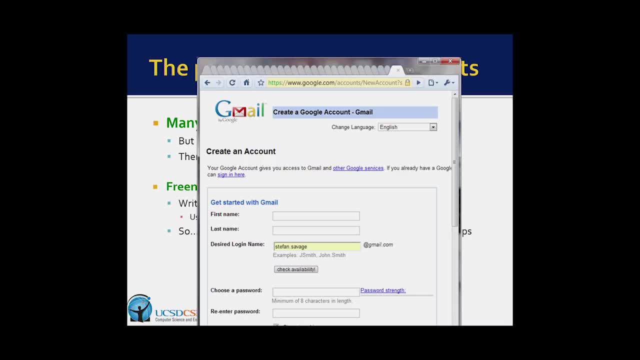 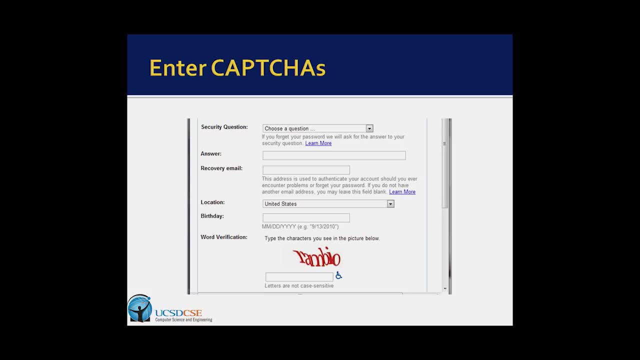 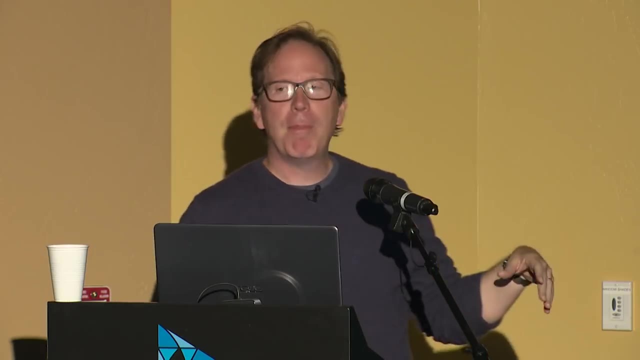 things industry came up with is this thing called a CAPTCHA. You sign up for a new free thing and it gives you some outrageous little. you know, doodad, that you have to interpret, where the premise is that this is something that is a human can look at and figure out. at times, I wonder, but that it's hard for a computer to do, And so that 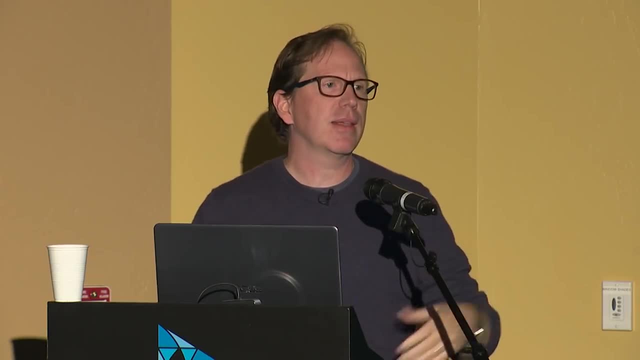 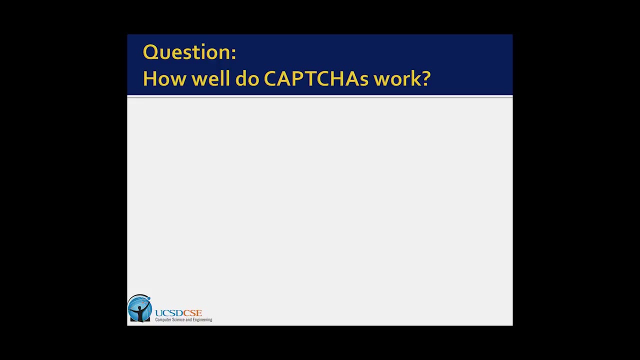 fact that a human needs to do the work will prevent it from being automated and create these mass sign-ups. All right. So you might ask the question: how well does this work? Do CAPTCHAs work? And this is actually a fairly tricky question to ask about any security mechanism. So security. 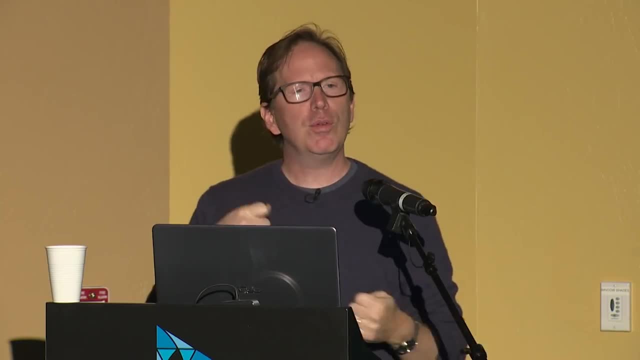 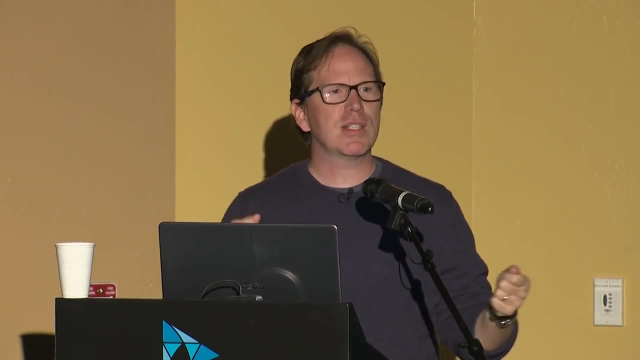 metrics are really tough. We don't know how to measure security. If you go and say, well, should I buy Norton antivirus or McAfee antivirus, And how many units of security does this one offer versus like there's no such thing? There's no such. 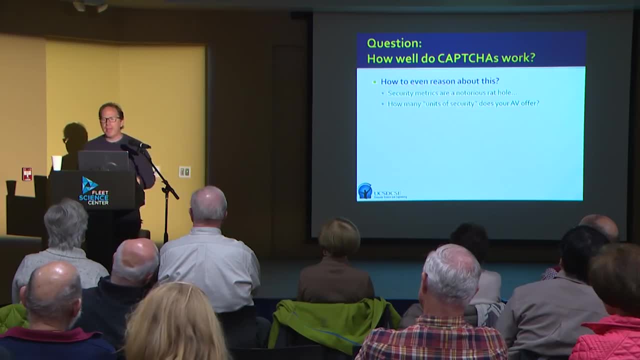 number that exists. We don't know how to measure that. So the way that we approach this was thinking about it economically, because it turned out that as soon as you sign up for a new free thing, you're going to be able to do it. 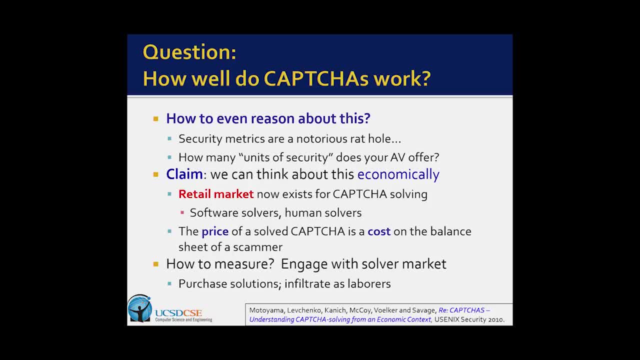 So what did we do? We introduced CAPTCHAs. The bad guys were like: oh crap, we got to solve CAPTCHAs. So it turns out that there is a retail market for solving them, so that criminals can go and still do their mass sign-up of accounts. So what we might say if we 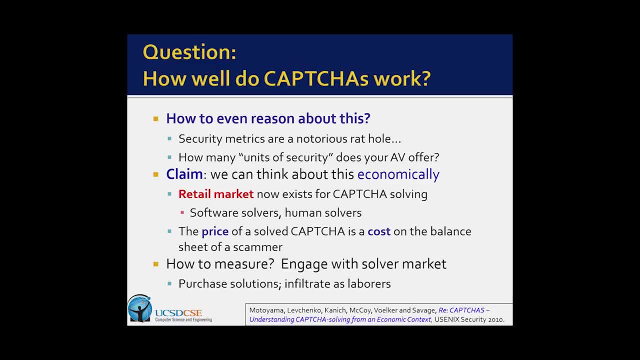 think about this from an economic standpoint. is the price to solve a CAPTCHA is a cost on the balance sheet of the attacker who is trying to artificially sign up large numbers of accounts. All right And well. how much does it cost them? One million, two. 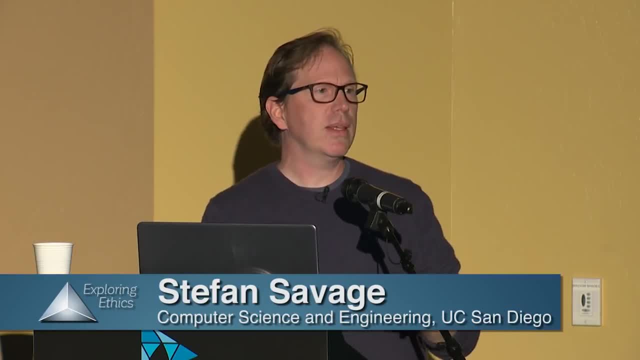 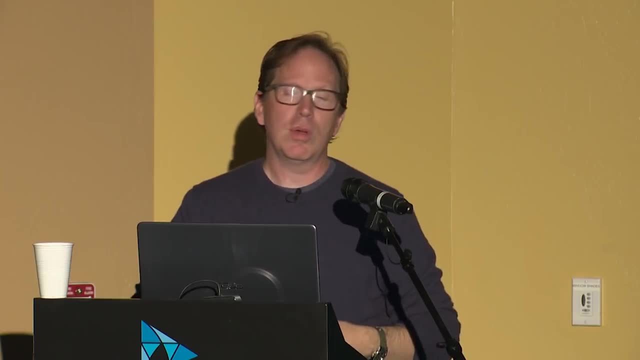 One way to do this is to engage directly with this market, And there are multiple ways, it turns out, you can engage. One is on a retail basis. You say I would like to buy solutions to CAPTCHAs and I'm going to give you a bunch and you will pay me. And there's a ton of services that will do this that are pretty sketchy, But you go there and you do this. The other is that it turns out that the way much of this works is with humans. So you have some service that wants to do mass sign up. 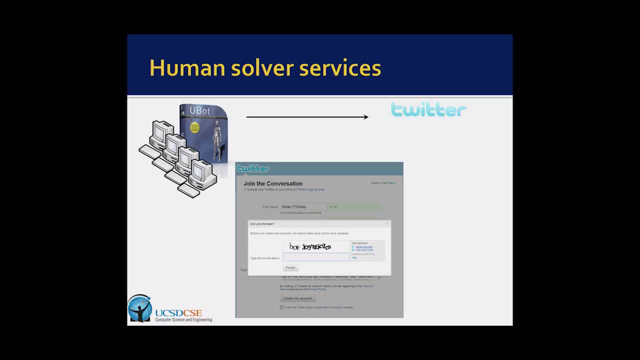 say for Twitter, and the computer software will recognize there's a CAPTCHA here, it'll grab a picture and it sends it off to some third party service. The service that I'm describing here is called DeCAPTCHA, which in turn has a partner program. 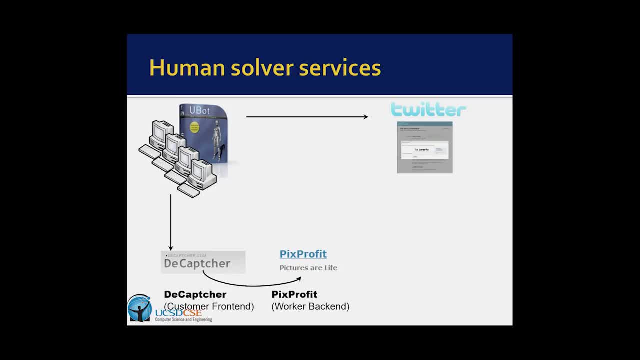 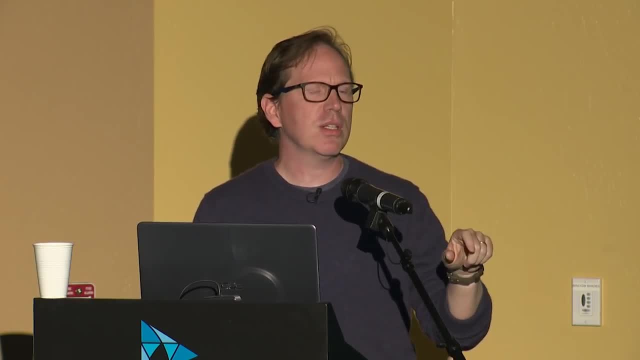 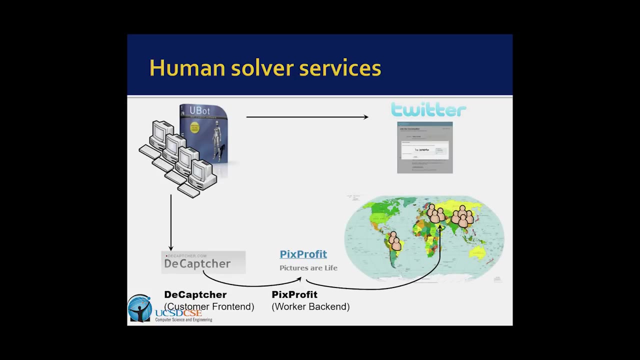 called PixProfit, that just hires extremely low cost labor, largely from China and Bangladesh, who just sit there and solve these things all day. That's all they do, And so they just sit and solve CAPTCHAs eight hours a day And it gets automatically routed to one. 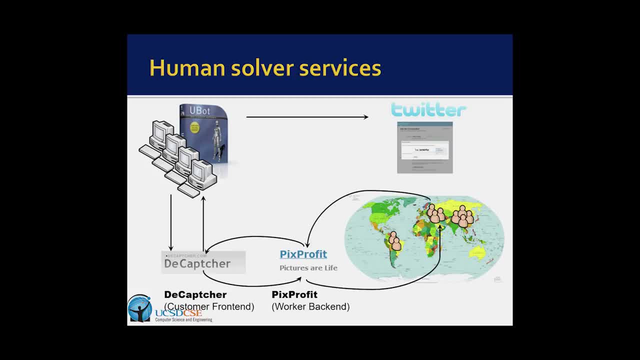 of the hundreds of workers that this particular organization has. They solve it, They send it back And then, in the course of a very short period of time- about the same time as it takes a normal human to do it- actually faster than you and I would do it. 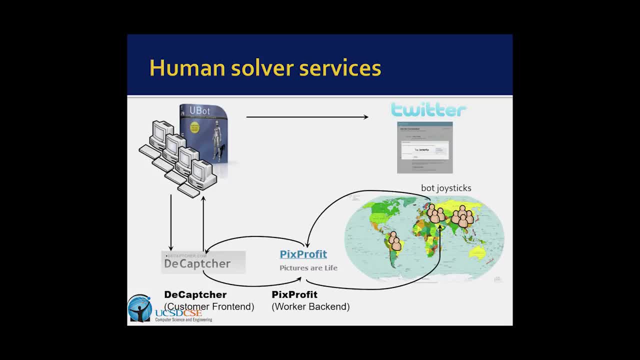 because they've been doing it all day, so they're quite good at it. you get an answer, Yeah, They get an answer back, and then this just gets plugged into a computer program, And so it's this computer program that has mechanically used human labor. 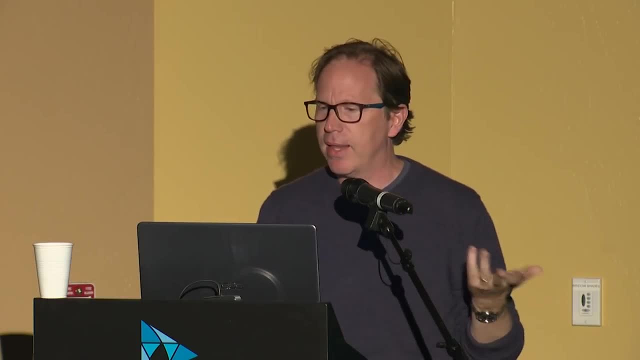 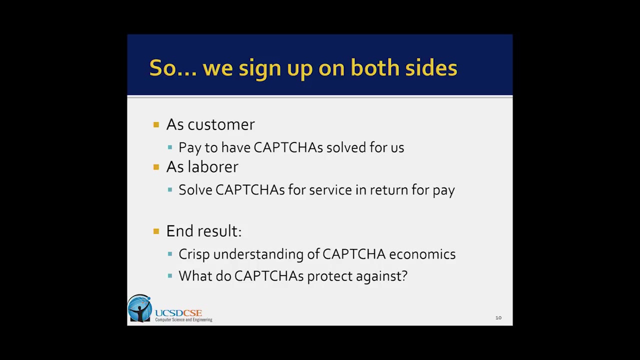 And so it just calls out every time it wants one of these solved and then puts it back in and then they can get their solutions. So we signed up on both sides for a number of these different services. One is a customer, So we paid to have CAPTCHA solved saying hey. 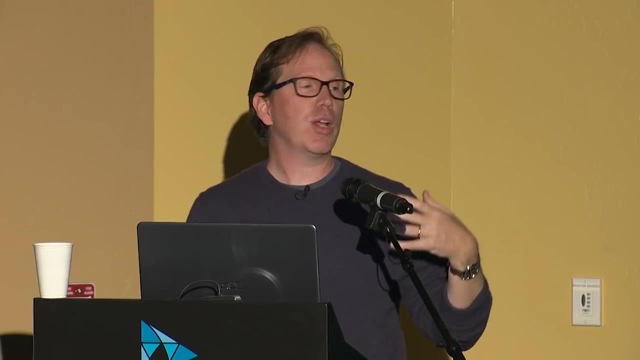 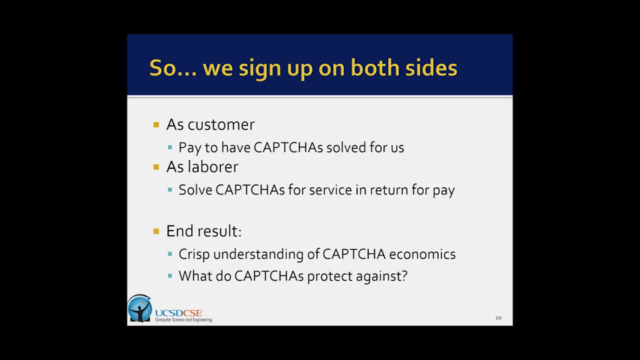 we want to solve this, And sometimes we would solve a lot to see at what point couldn't they solve any more. And on the other hand, we would sign up as a laborer and say, yeah, we're willing to solve CAPTCHAs for money. 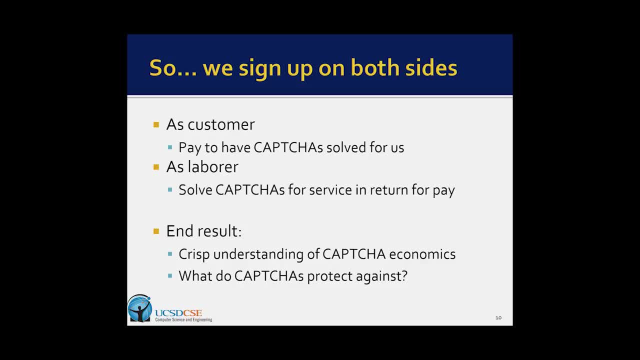 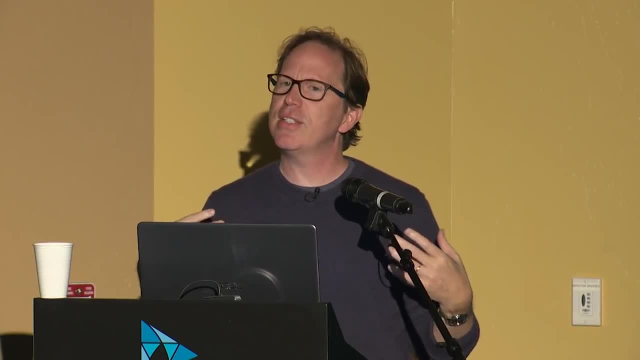 And that would let us see what kinds of CAPTCHAs did we get, and so on and so forth. In both cases we are engaging with potentially criminal activity in different contexts And there are different ways in which ethical issues come up in this one. 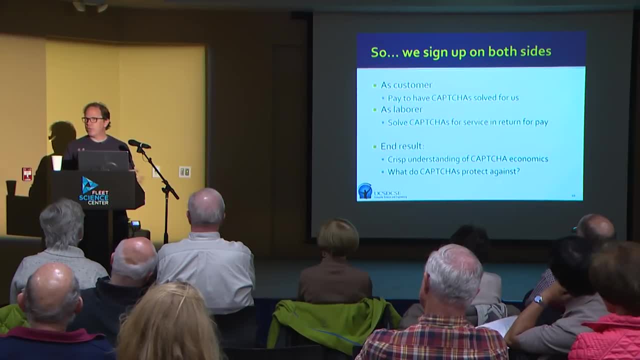 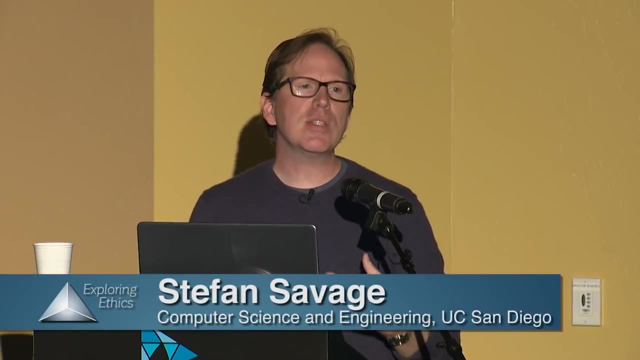 Now, and we can talk later about the ways that we try to address these issues. One of the benefits that came out of this, though, is that we were able to say very crisply: all right, here's the cost structure of CAPTCHA solving. 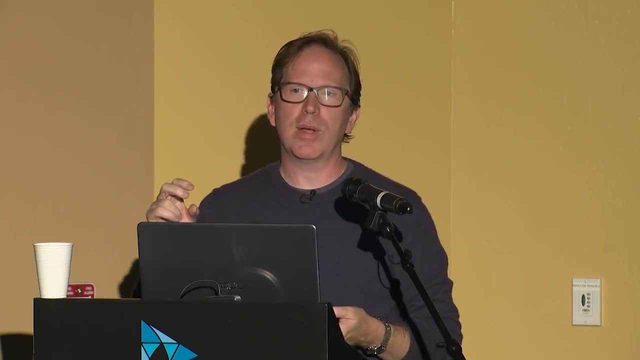 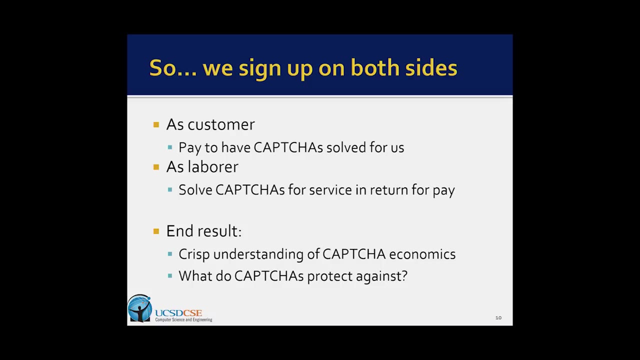 Here's where it's not going to go below, because this represents basically what the prevailing minimum wage in low wage countries that have internet access is going to be, And it changed the way that places like Google and Yahoo and so forth think about this- that this is not a defense. 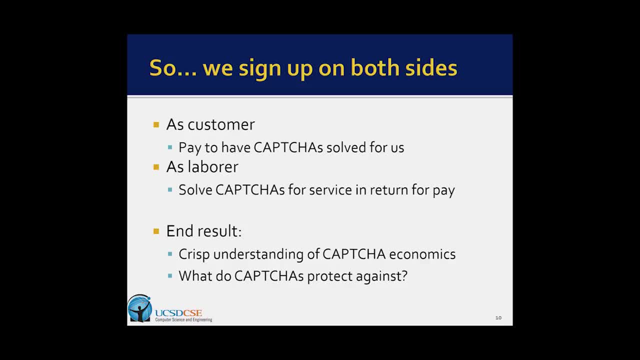 It is a filter. It ensures that the people who are abusing your service need a business model. That's not a defense. It's a filter. It ensures that the people who are abusing your service need a business model. That's not a defense. 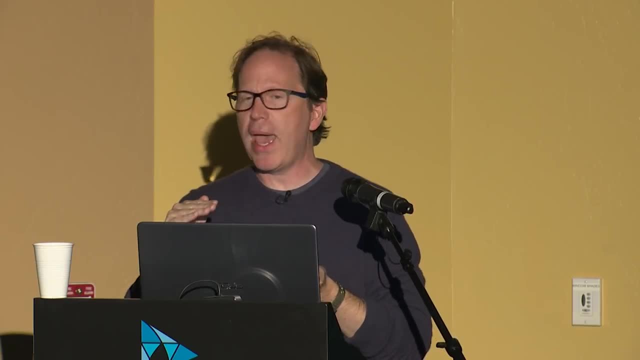 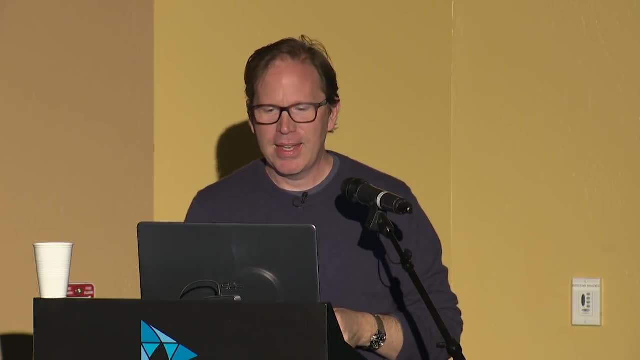 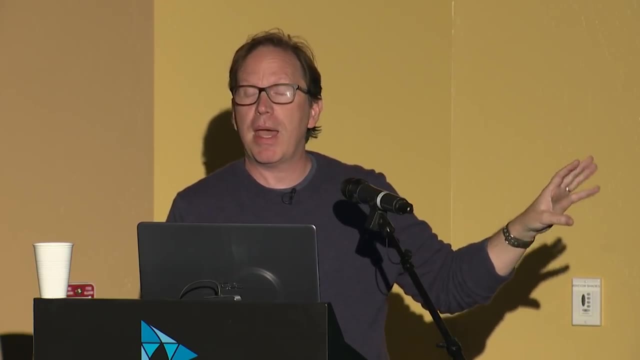 And you've got to feel for these people who are solving them All right. So that's one, And I'll just let you think about some of the challenges. So this is actually quite valuable for the companies to then think about. It also helps them figure out when 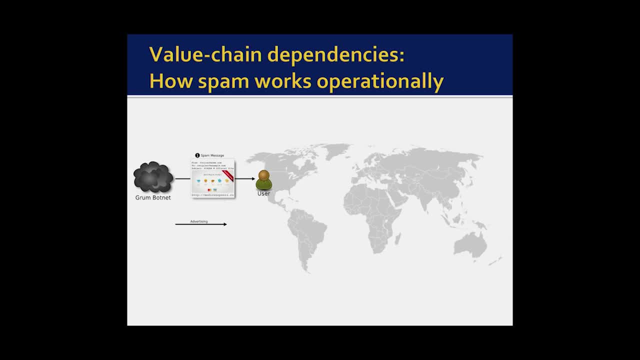 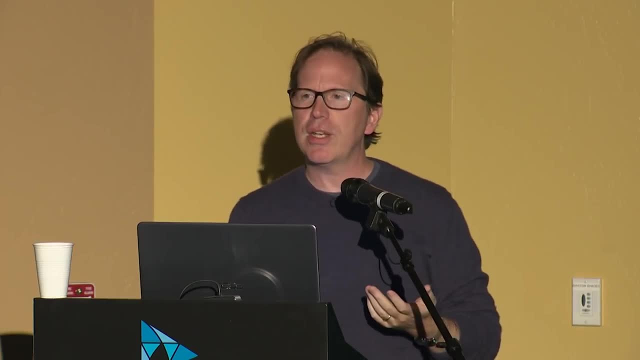 they have to change their CAPTCHAs, and so on and so forth. All right, So I'm going to shift to a related project, which was looking at the spam ecosystem, which is actually quite complex, And so this is an animation of what 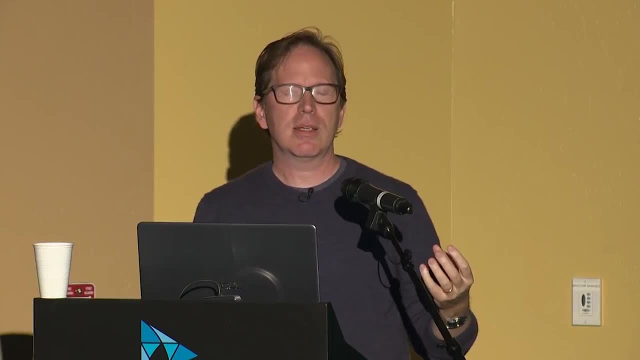 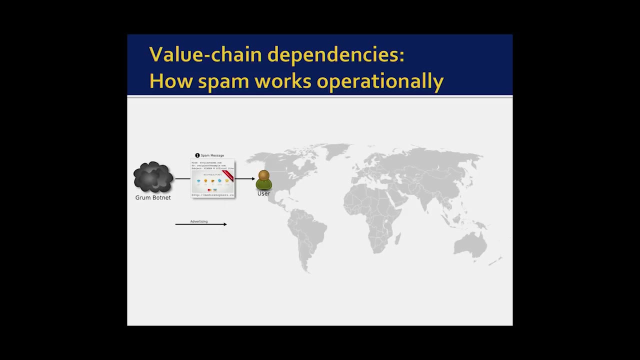 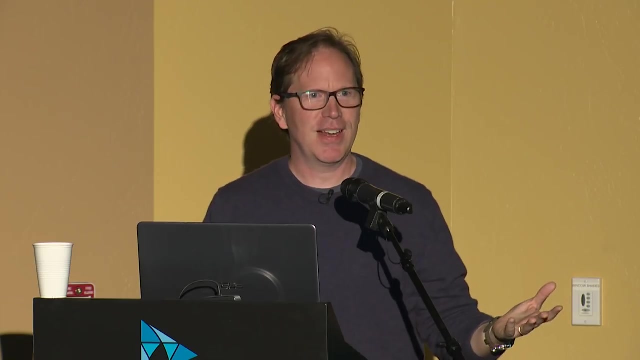 goes on every time a spam message is sent in order for it to make the sender money- Because we tend to focus just on it arriving. But for them to make money on it, one of you all has to click and buy the stuff, And that's the bottom line. 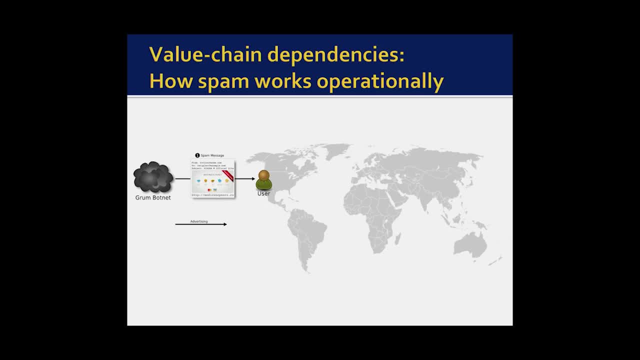 Otherwise they wouldn't send it, And so it comes in and then someone has to click And a lot of things need to happen at this point. So in this case there's a domain name It says: click on whatever. this is medshoprxru. 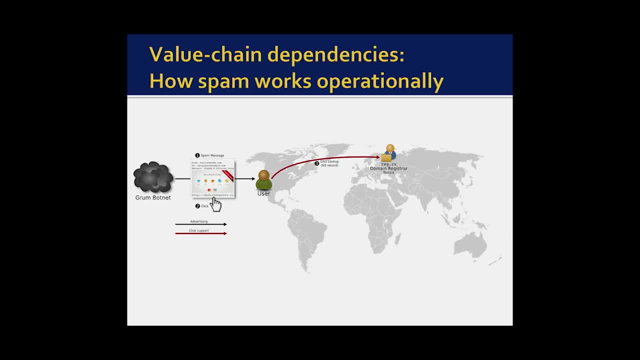 There's what's called a domain registrar that you have to buy that domain name from. This one was in Russia, And then there has to be a thing called a name server to say how do you find that server? This one was located in China. 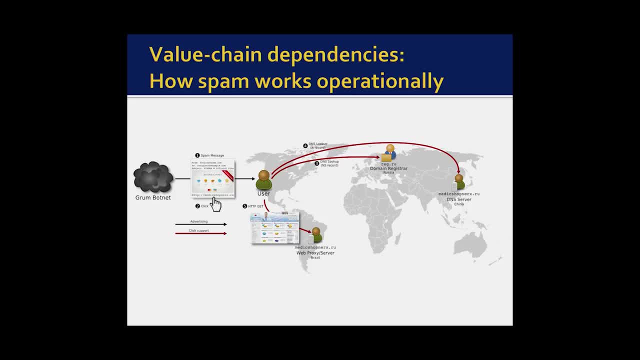 This is an actual example of a particular message. Then it has to get content. This was actually from a proxy server in Brazil. Then actually, if you want to make the sale, it reaches back to this criminal enterprise called an affiliate program in Russia. 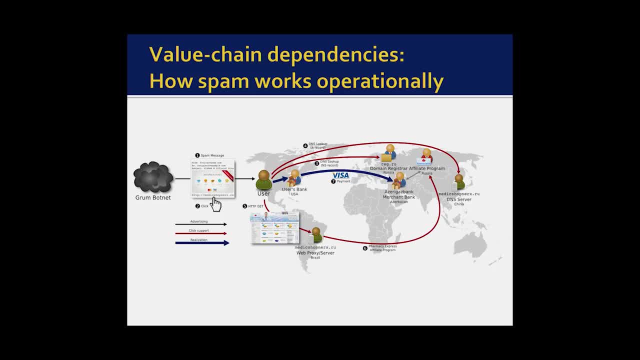 that had contracts with an Azerbaijani bank that could accept visa and then arranged to do drop shipping out of India back to you to get your Viagra in this particular case, And so all of these things need to work. This is a complicated business and these 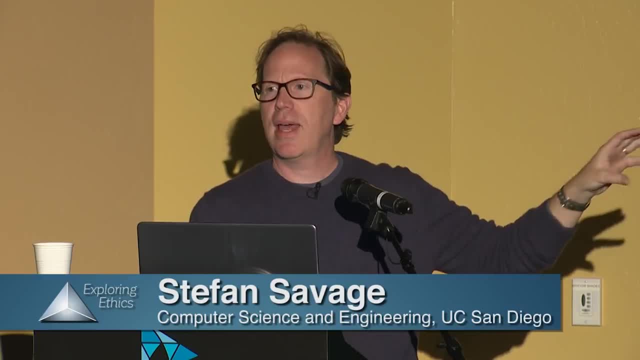 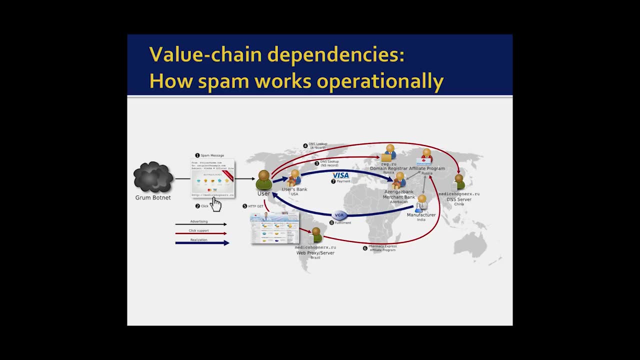 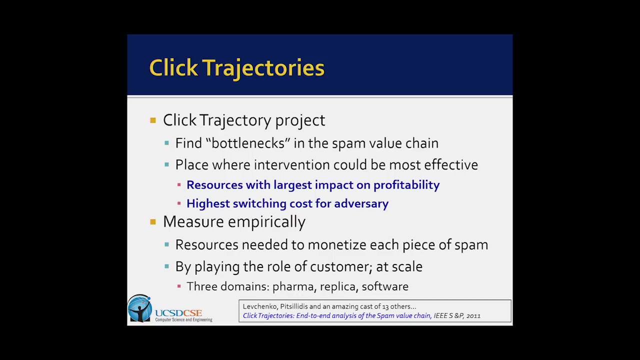 are all separate entities that in some sense are knowing or unknowingly involved in a conspiracy to put together this business. So we asked ourselves: rather than think about this entirely in terms of how do I filter this stuff out, could we think about it in terms of what is it? 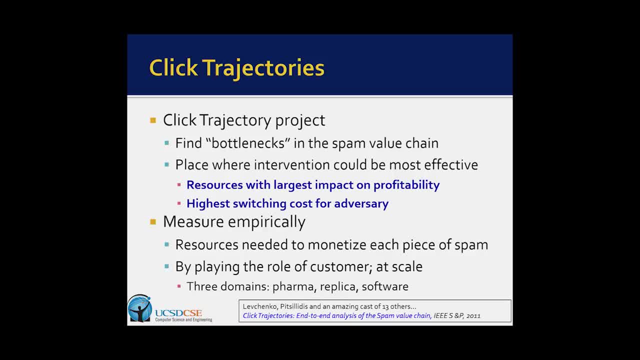 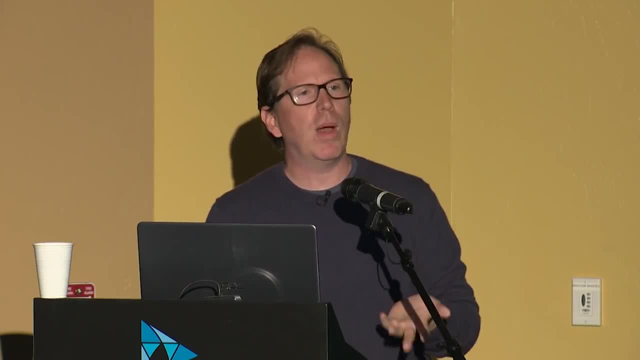 that makes spam profitable. There are all these different in that graph. I showed you any one of those edges. if you got rid of them, that message could not be monetized, And so then you might say: well, which edges? 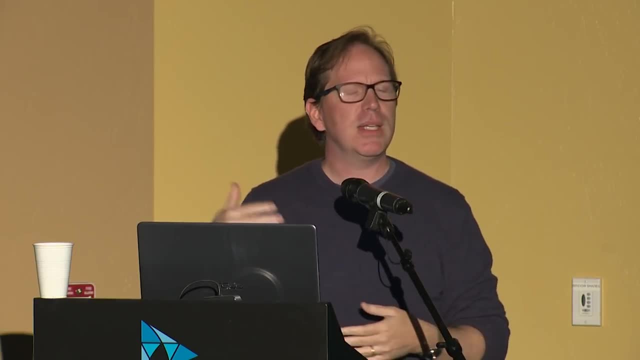 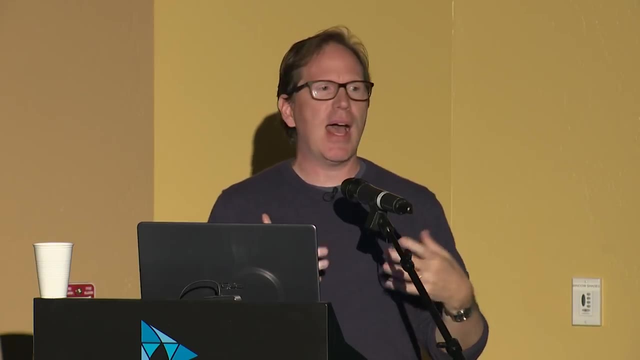 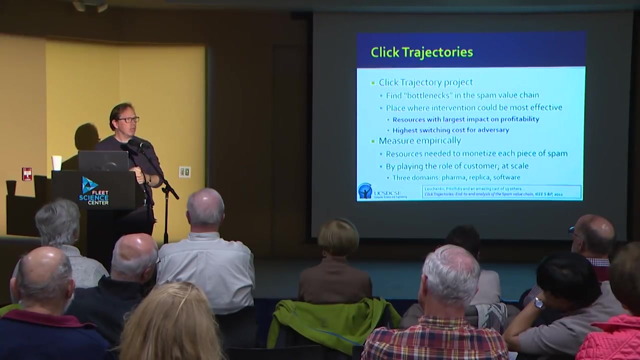 are the most valuable edges. What does it mean to be most valuable? It means that it's cost effective to get rid of it and that the replacement cost for the bad guy is high for them to find an alternative. And so we did this by building the world's most naive user. 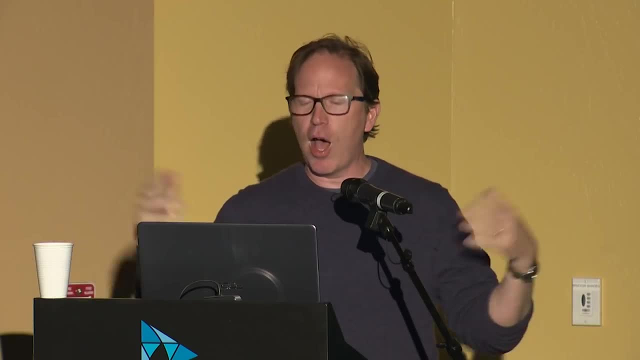 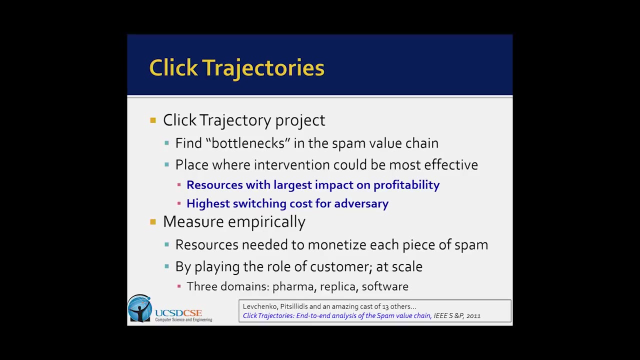 which was a stack of 40 servers that all day long took all the spam of all these big companies that they gave us and clicked on every single one, and then it would visit the sites, And then we created a system that could automatically categorize which ones belong to which criminal program. 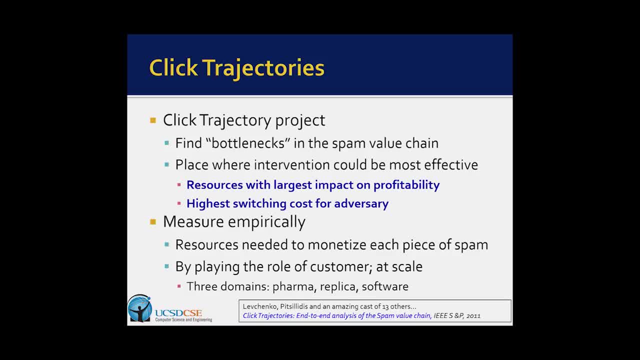 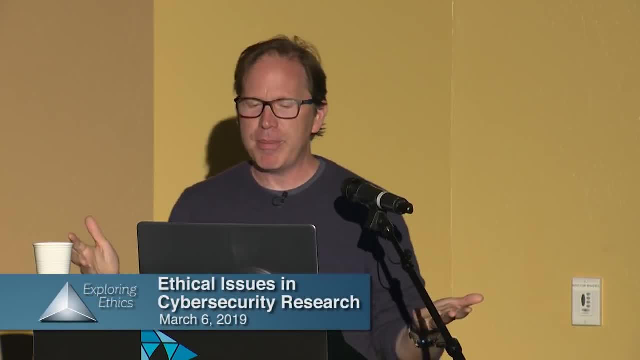 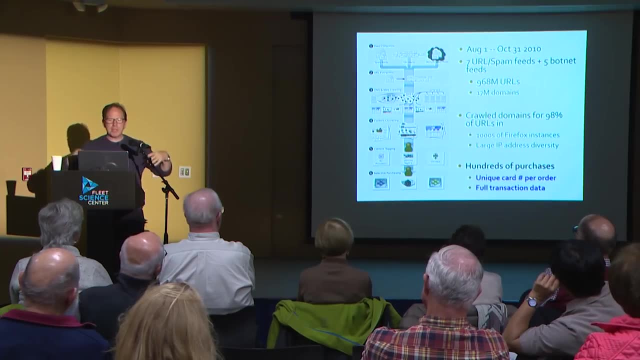 We also had a student- and this is where one of the ethical issues comes in- who joined two dozen criminal programs pretending to be that they wanted to be a spammer, And then we purchased from all of these criminal organizations And so we had this big thing that. 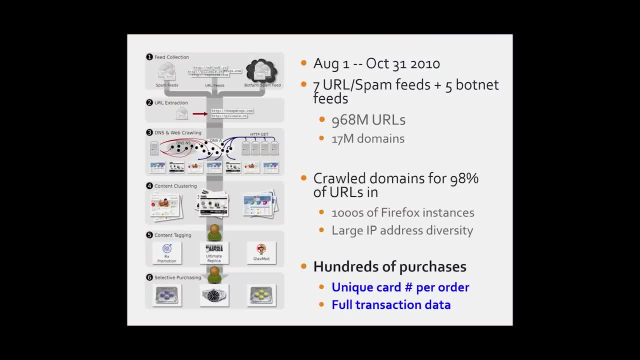 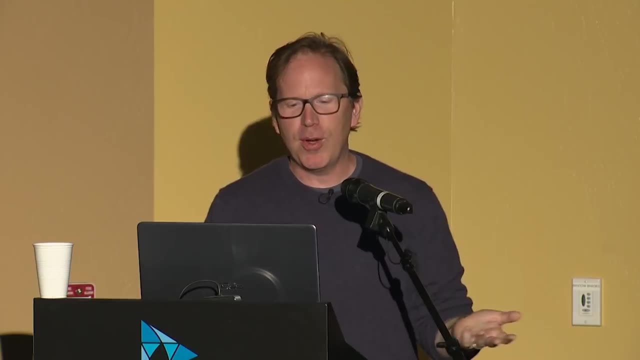 would crawl everything and then buy stuff from all these spam-advertised goods. And we had a special deal with a bank that then allowed us to track the flow of money to figure out when we bought something, where did that money go. So it was rather unusual for a computer science effort. 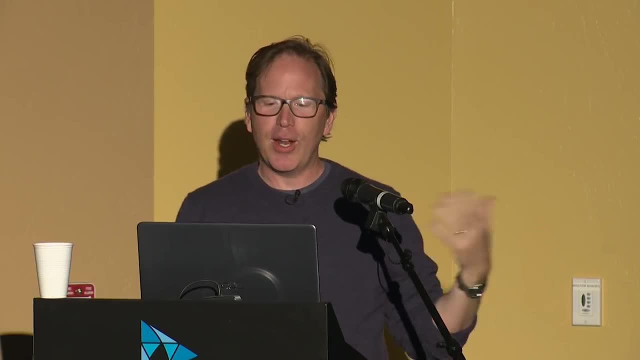 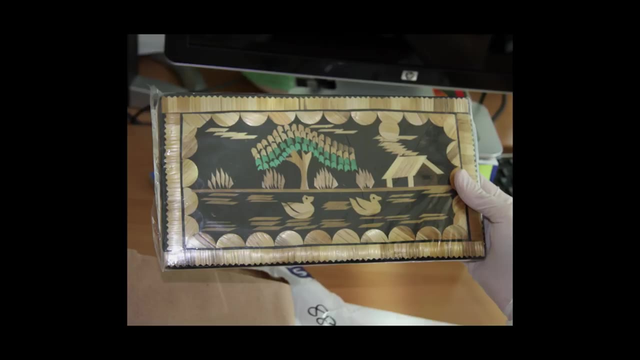 So we had all these people, grad students, who would get these things in the mail. They would have pharmaceuticals or counterfeit Rolex watches, Or occasionally we would get this textile, That then you would kind of notice that one part was a little lumpier. 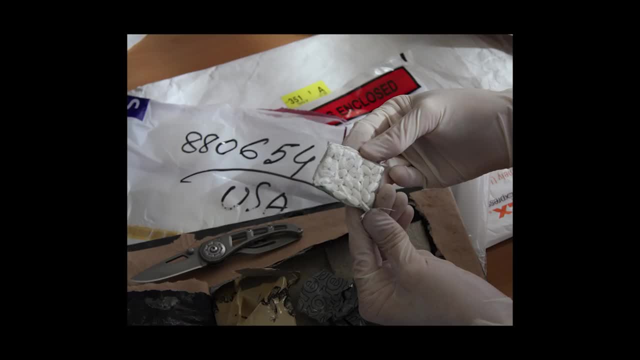 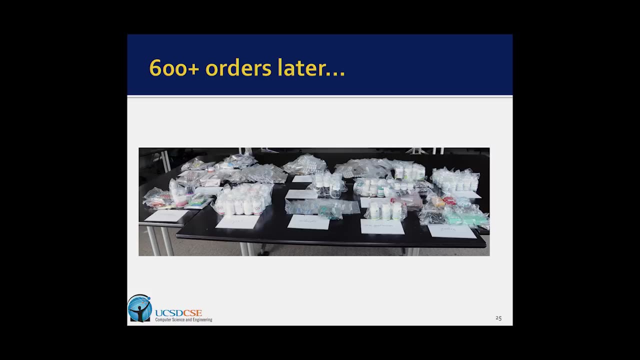 And you'd find out that that's where the drugs were secretly hidden so that it could get out of Pakistan. And so we are unique in computer science in having a drug room. But the result is that we were able to go through and look at all of the different resources. So literally for like a billion spam messages, every resource that was required to make one of those monetizable And see what's the replacement cost if it were gotten rid of. And the sad news was that most of them have very low replacement costs. 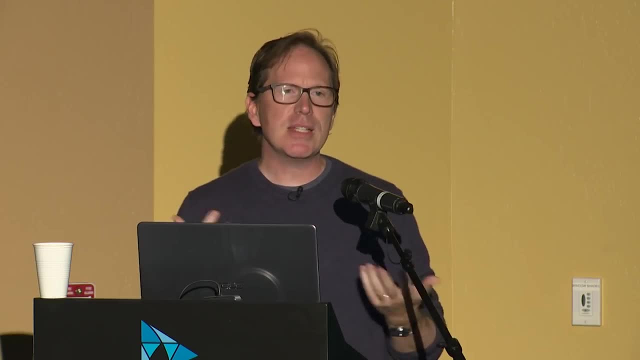 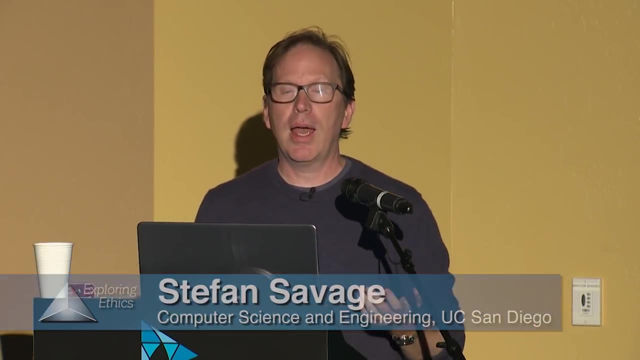 And this is why if you shut down a cyber crime server, it doesn't matter, Or you take down a domain because they can get another one for $3 in five minutes. And the exception was banks. So the banks who could accept Visa were few and far between. 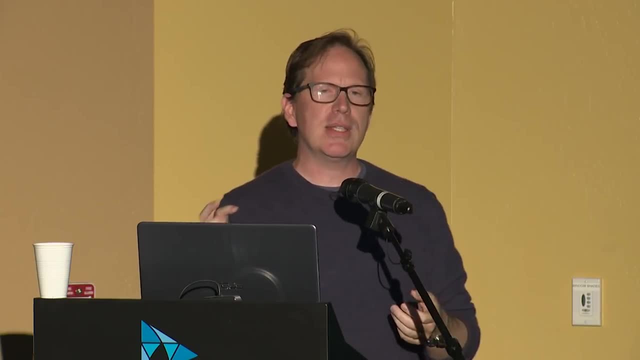 And there was a variety of financial incentive mechanisms, in particular something called holdback, Holdback forfeiture- that I can go into in more detail if people are interested. that meant that when they lost one of these accounts, that for the kinds of cash flow we were dealing with. 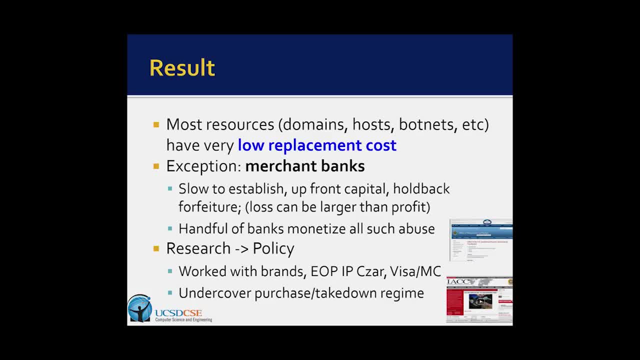 they could be out $3 or $4 million. So it was a significant loss, And so we then spent a bunch of time working with Visa and MasterCard and the White House and some brand holders to put together a program to do this. The first example was with Microsoft. 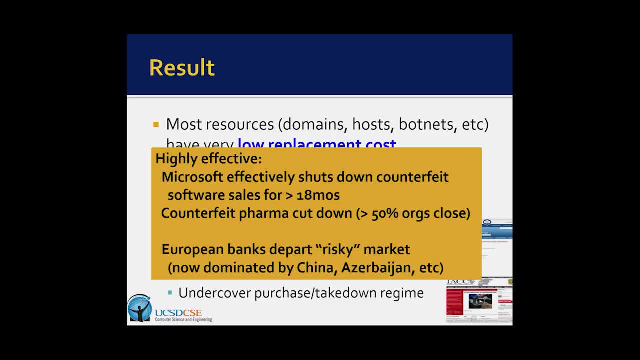 And we effectively shut down the sale of counterfeit Microsoft software anywhere in the world for 18 months. It could not be done. And then we did some similar stuff with pharmaceuticals, maybe not quite as effectively, But here's kind of a qualitative example. 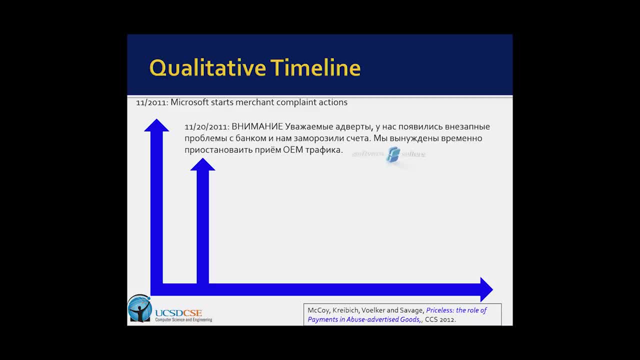 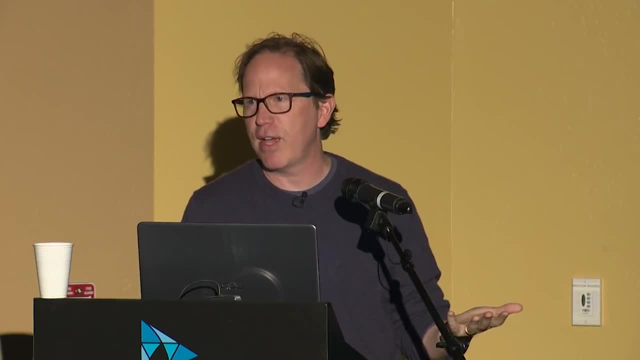 We started this in November 2011.. And, as I said, we had a student who had joined a bunch of. this is a set of criminal organizations that sold counterfeit Microsoft software, And so we had a student who had joined these organizations, pretending that they, too, wanted to be involved in the sale. 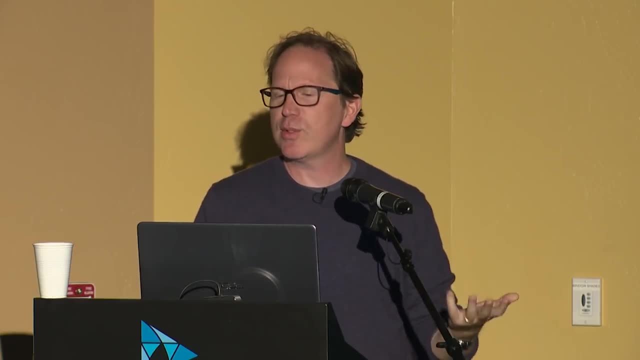 And so they would get notifications from the boss, as it were, saying here's what's going on, And so you can think of this as like the battle damage assessment of cyber crime fighting. And so, of course, it was in Russian. 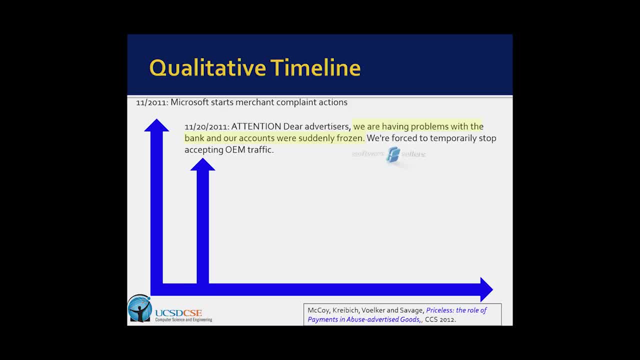 because all these guys were Russian, And so this is what it translates to in English: We're having problems with our bank. Our accounts are frozen. We're temporarily forced to stop selling this stuff. Another one said our bank has stopped working. 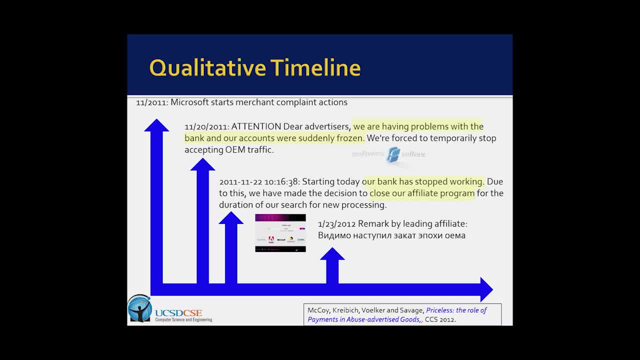 We have to close. And then my favorite, because it's very Russian and very poetic, was this one, which I can't read in the native Russian, but it's: the sun is setting on the OEA, Oh yeah, On the OEA. 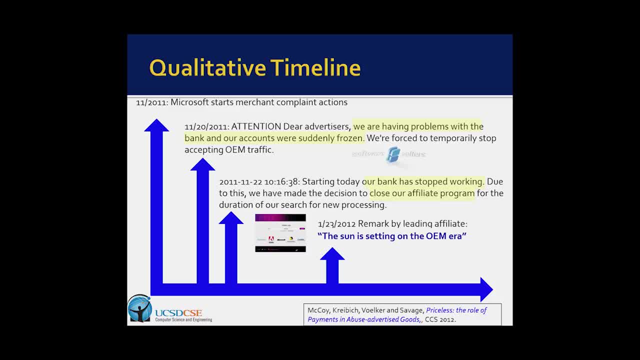 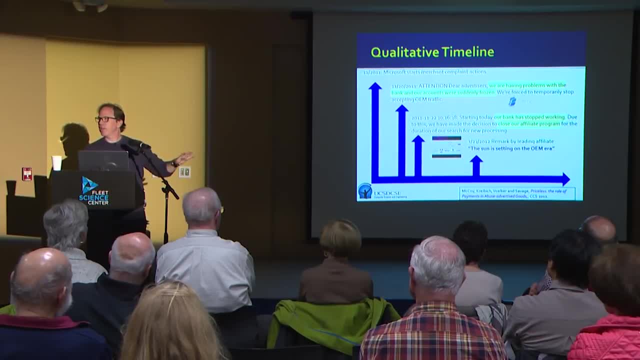 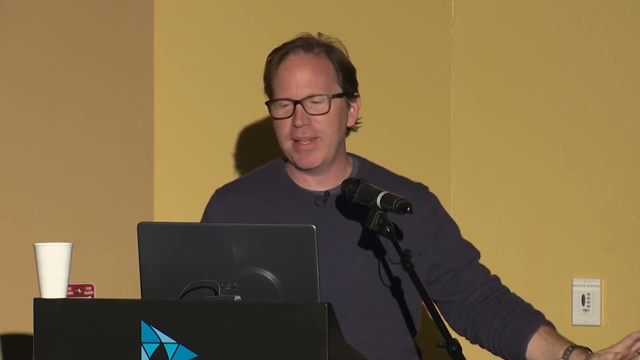 All right. So there were a ton of ethical issues here involved in large-scale interaction with criminals, with joining criminal organizations, a bunch of others. I can tell you that everything that we did that involved an IRB, had an IRB and our general counsel. 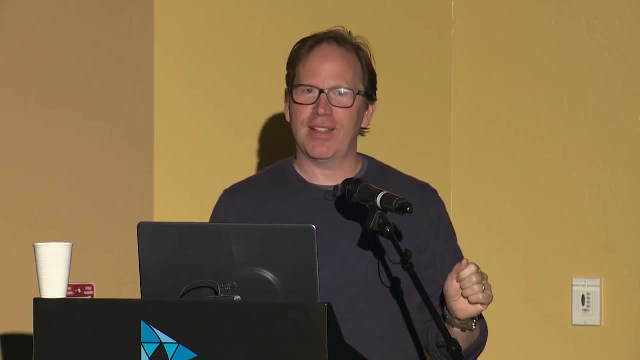 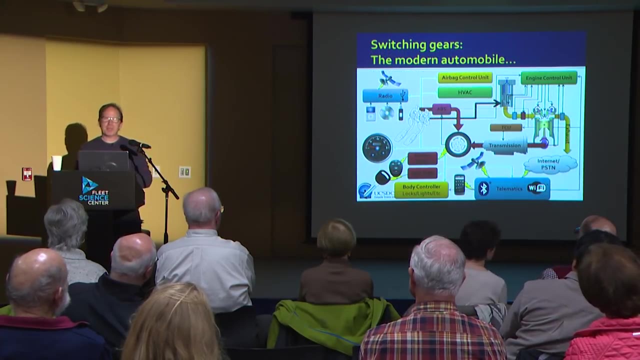 was involved with everything, But it was non-trivial thinking through these things. These were not something you just go and do. And then the last one: I'm going to put up. very different work that we did for some time focused on automobiles. 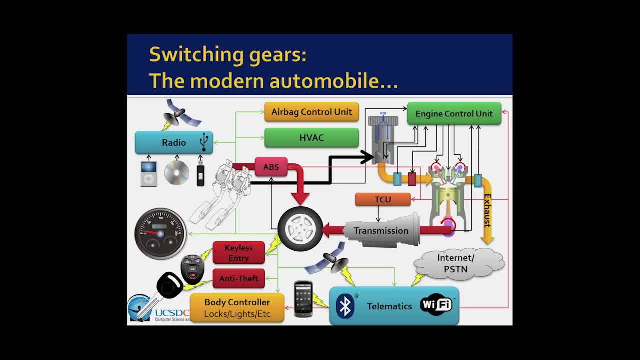 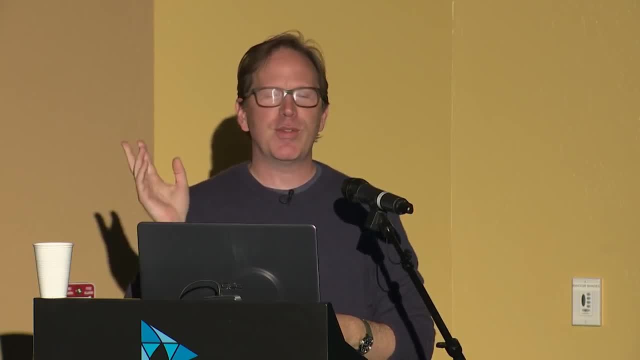 And the way I learned about an automobile. my mental model is the Henry Ford model. There's this mechanical thing where there's hydraulics and gears and something like that, And that has been true for a while. So they're all computers that are between you and anything. 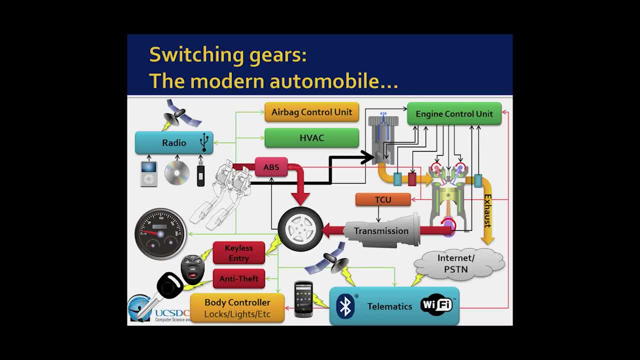 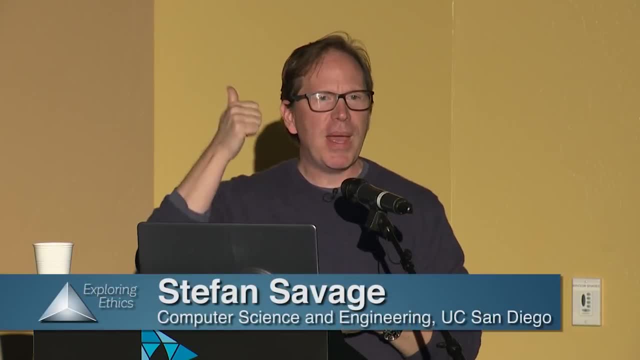 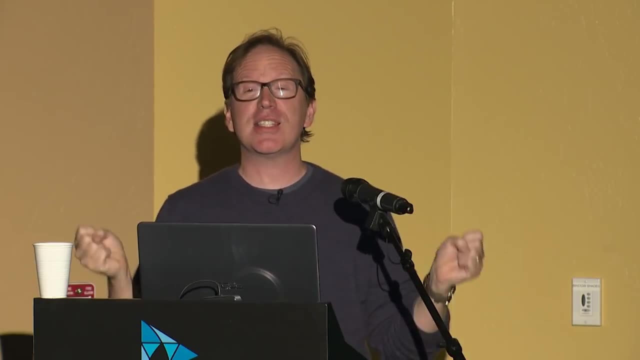 And a computer reads that and says: you know, the meat bag up top wants to go faster. Please go and change the fuel and oxygen mixture to make us go faster, Because there's a ton of variables that they're doing And a lot of this is for good reason. 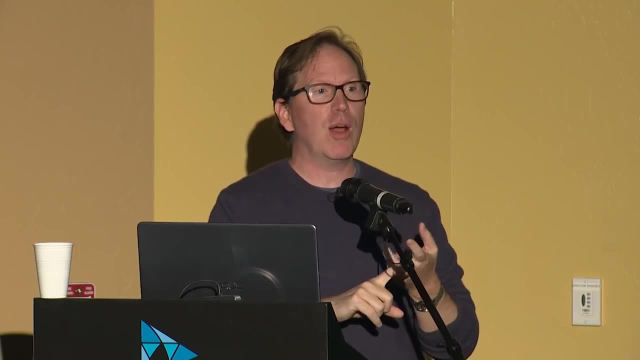 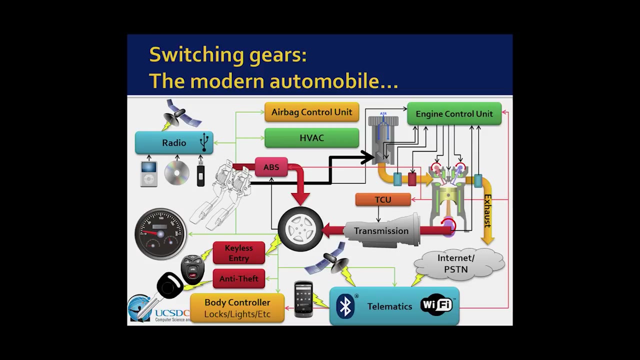 It makes cars more fuel efficient. It makes them more safe. Anti-lock brakes could not work if a computer was not in the way. Stability control is the same way, But it turns out that as this has grown, we've got tons of these computers. 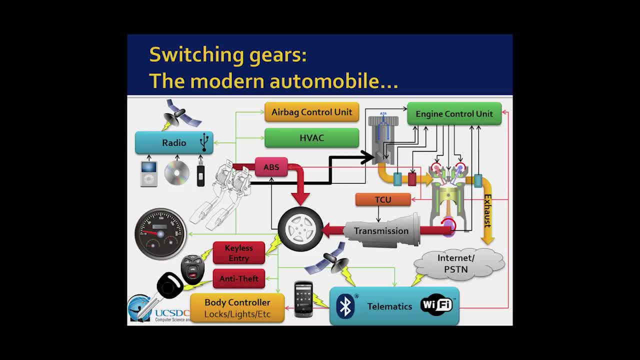 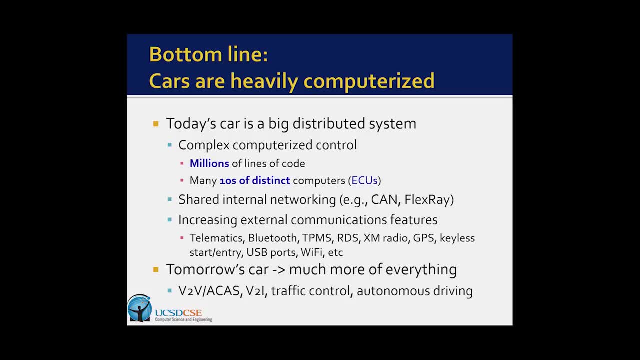 that control everything in your car. They're all networked together And increasingly they're externally networked, And so today, a car is just like the most complicated distributed system that you personally own. There's nothing in your life that is close to it. 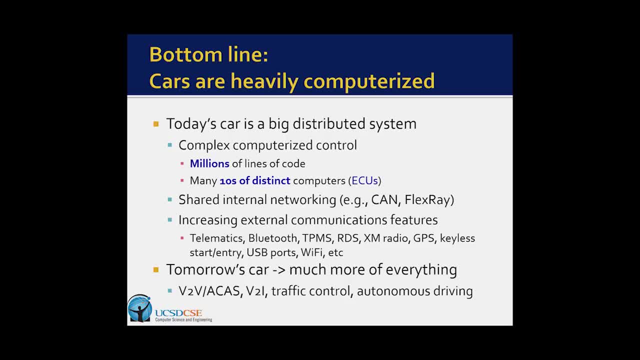 Their ballpark are going to be 30 or 40 different computers in your car that will have millions of lines of code that are talking to each other over all of these different networks and are connected to the external world in ways that you may not recognize. 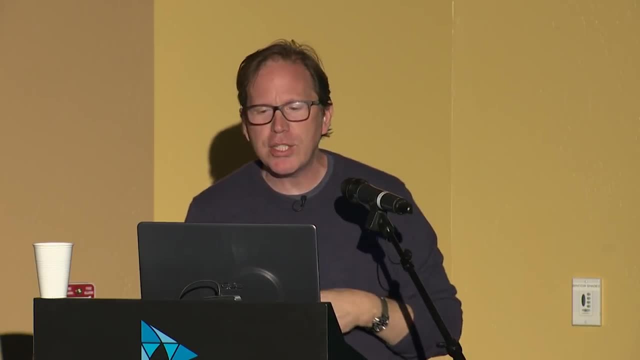 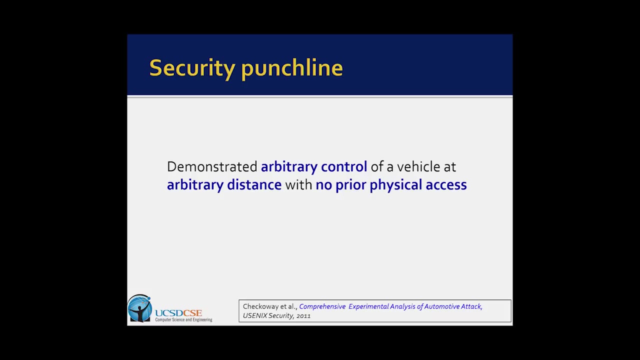 And so we did some work, This joint work with the University of Washington, showing that, for very large numbers of cars that we were able to sight unseen, just take them over. And so here's the punch line, which is from a 60 Minutes piece that highlighted some of our 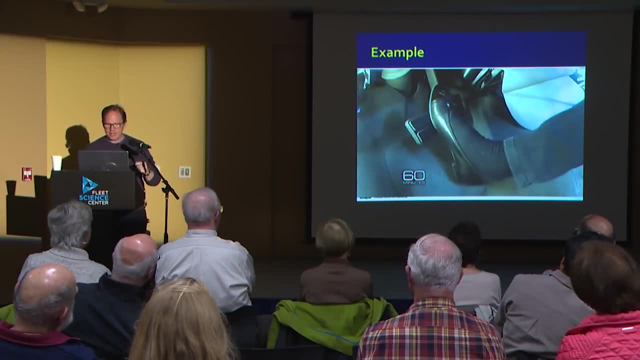 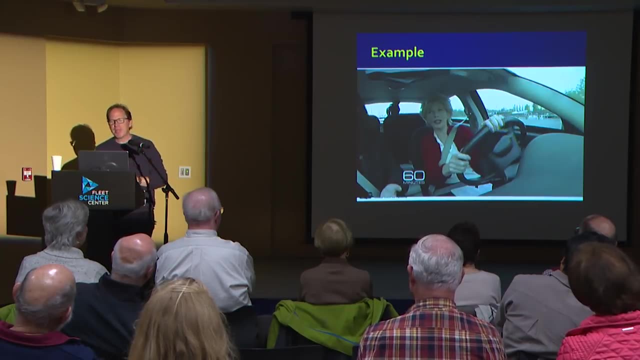 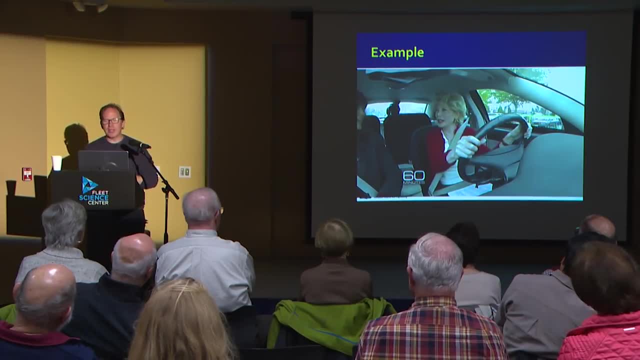 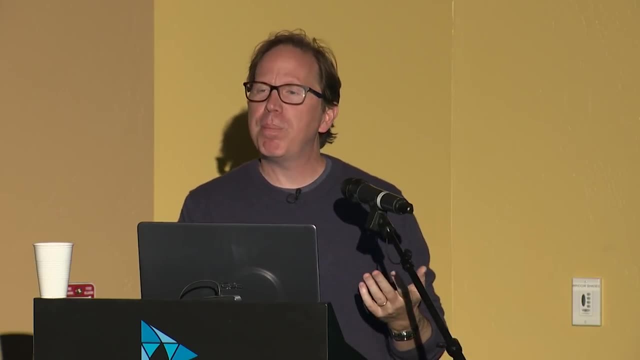 And the part that's not shown here is when we had a little, A little glitch and couldn't get her brakes back on, But she survived. We've seen her in future shows And so this had a lot of So we did this work and we did disclosure. 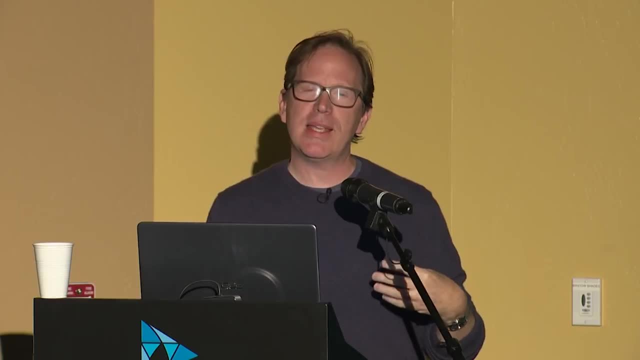 And that's where a lot of our ethical issues came down to- is: what can we safely say, Because we were in a position at multiple times where we were actually able. There were probably 7 million cars on the road that we could take over. 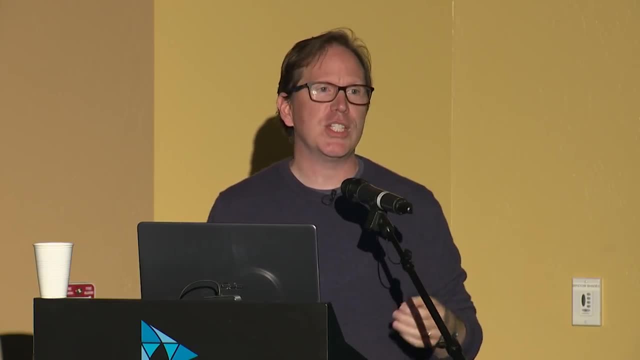 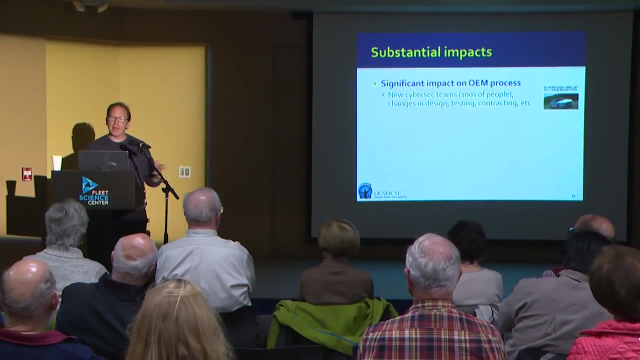 And the federal government didn't know what to do And the manufacturer at the time, which was GM, was really not sure what to do And we had to be very careful about how we talked about our work Long term. there have been a lot of positive impacts. 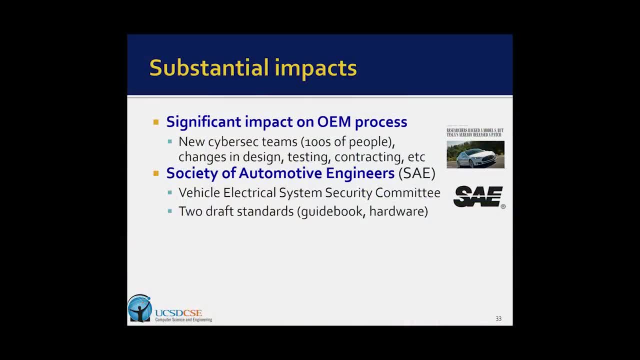 Literally hundreds of people hired into the different OEMs. There's a new standards process. The National Highway and Traffic Safety Administration has a test lab. There's many tens of millions of dollars in research. Cars are much more secure today as a result. 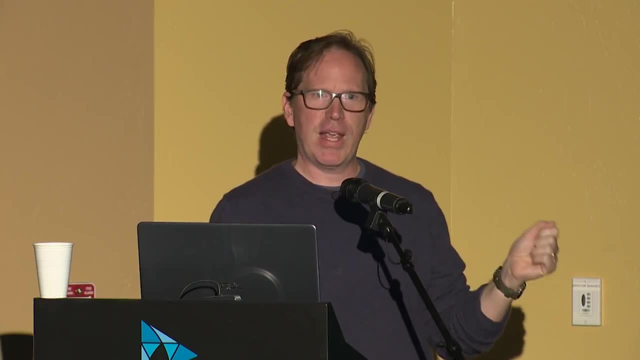 But it was a very tricky business figuring out what we could say and when and to whom and how, And also negotiating to make sure that we weren't going to be sued, which was GM, it turns out- had two board meetings to decide not to sue. 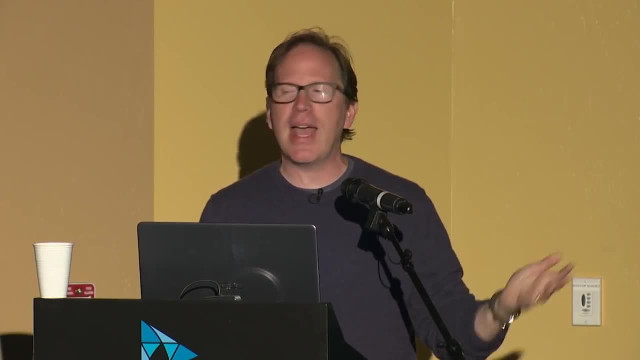 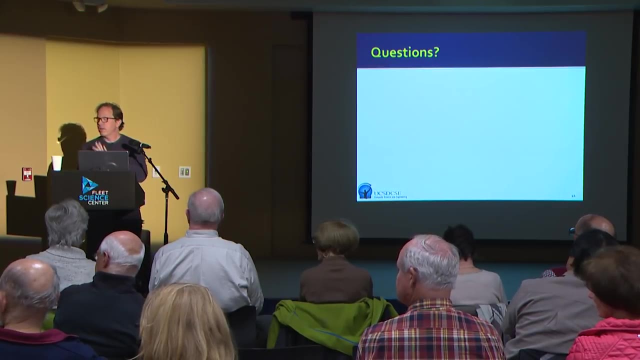 the University of California, Anyway. so that's kind of a summary of the kinds of things that I've been doing that have brought up these ethical issues And I don't know. We're going to do a break now. We'll take a brief break. 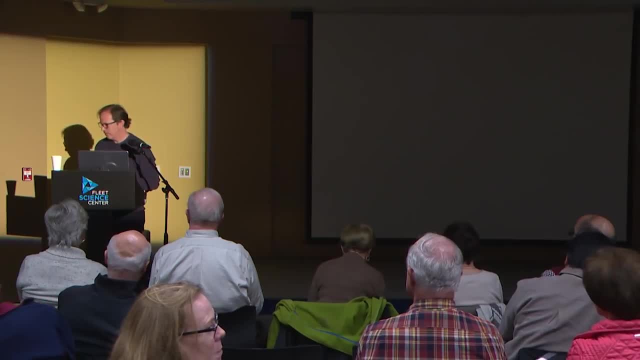 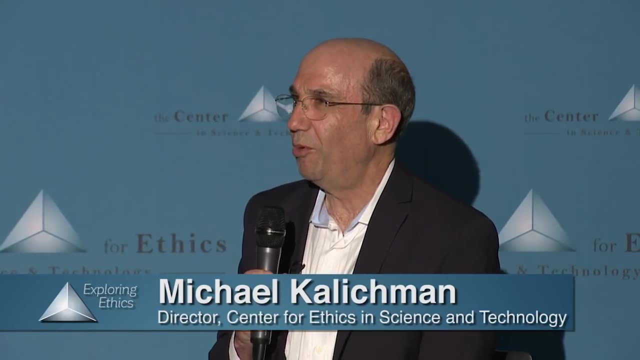 Quick break now and you guys can think about questions you have and we will get back. Before we get to some of your questions, I have a couple that came to mind. One came to mind because of my experience teaching research ethics to researchers. 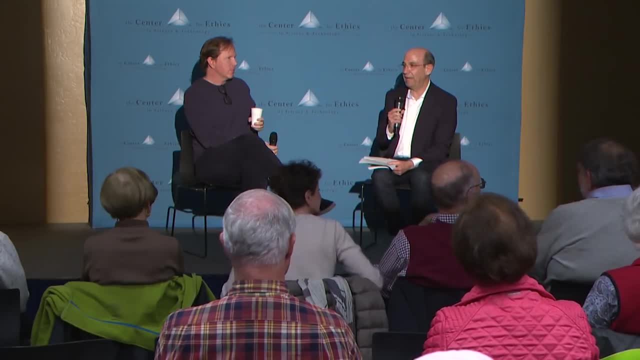 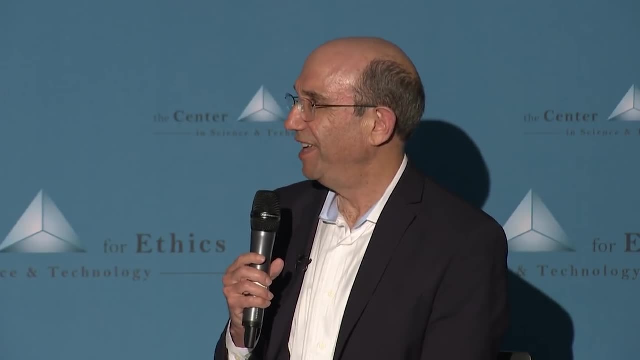 and the problem of talking to them, for example, about manipulating images, and talking to them about how one can do that and get away with it. And so what you're doing: while you're telling people about a problem that's out there, you're also telling them how to do it. 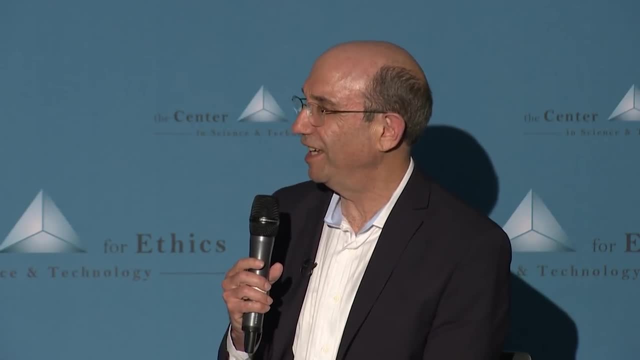 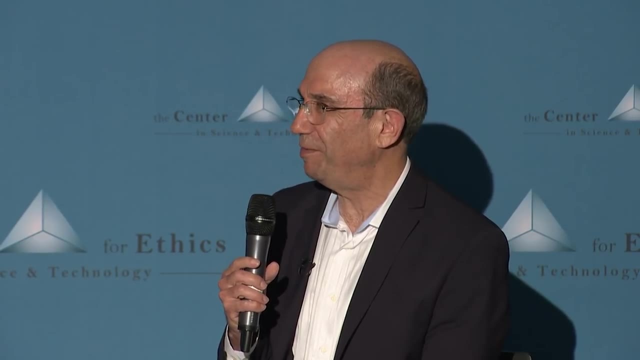 So do you ever worry that you're getting up in a talk like this one and saying: here there are services you can find that will do, that will cover CAPTCHA and be able to for pennies, you can use them. Do you feel like you're spreading information more? 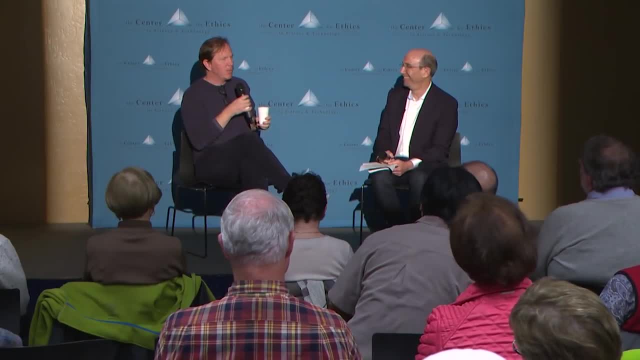 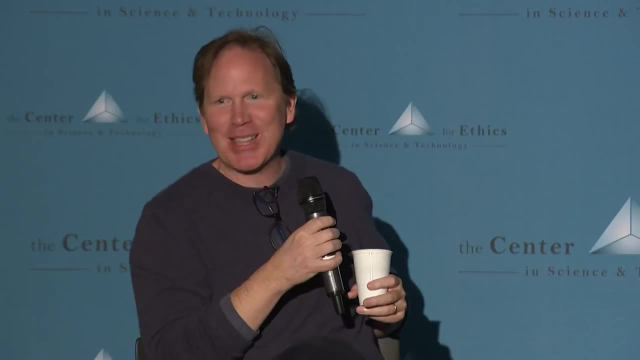 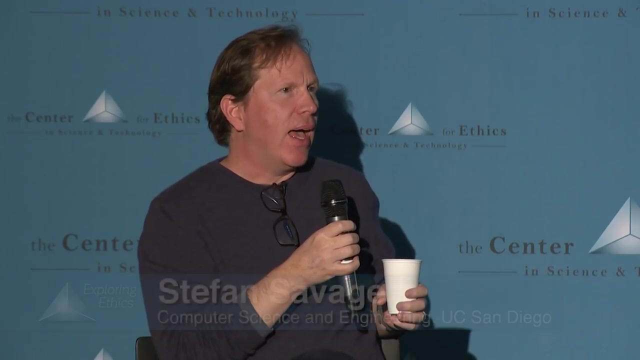 widely about how to do bad stuff. So the premise being that someone in the audience is a latent criminal and but for my talk they would have led a straight life. but now I would say that I do not have that much concern because- and 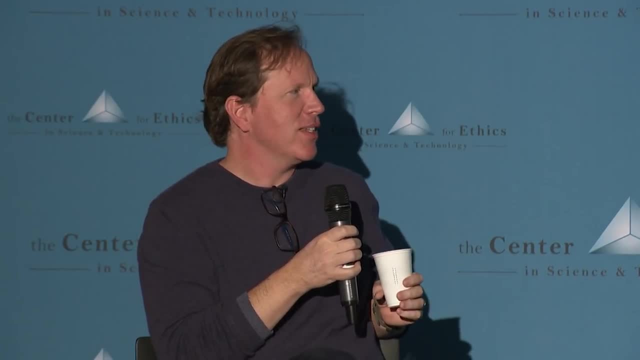 and I'm sure that the public will not have that much concern, But I will say that I do have a little bit of concern because I think that the fact that you're talking about this thing in an afternoon with Google will disabuse you of the notion that this stuff is at all. 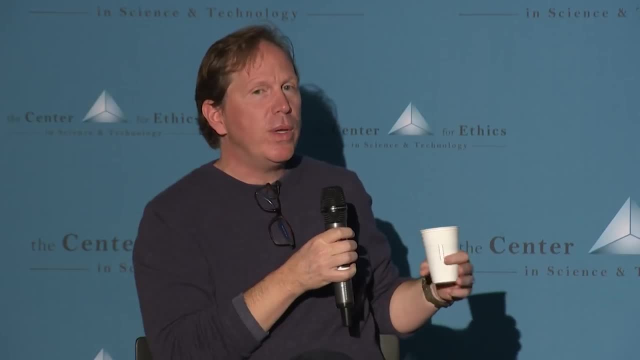 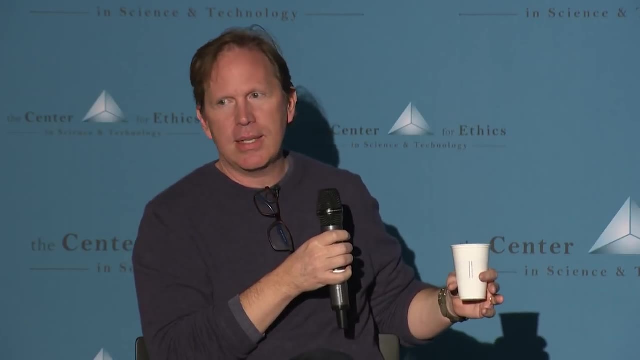 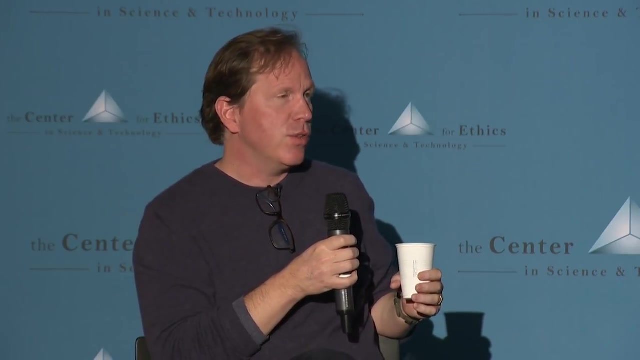 secret. However, there is an aspect of this that at times does give us pause. So, for example, we did a fairly comprehensive evaluation of these CAPTCHA-solving services and characterizing their latency and correctness and how many of these services were in place and how much data we could. 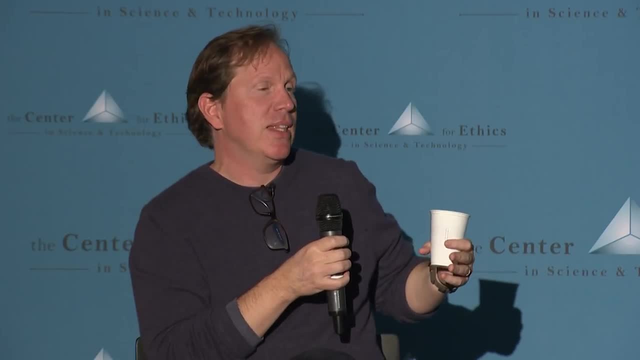 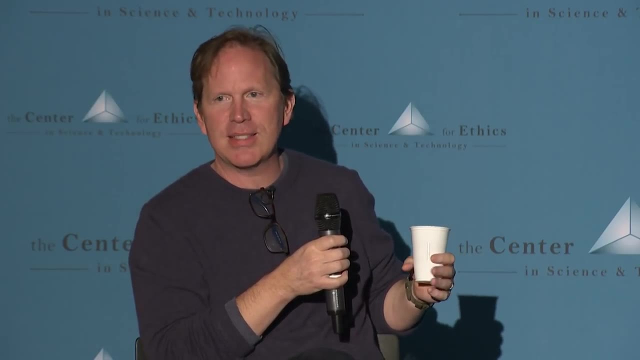 collect, how much data we could increase, how many of these services we could send to the founders- which was bizarre, You would just send these. we sent these random questions because we managed to—there was a bunch of technical stuff to figure out who actually ran these things, because they tend 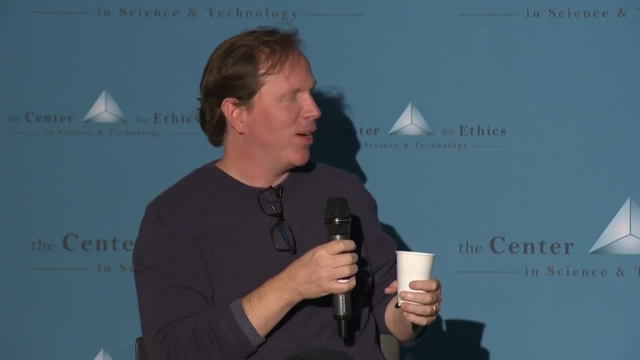 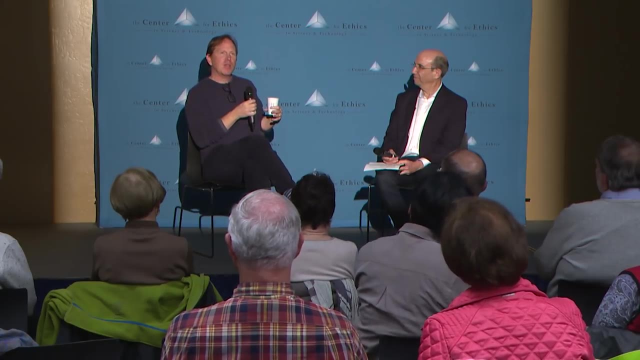 to not announce that, But they made some mistakes and we found them. Sight Unseen would send to you know some Chinese gentleman. hey, we're writing research. Would you answer this query? In the end, one of the things that I think made me a little uncomfortable is that we found again 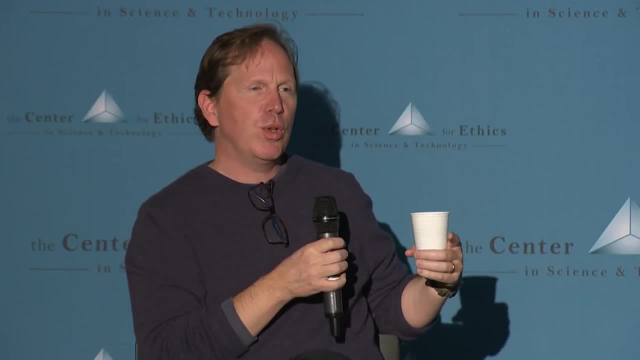 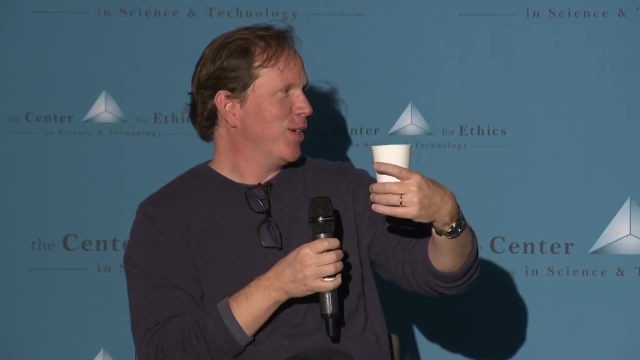 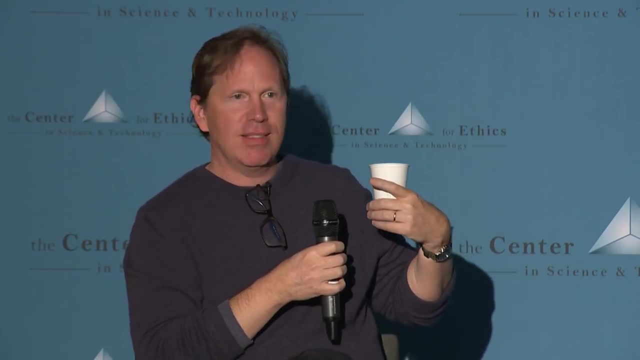 that in the criminal underground people would use our paper as a consumer reports and they would say: well, look there, their paper says this is the most cost-effective one to use and people would advertise their service saying: you know, if you don't believe us, you know. University of California says that our 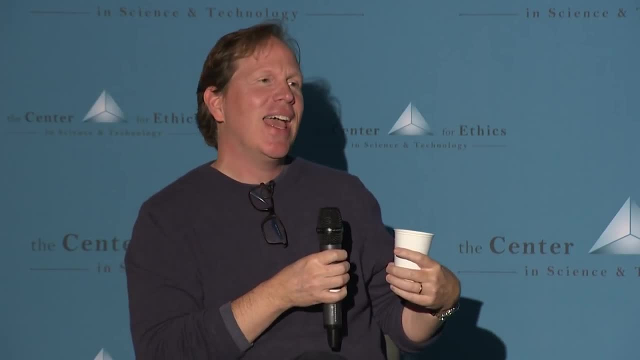 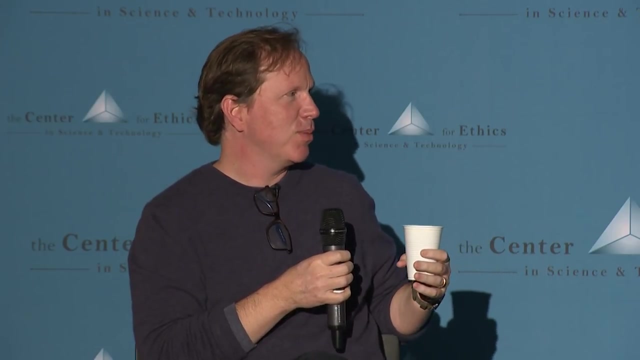 service is the most effective one and- and that was certainly not not our intent- I think the capture-solving is- is you know, in this, in the spectrum of white to black, is the beigest of the things we are dealing with. I mean, there are some legitimate uses for capture-solving, like for the blind. now I 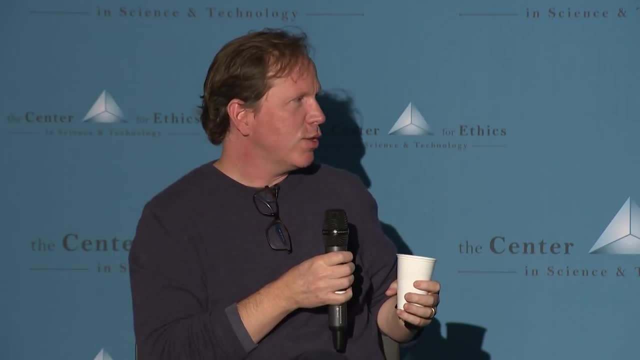 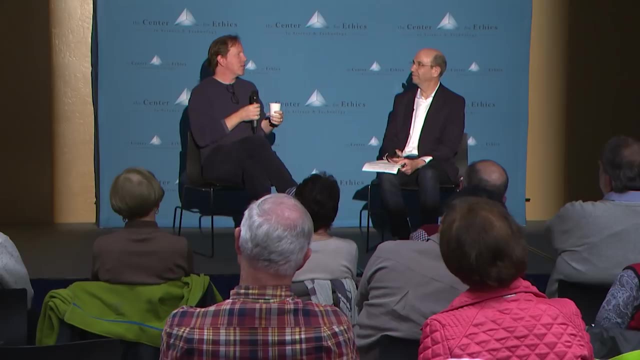 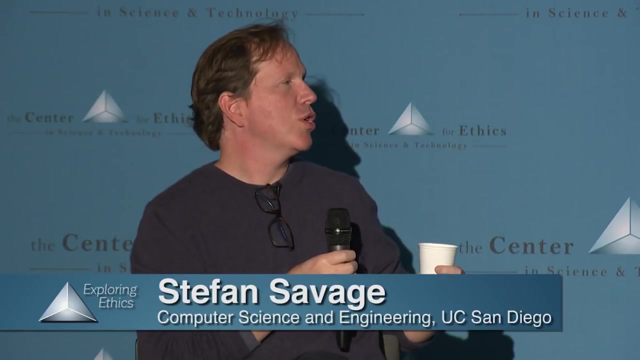 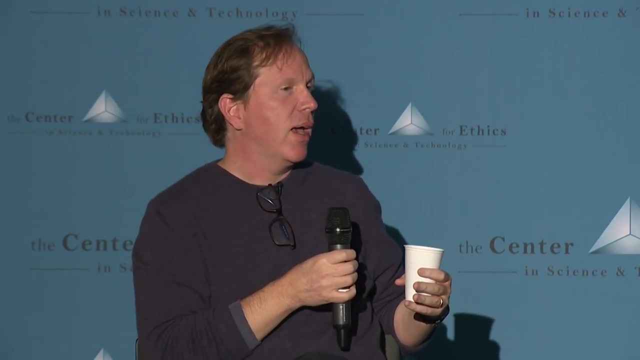 don't think that's what the majority of them are being used for. but I think on balance- you know this is what you end up weighing when you do these kinds of things- is: are your expected benefits from having done the research? do they outweigh your expected negative impacts? sometimes you can get surprised in either direction. 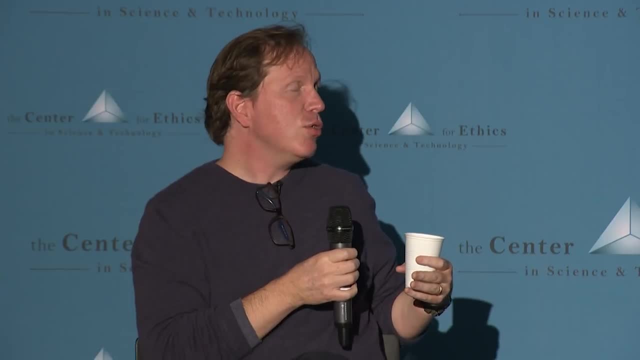 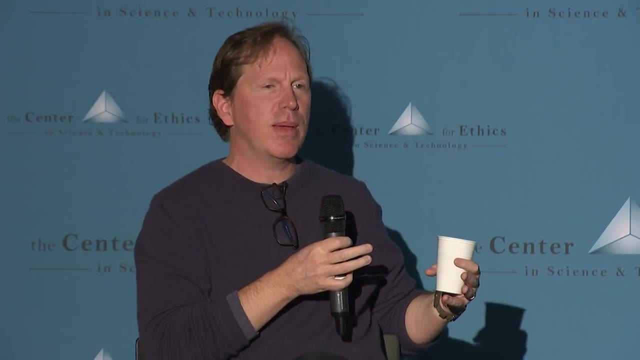 and so you know you do your best to make those guesses and you usually have. you know all of these questions are some combination of different ethical systems. so what I just described here, this balancing test about outcomes, is you know what we would call. you know deontological ethics, but 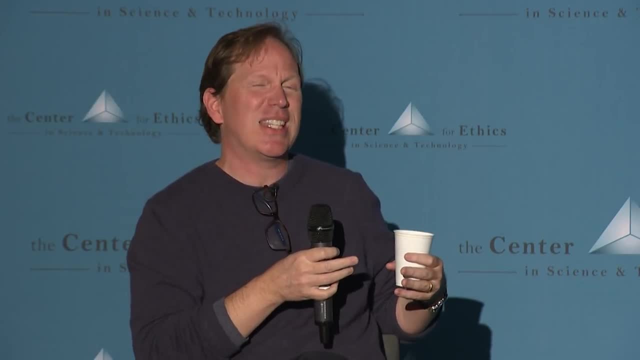 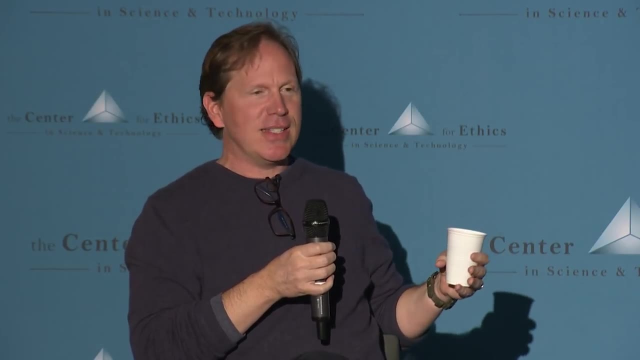 there are certain things you just won't do, and that's where kind of virtue ethics comes in. it's like, okay, I have this balancing test between what are the positives and the negatives, but no matter how good the positive is, you know, I'm not gonna shoot somebody. it's just I'm like there's, there's not enough. 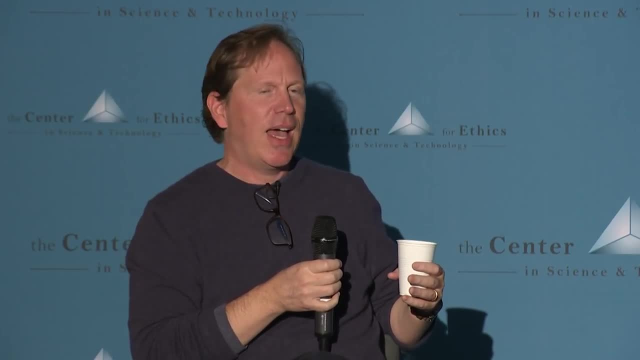 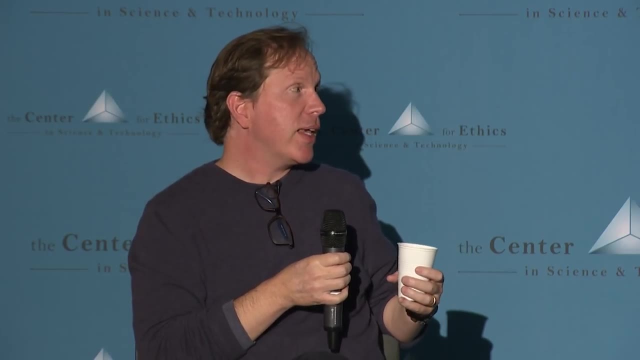 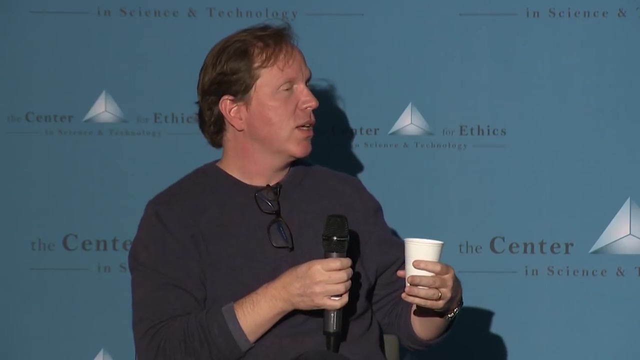 positives for me to go and do that and capture-solving. the costs are relatively modest. it also helped that we were very careful, whenever we engage with that ecosystem, that we were working in the context of the thing that we're the context, the people who were being abused we would partner with. 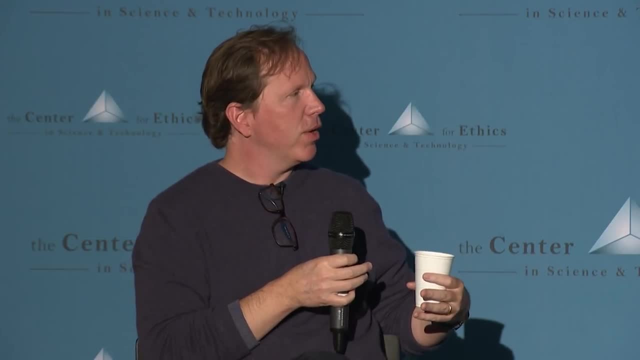 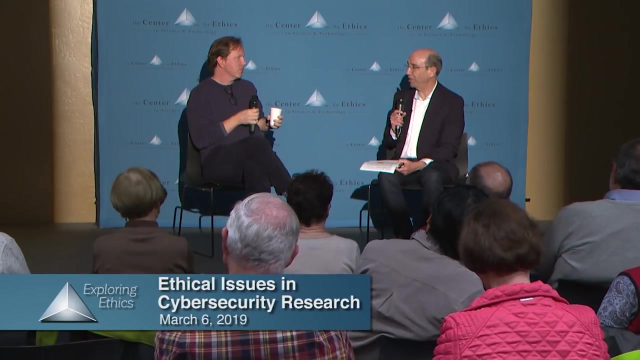 When we were dealing with stuff related to Google, Google would be a partner in our work. They were the ones, in some sense, upon whom the abuse was being visited. That makes sense. You actually have touched on another general question that I need to preface a little bit. 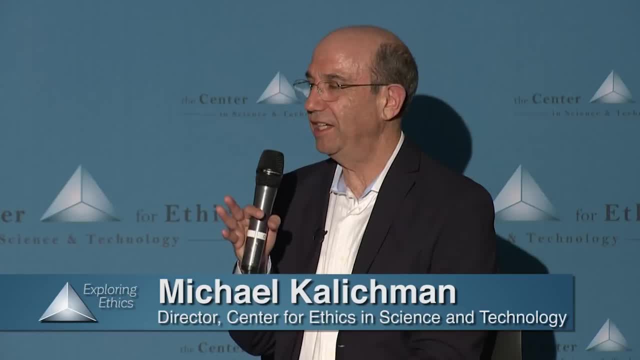 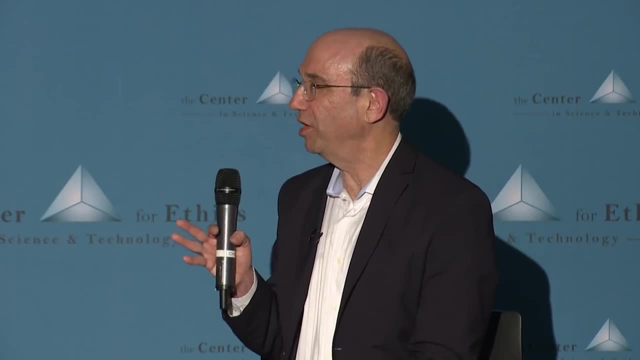 Most of the topics we have in this program are topics where you say: here is something we do and there are some downsides to this. What should we do about it? Actually, most of what you do is trying to do something about a problem that we have. 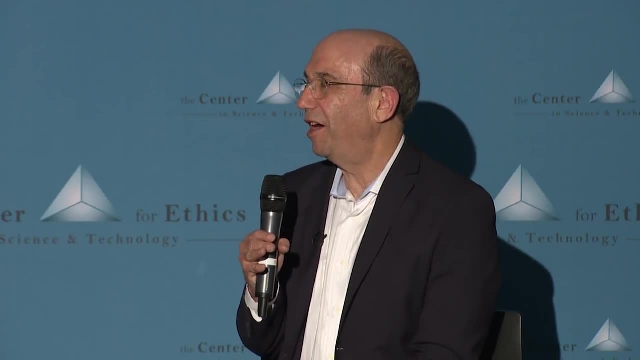 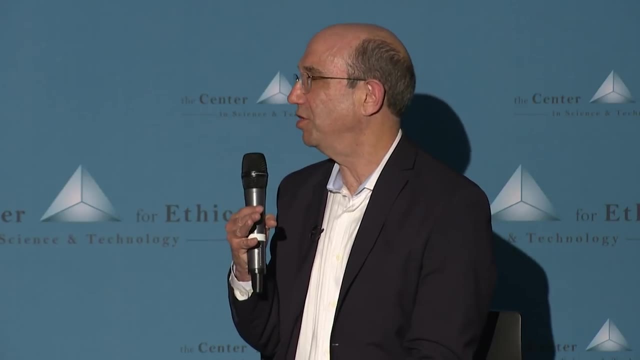 with the Internet, broadly speaking. Yet even within your desire to do that, there are questions. One is on the research side and the other, in other words, how do you do research? The other is how your research might be used. 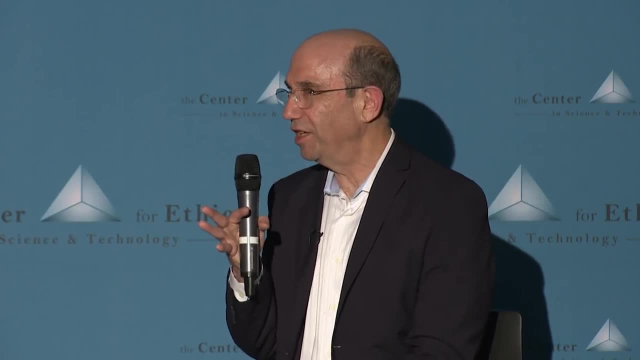 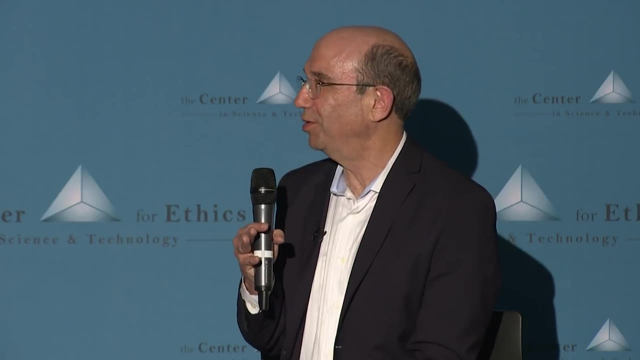 You talk about how your research is done. During the break it sounded like you were talking a little bit about a question of how you get approval from the university to be able to do questionable things. Can you talk for a moment about: do you have to have human subjects committee review? what? 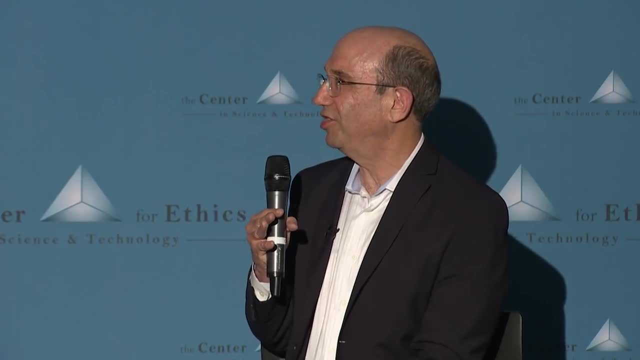 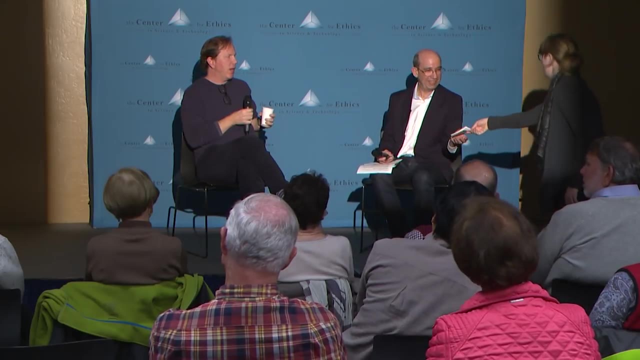 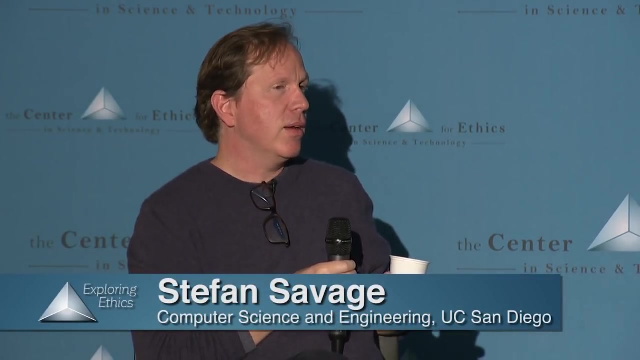 you're doing? You've talked to campus council. Who do you talk to? Who is watching you? It depends on the project. There are going to be a variety of different topics, People who need to be involved. If we are dealing with any research that directly involves human subjects, then there's going. 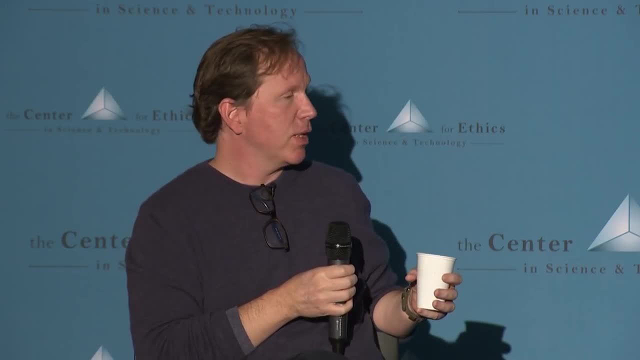 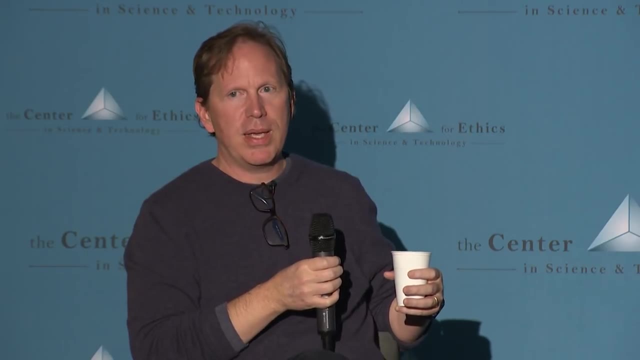 to be an institutional review board that we need to submit something to, where they need to understand what are the risks of the research to those people and what controls do we have in place. and then they need to approve it before we can move forward. 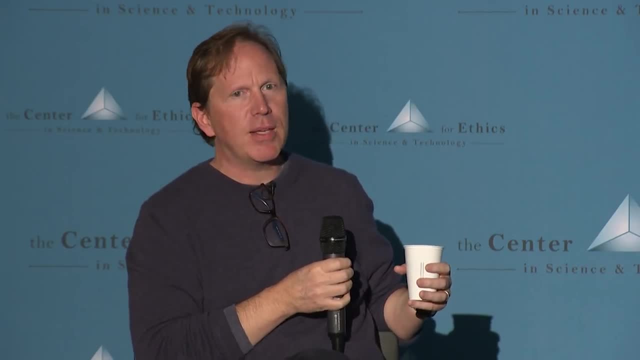 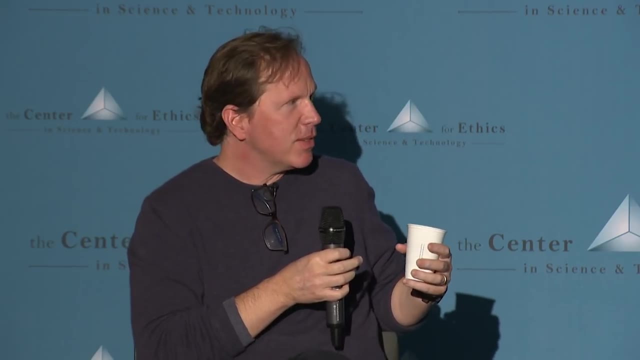 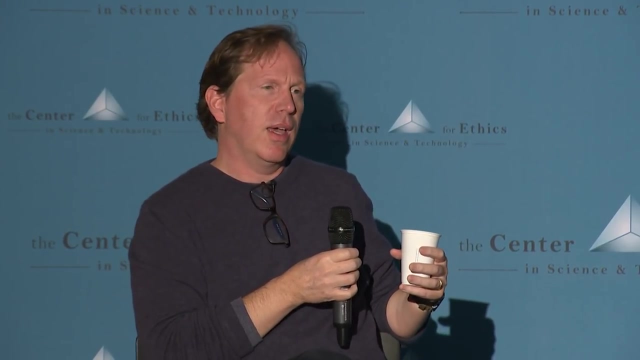 That is a subset of ethics. That is, I think, my community. It frequently likes to waive having a human subjects review as the badge of ethics. It covers a subset of ethical challenges, Like I'll give you an example. There are no human subject issues in the General Motors, the car work that I did. 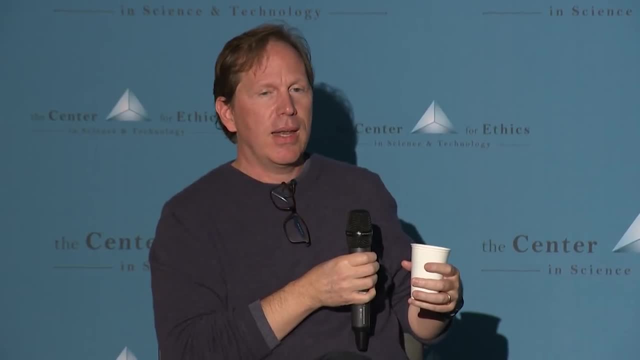 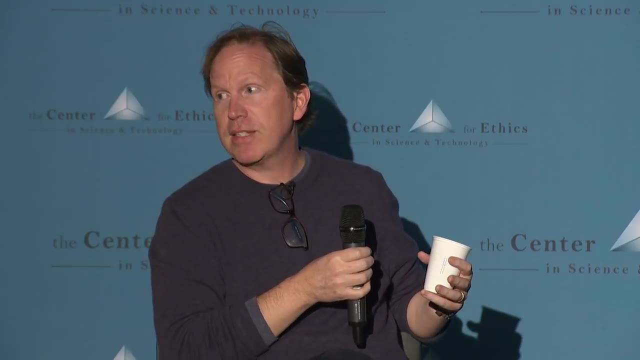 One of our concerns when we did this was that at the time we did it, General Motors was basically in receivership to the US government. They were, They had effectively just escaped bankruptcy by the US government coming in And supporting them, And this was right. after that. 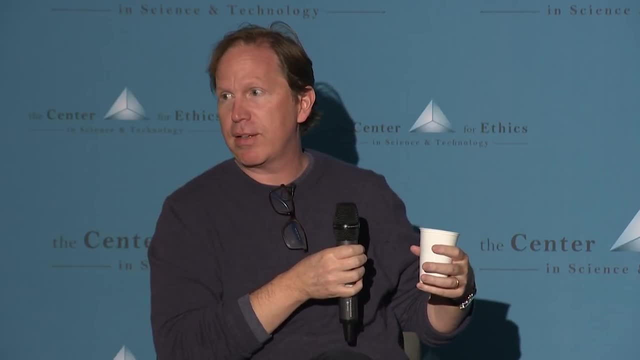 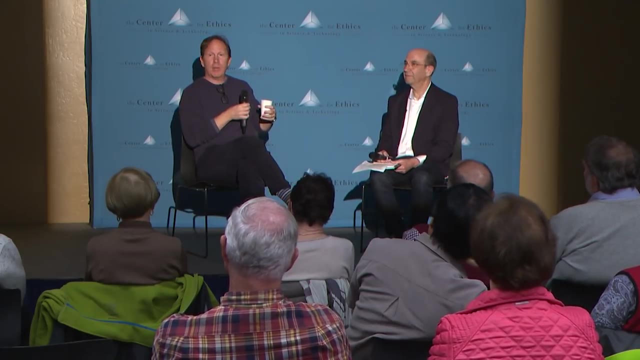 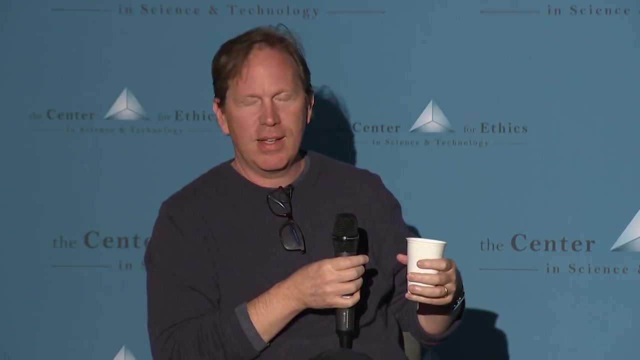 And it was just after the Toyota unintended acceleration debacle. that cost Toyota a huge amount of money And there was significant worry If we had come out. By the way, we did not go and publish any paper ever that said it was General Motors cars can all be taken over. 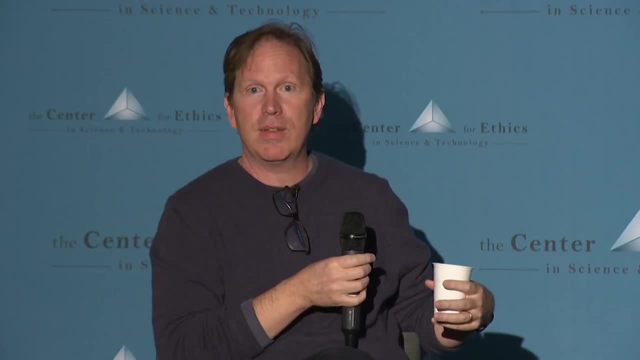 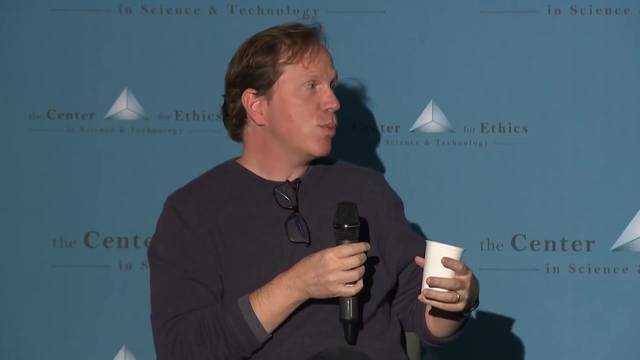 We never disclosed who it was. We never disclosed how to do it, Even in- Which was an odd thing to do in a research paper, where you don't describe exactly what you did. But among the issues where we didn't want, It would have been the largest recall in US history if they had been forced to do a recall. 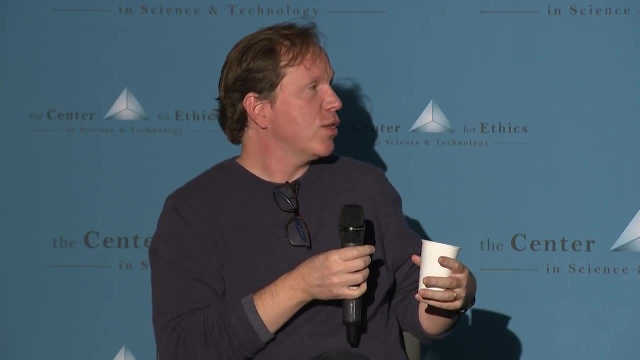 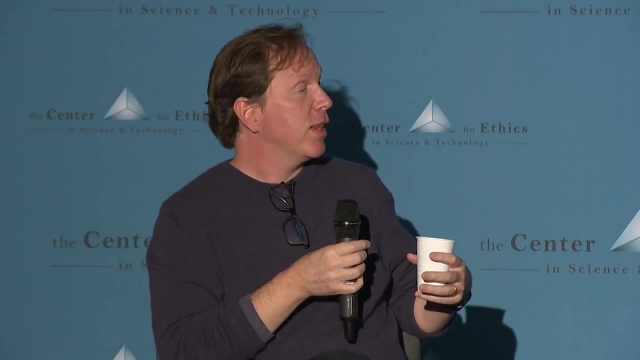 because of this, And it's quite likely a lot of people would have lost their jobs, And a human subjects board will not. That's not their job, They won't look at that, And so for that we don't necessarily have people to turn to. 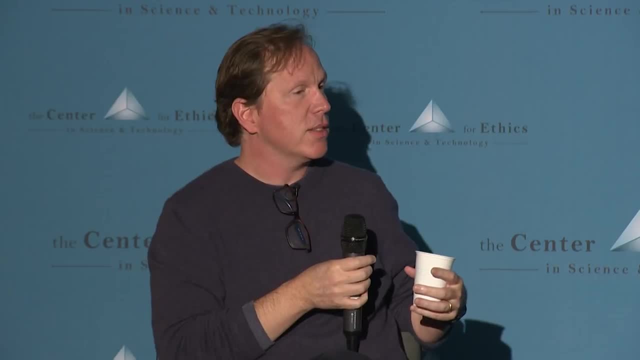 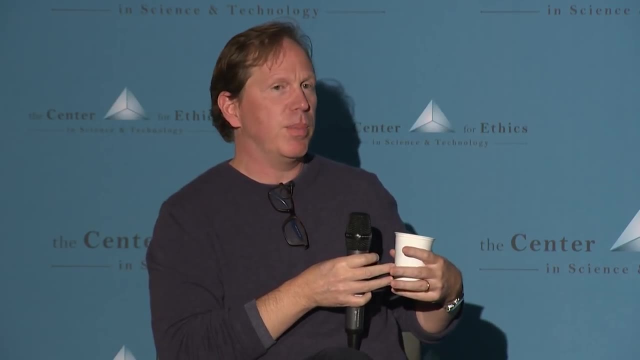 There is not like an independent ethics review board that looks at that. We have to think about that ourselves. For other things we have legal. We go to campus council for things that are legal And legal intersects with ethics. It intersects with ethical but is actually quite different. 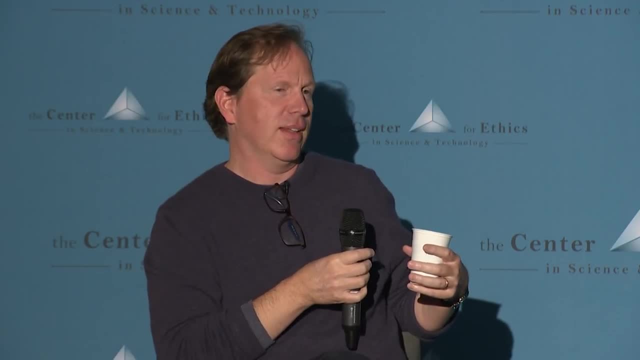 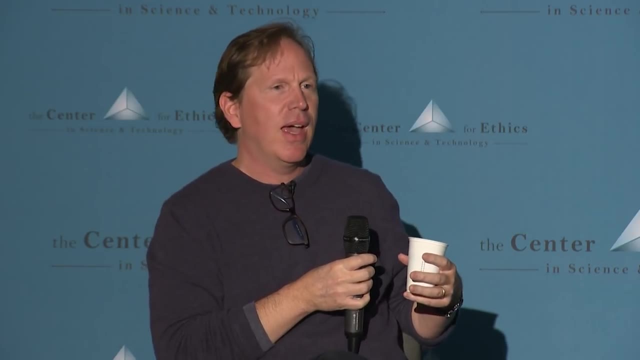 You can be ethical and legal And you can be ethical and illegal, And vice versa. I mean, it's pretty amazing that every combination of the two exists in real life, And so any time we know we are going to touch on something where there is the potential. 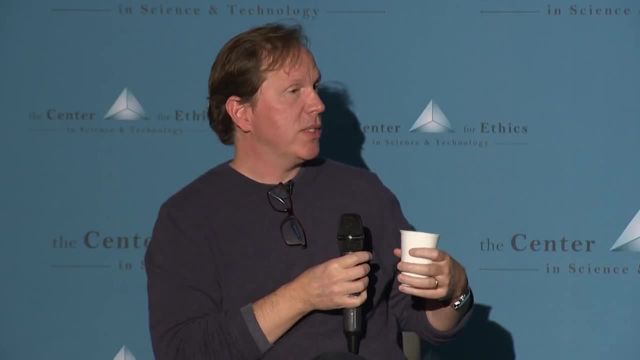 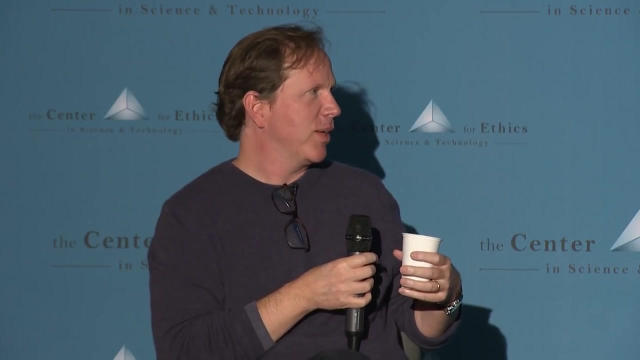 for either criminal liability or, where there is the potential for- And I think So- first approximation. campus council is much more concerned about civil liability because the US Attorney's Office by and large is not obsessed with suing university professors for doing measurement projects. 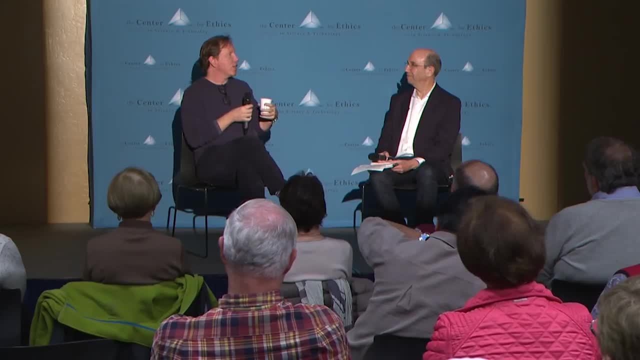 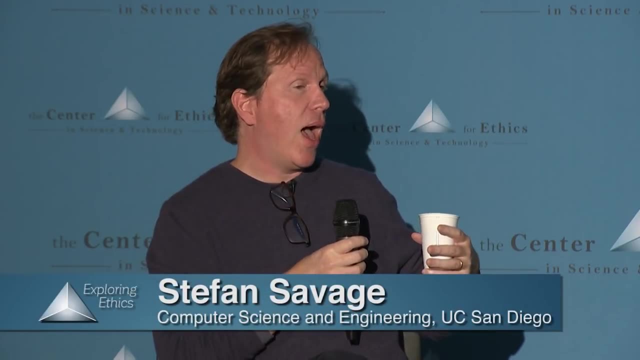 Then we end up Before we even start designing the project, we go to general counsel and get them to talk to us about it. But then there are other things. when we want a resource, Like I needed to have these special credit cards, I needed to have these special credit cards. 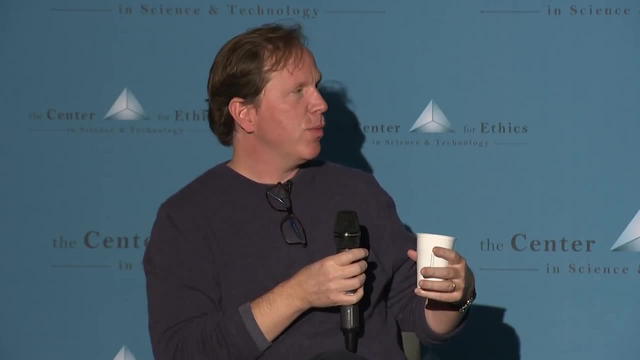 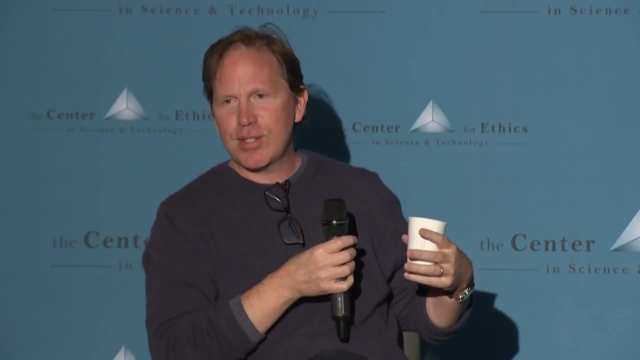 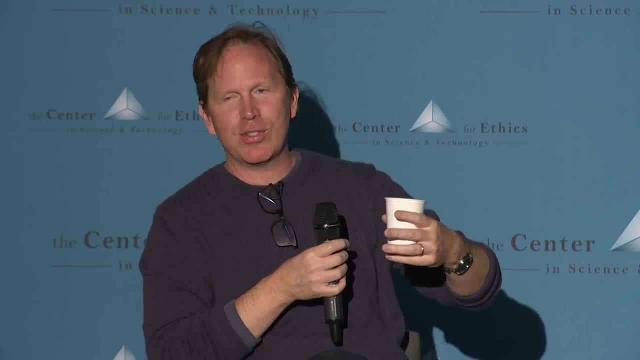 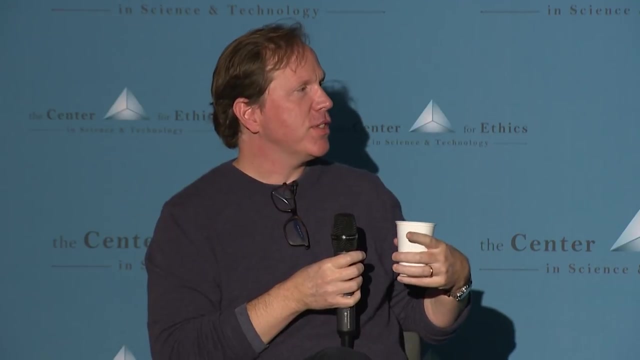 And imagine going to an institution as conservative as a university and say: and by the way, I need credit cards under different names for buying illegal drugs, and they're going to steal the money too. Okay, And that actually had to go all the way to the Office of the President and the Office. 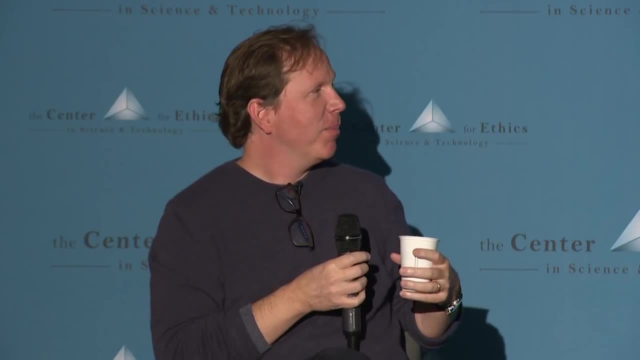 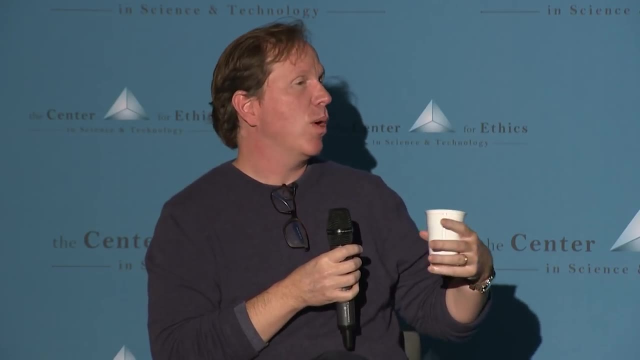 of Research Compliance And that was a legendary meeting. But they were very supportive in the end once we explained why there weren't easier alternatives and what we were going to do to keep everything controlled. And so you document your process meticulously And they asked us to do certain things. 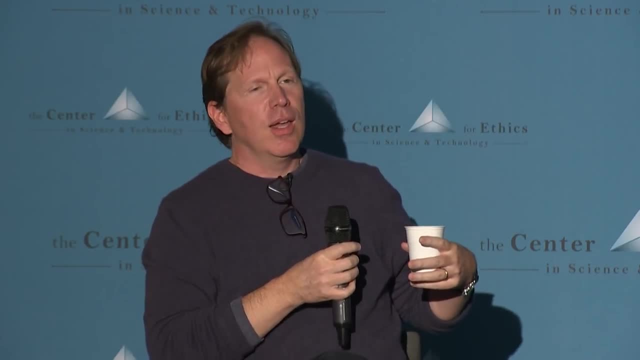 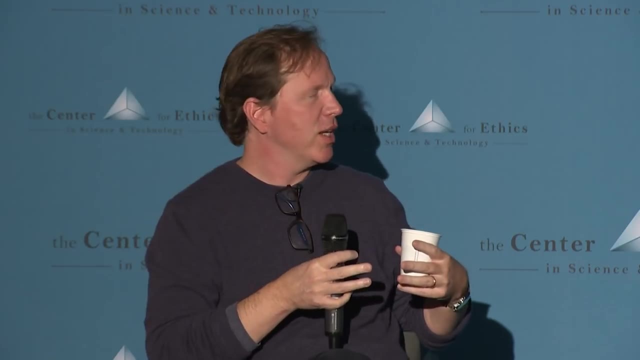 like we had this special lock on the door And we limited which drugs we were going to buy according to the University of California's interpretation of California drug importation law, And so there were always some back and forth to design the methodology in a way. 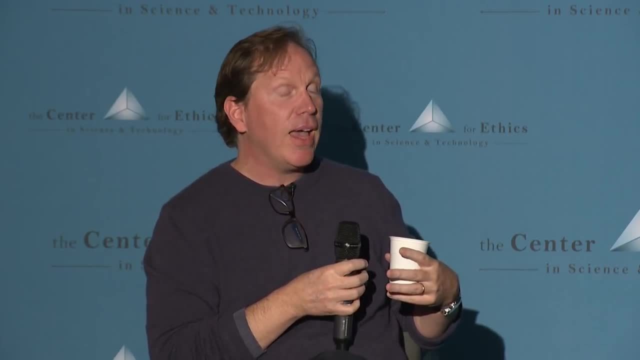 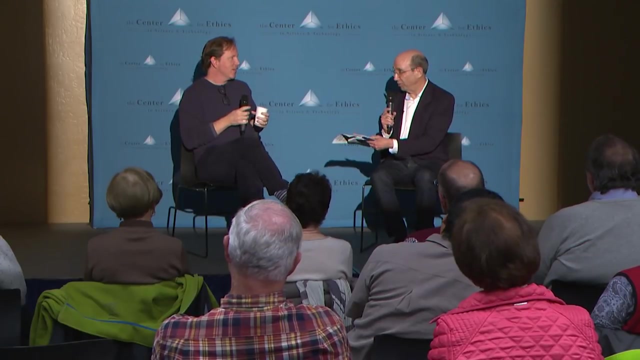 that would be in compliance, But I have ended up at various times needing to deal with a lot of different parts of campus. It's not as singular as just human subjects, So this is the first time I've met you in person. I have the feeling that you are extremely 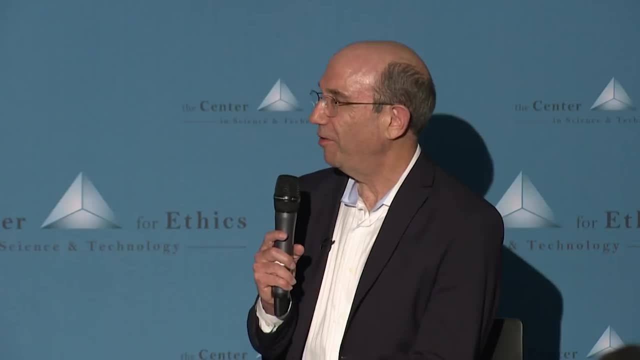 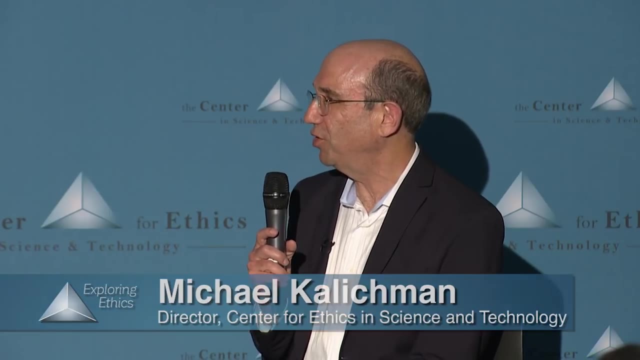 thoughtful and careful about doing these things, which is great. But it seems to me that a lot of this depends on you. I mean, I'm just trying to figure out how much of this could have been done by you without asking those questions. 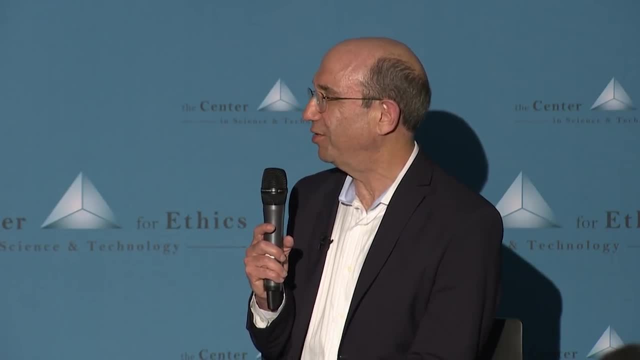 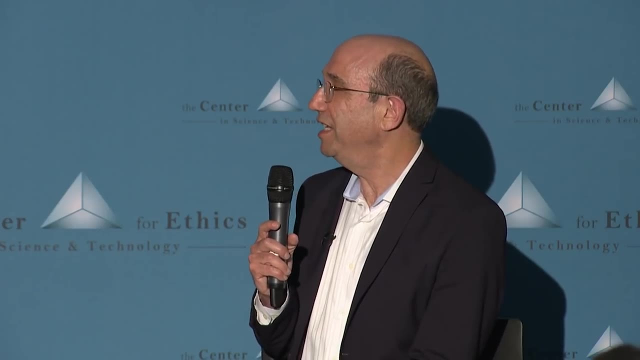 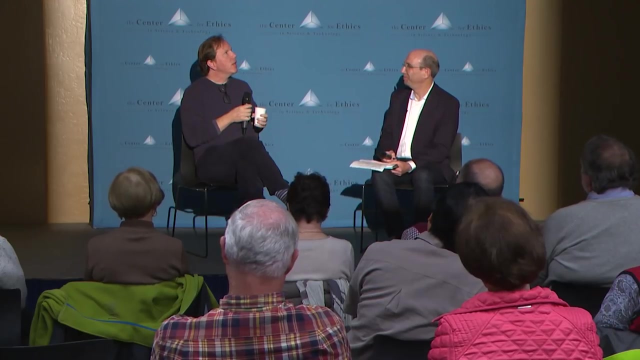 How far could you have gone to get those credit cards to buy those drugs? So this is a legitimate question. I mean, do we need that independent review board for what computer scientists might be doing? So I don't understand the difference. The two questions seem different. 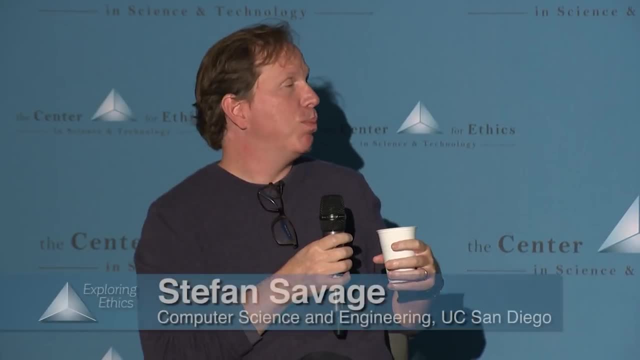 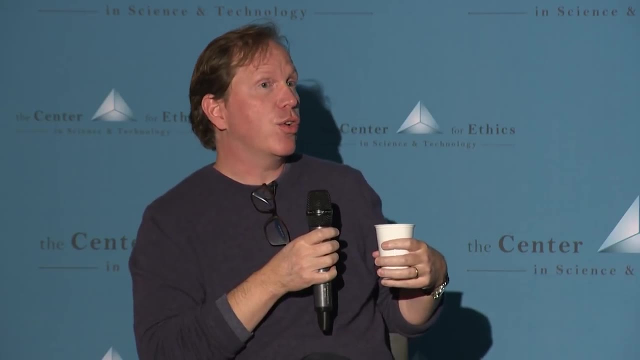 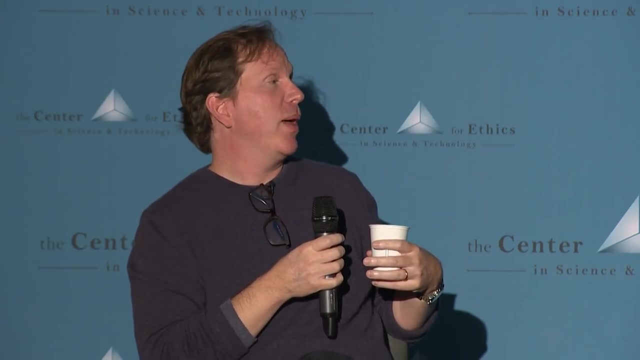 There's the one. could I have done it without? could I have just broken all of our policy rules and done it independently, Like I think I could have, but for the resource issue? So I guess I could have spent all my own money on that stuff. 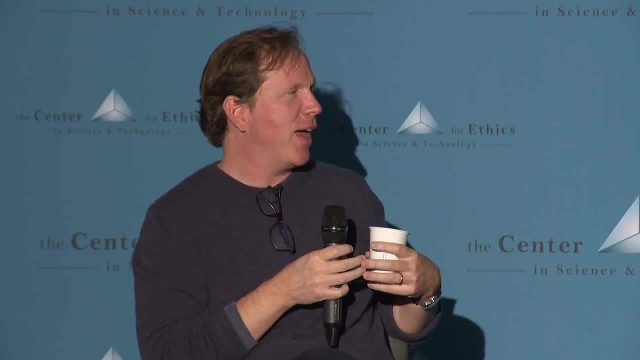 as opposed to using the money that our research sponsors provided, But that would have made it a less attractive activity, But technically, nothing would have prevented me from doing what I was doing. I think I would have felt much more nervous. I think one of the things that puts us 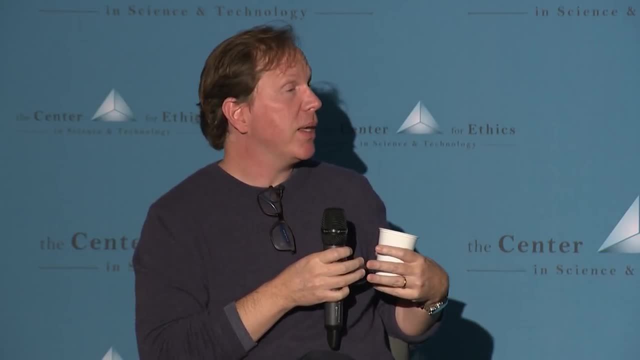 in a much stronger position when we present our work is being able, because people ask: how in the world did you do that, surely? And then that we are able to explain at great lengths the kinds of things that we did in order to control us. 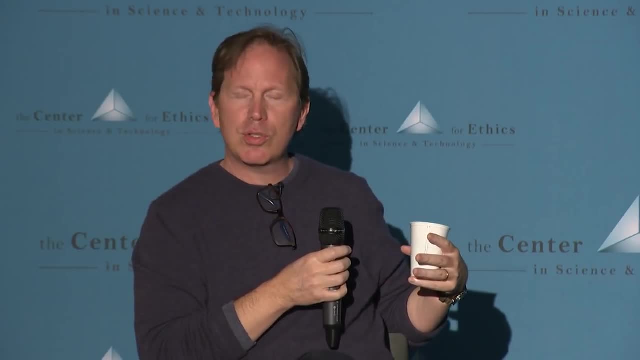 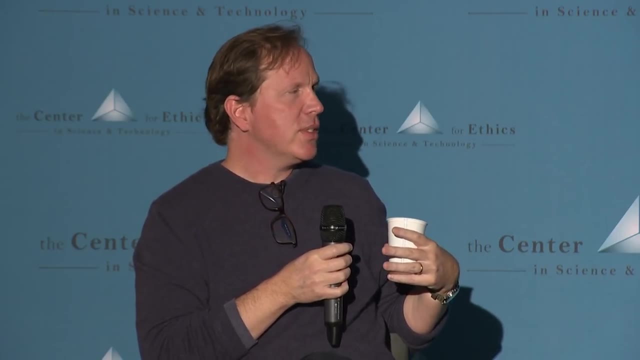 Now I will say that in the computer science community there's been a tremendous evolution over the last two decades. You know, In the mid-'90s it was very much a cowboy mentality. All kinds of crazy things got done without any notion. 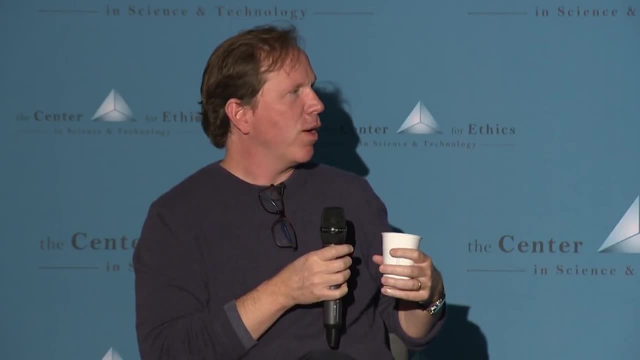 The human subjects was something for doctors or pharmaceutical people. It was not something that people in my world did, And you would routinely read papers where they said, oh, and we tapped an optical tap and then grabbed all of the traffic going in and out of our institution. 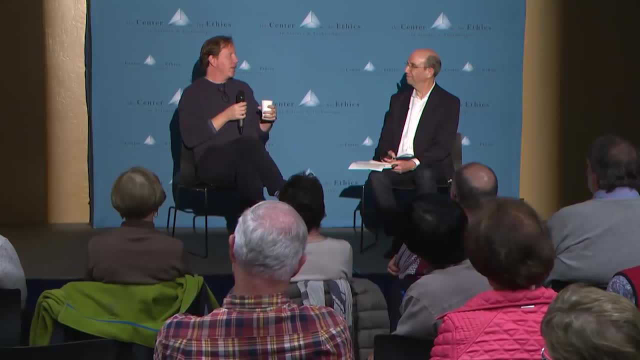 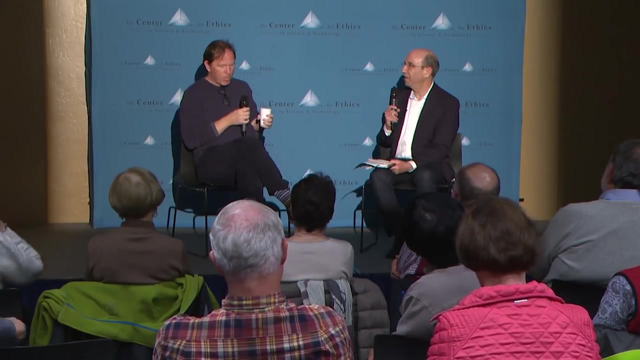 and all of this other stuff. And now you know you couldn't get that paper accepted without a long explanation for how it was that what you did was actually OK. So that actually is, I think, a shift in those years for that field. 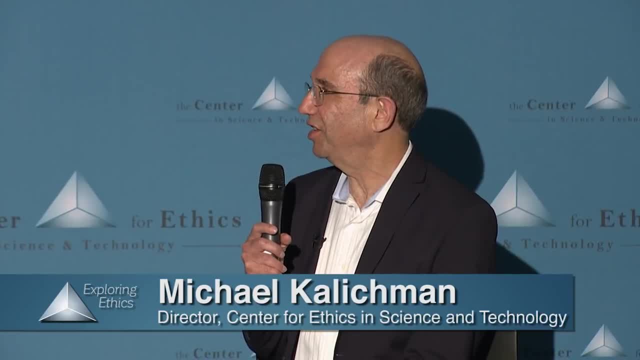 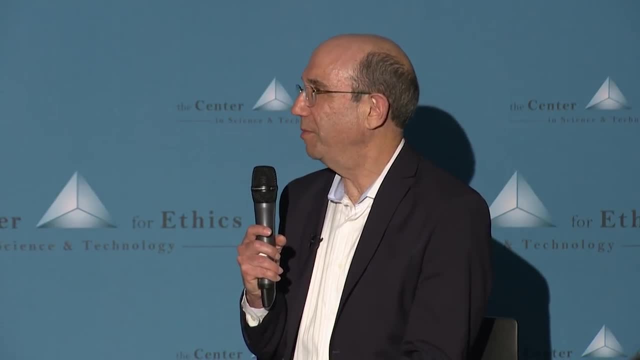 But what I was thinking is that it sounds like you felt that at certain junctures you weren't required to get human subjects review. There was no committee to look at some of the ethical questions that you came up with, So you asked those questions. 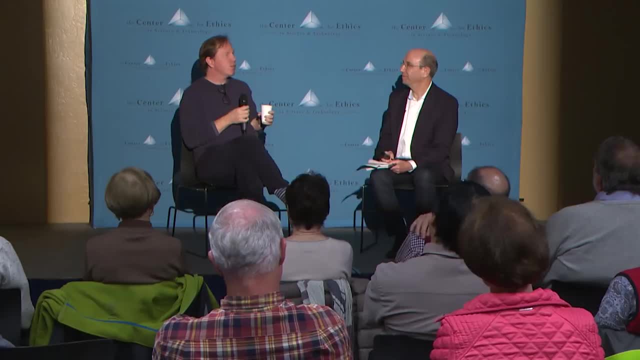 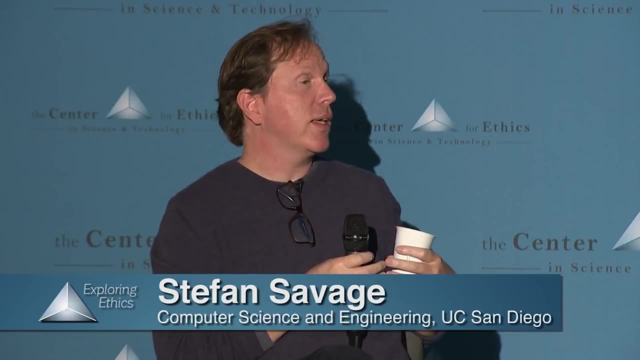 Ah, ah, ah. Yeah, There are portions for which there is no special question, There's no committee. Yeah, that's absolutely right. And it's not clear where you quite draw those boundaries, because it's certainly the case that there's, even in the strongest advocates. 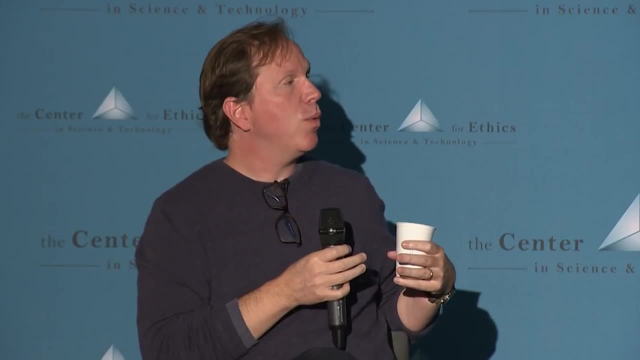 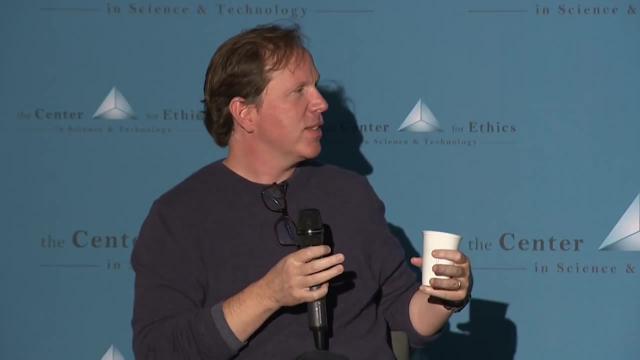 for ethical oversight, I've yet to hear one where they were thinking of protecting the fiduciary interests of a company That's not usually in the remit of, And so I think different people would have different points of view on this, And in fact I know there are other researchers. 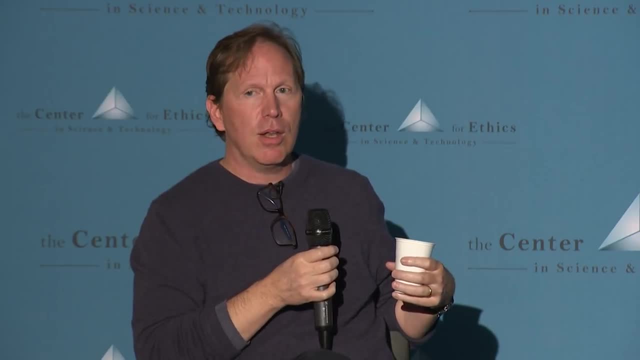 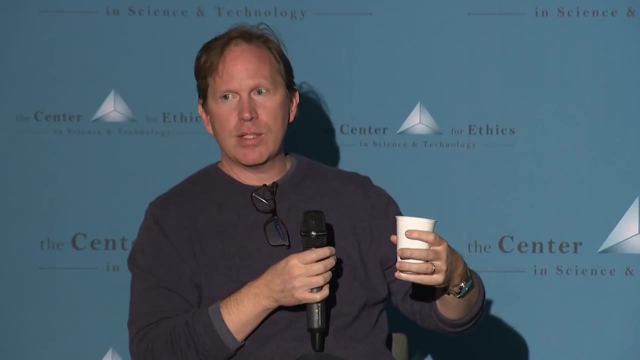 I know there are other people who took very different points of view and, for example, said: no, we disagree with the choice you made. You should have come out and disclosed everything as a way to force the issue, and that the shaming of the company. 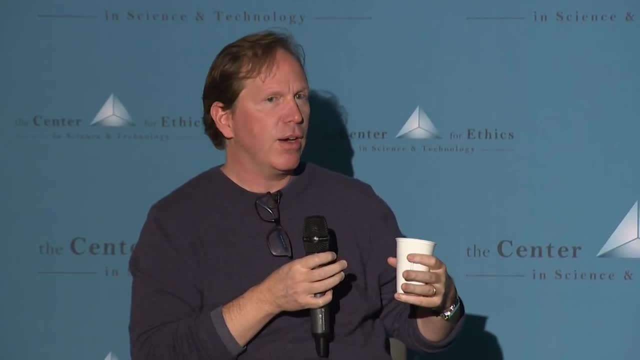 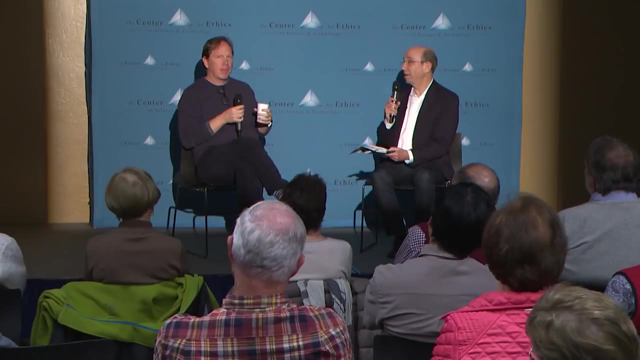 would have driven them to go and fix this stuff more quickly, And there, I think, are differences of opinion on the cost-benefit analysis of those kinds of choices. So one option, of course, would be to require all faculty doing projects like this to come and speak to the public. 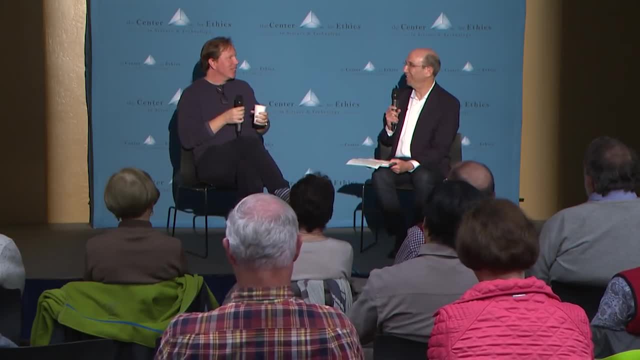 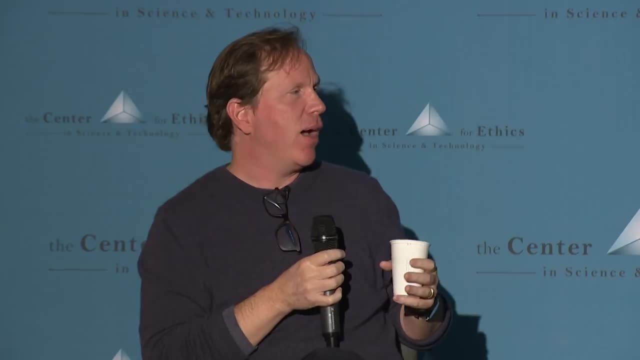 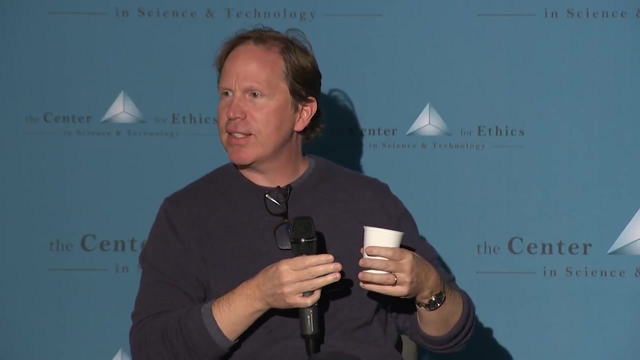 and ask them: what are the issues you see that we should be addressing? I actually think that being able to have a broader set of inputs about where the questions are I think is really valuable, Because there is this kind of groupthink that goes on when you do research in any field. 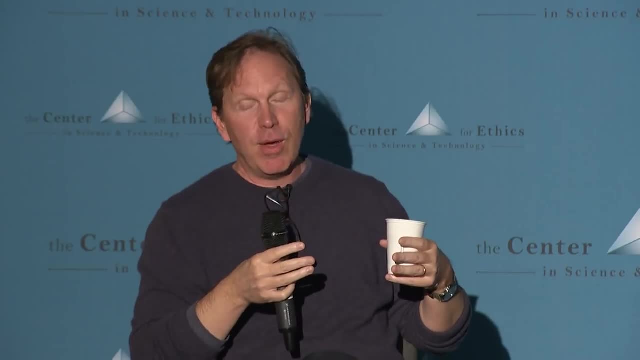 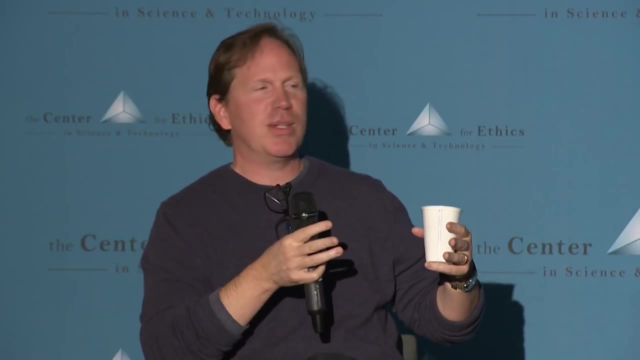 because you're so focused on the prize that you have to take an effort to step back and say, all right, how would other people feel when it was described what we did in the following way: So this is all a good segue to some of the questions. 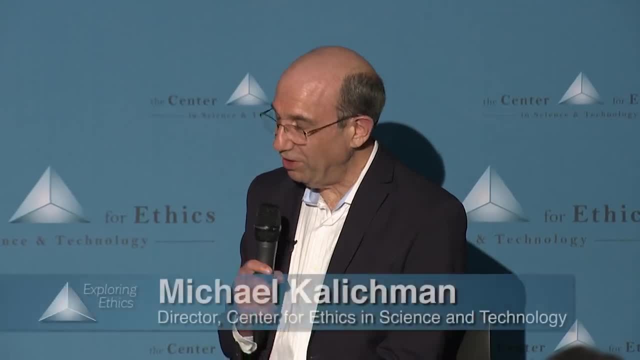 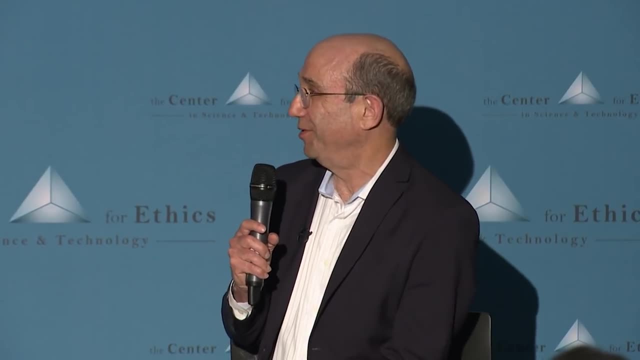 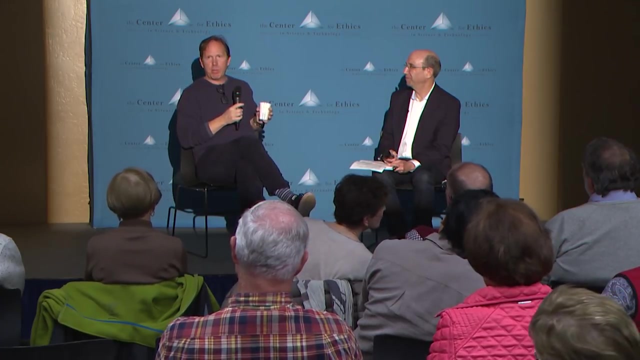 And the first one is about drugs, And they're wondering what happens with all those drugs you collected. Basically, they're saying: why wasn't it confiscated by customs, or what happened to them? 5% confiscation rate in general, And so one interesting issue in the context of counterfeits. 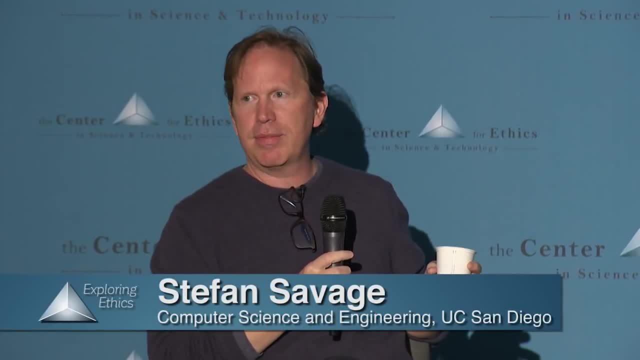 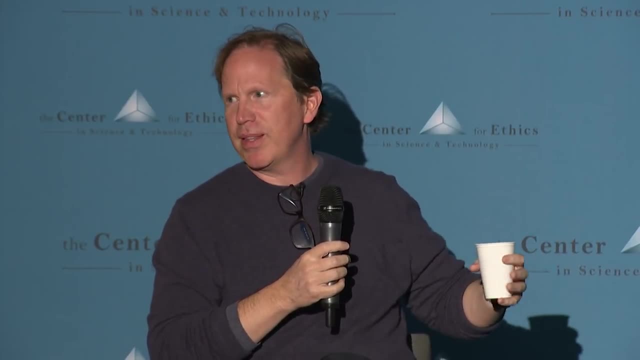 broadly writ is that the previous model of counterfeiting is something that would come in on. you know, container ships into the New York Harbor and then show up on the streets of Canal Street and then have some kind of underground networks. None of that exists anymore. 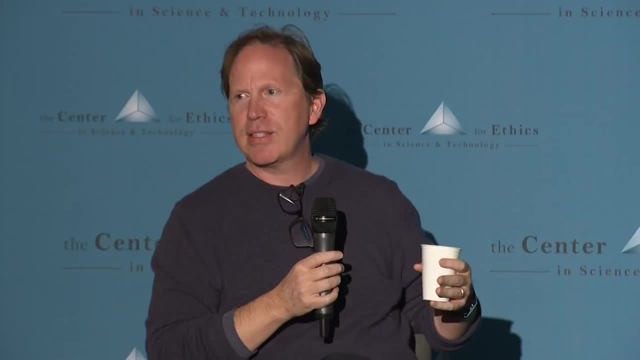 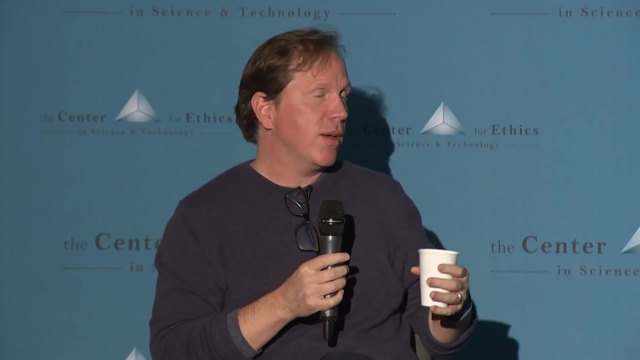 By and large, everything is just shipped direct, And that's for all kinds of counterfeiting, Because we have basically an amazing postal system and package delivery system And the odds of any particular one being interdicted is incredibly small. And when I talked to a postal inspector- 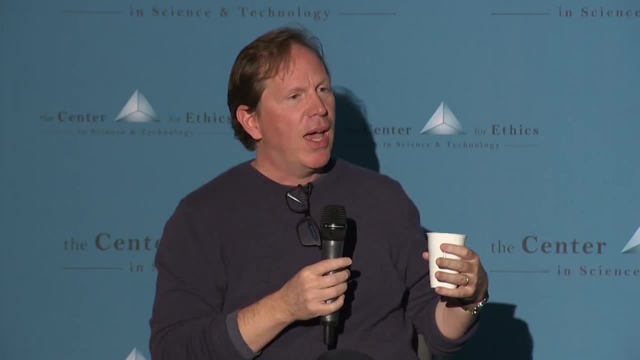 he was very happy that they got 5%. So the reason they didn't is because there's way too much for them to possibly go through all of this stuff and check it As to what eventually happened. so we kept it around for a while to do. 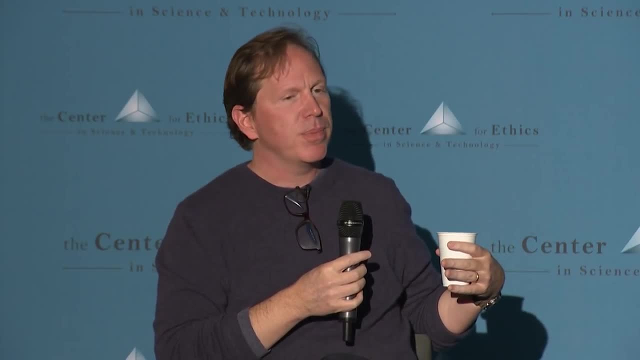 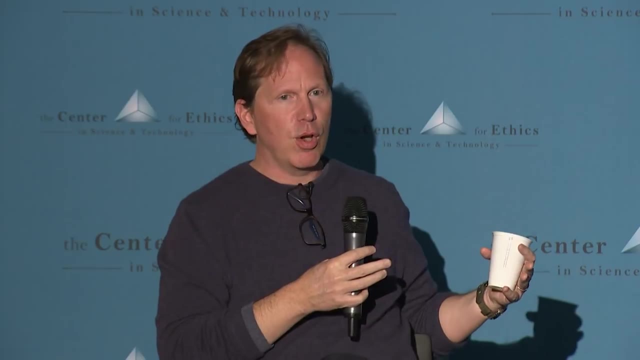 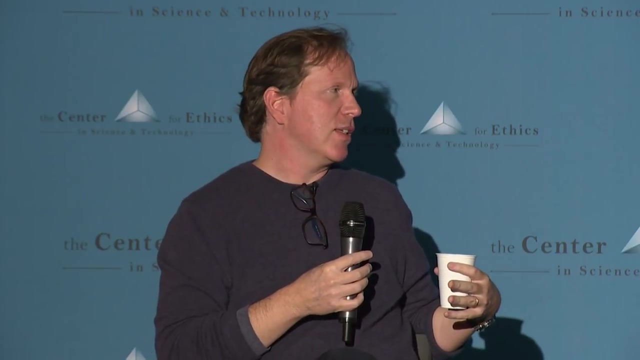 We had a variety of follow-on projects that we're doing. We did some projects because we were curious: are the drugs what they say they are? Because that goes to in some sense, the economic model that the people are pursuing. And then we did some forensic analysis as well. 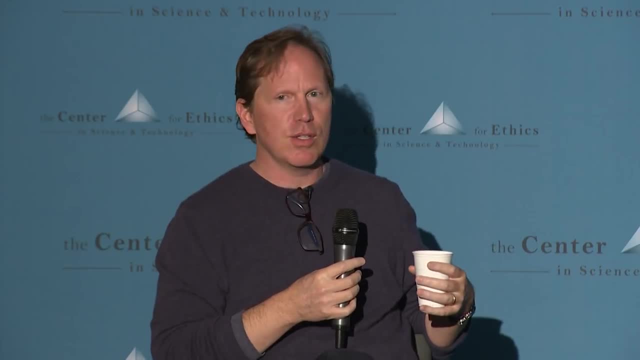 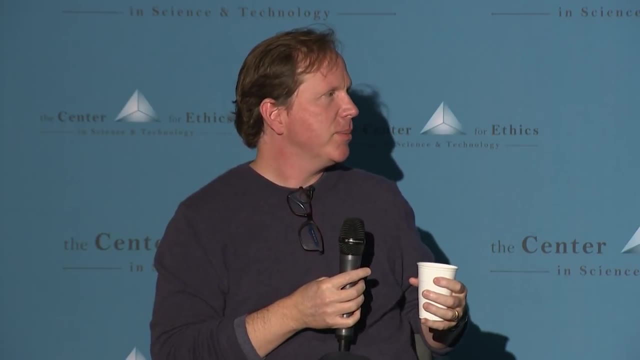 to try to identify commonalities between different suppliers and so forth. Most of them, I think, were eventually destroyed because we didn't have a use for all the stuff that we had had acquired. OK, well put, OK, so all right. 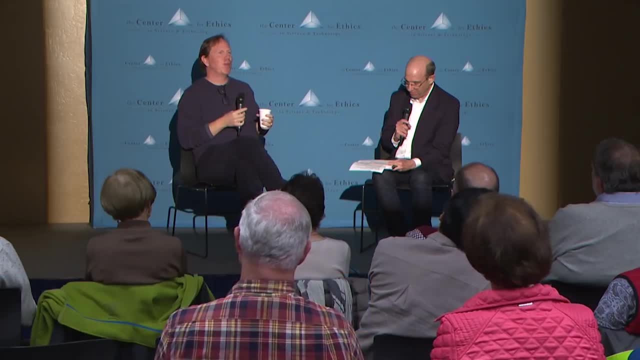 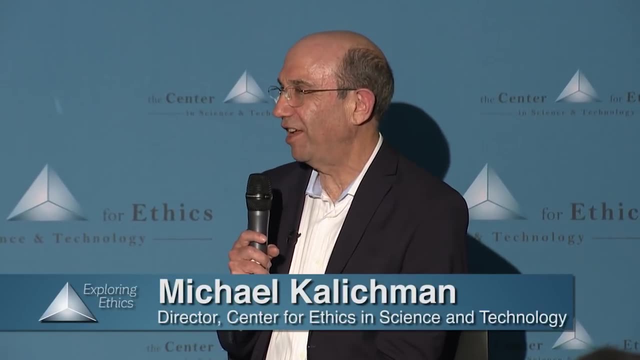 And so let's see, I think we did promise that no one would ingest any of the drugs. Good, Good, I mean, I have to say I suspect a lot of people are thinking what I'm thinking- I think that there should be something more solid in place. 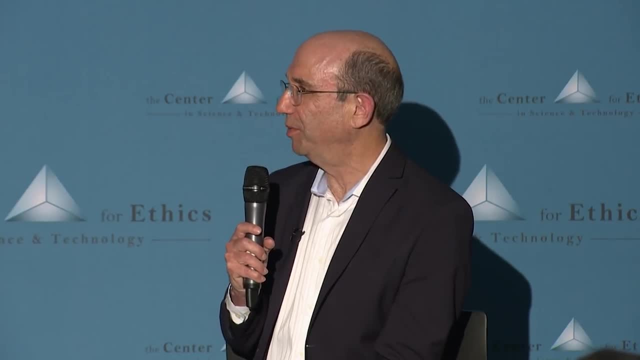 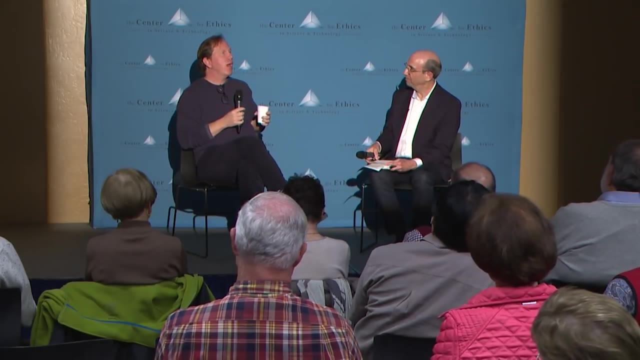 to say, all right, this has arrived, It's sequestered in this room, There's going to be a log, And that somebody is going to say, Oh, all those things existed, Yeah, in some tracks. There was not a person outside of the group whose job it was. 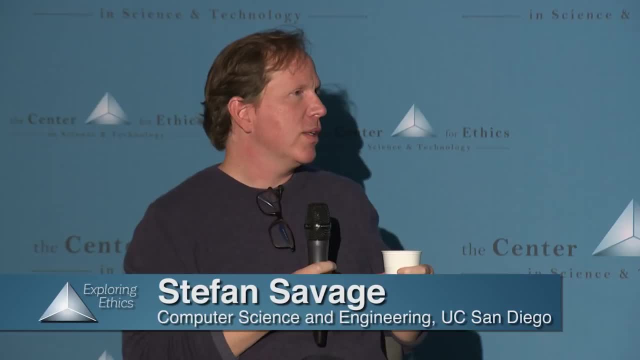 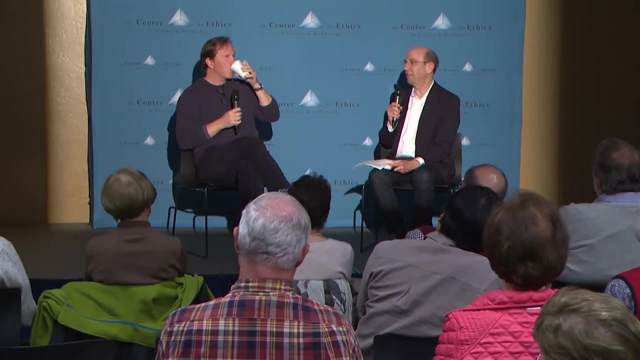 though, to do that, And this is not something that the university has as a service. Yeah, I mean what I'm thinking: that there's a legal problem. There's a legal process where people, for example, do work with animals in laboratories. 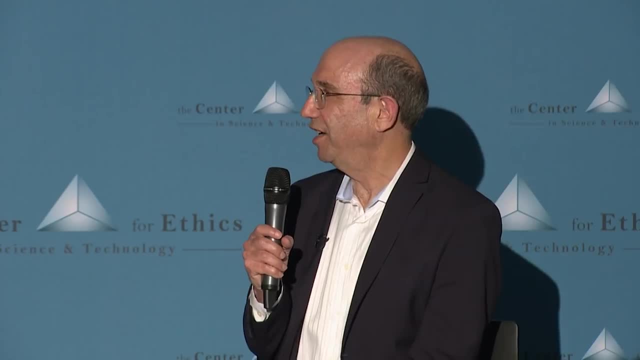 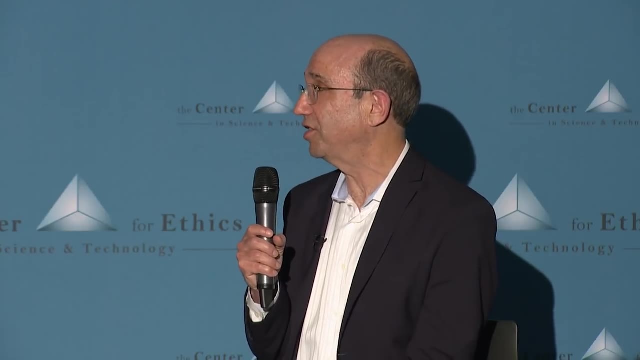 or they're working in hospital settings working with controlled substances. There's a pretty rigorous process of trying to keep track of it, But it's done by the people themselves. There can be external audits, though, of that Absolutely, And we could have always been audited. 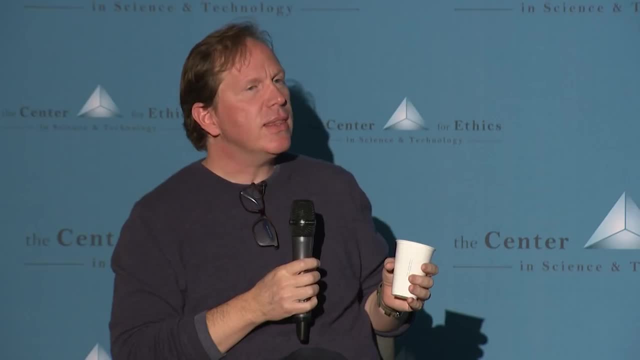 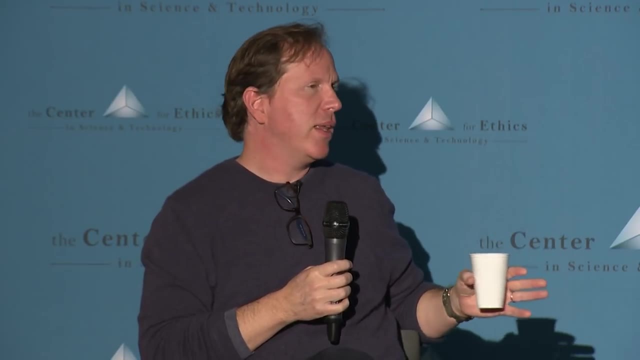 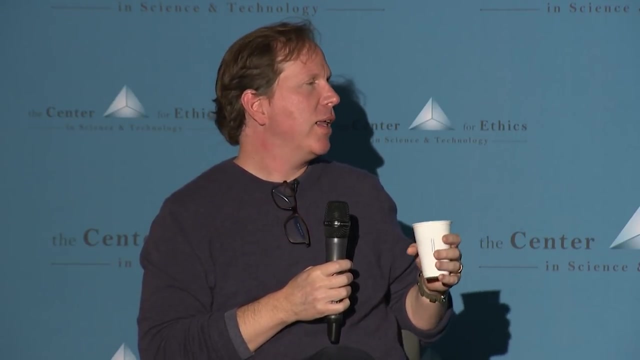 I will say that there were no controlled substances being dealt with And there was nothing that was there was nothing. there were no drugs as part of the many negotiations that we had. There was nothing that had any were attractive for any abuse-oriented purpose. 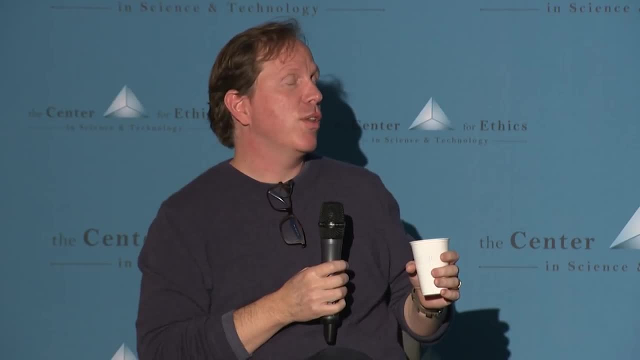 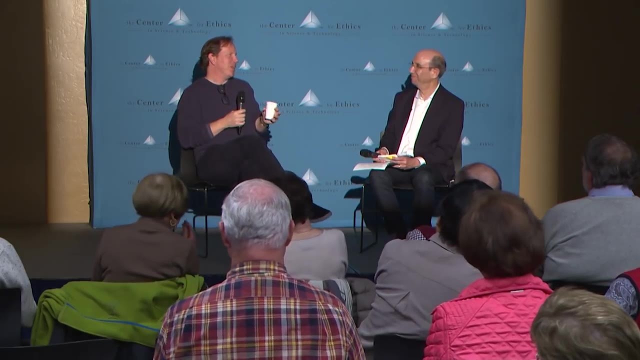 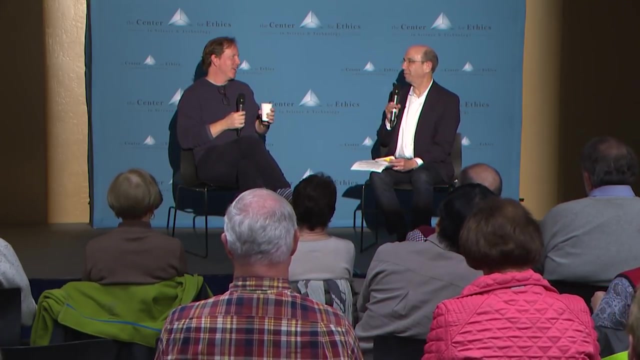 So we cornered the market on counterfeit Claritin, I think for a little while, But it's not like people were breaking in to get that. And just to be clear, we have a talk coming up in the future about political science experiments where they 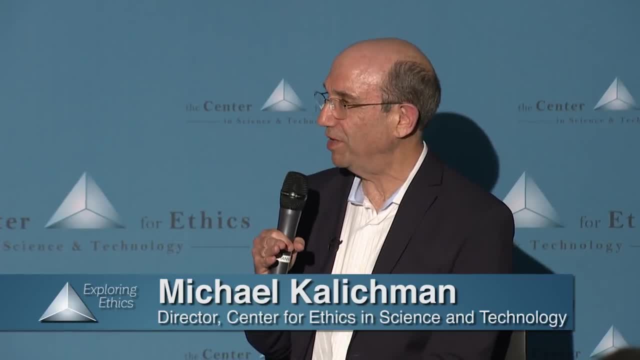 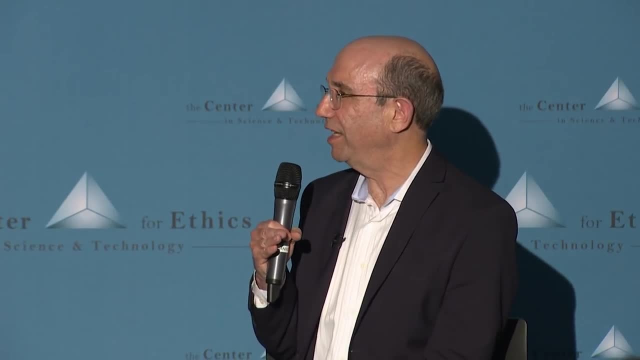 might put money into an election campaign to see what happens, And in certain places that money might be overwhelming. So you shift what's going on. You're pretty confident that the amount that you contributed to this industry was a small percentage of the total. 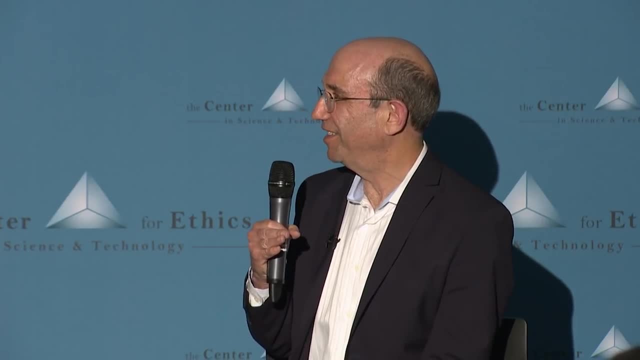 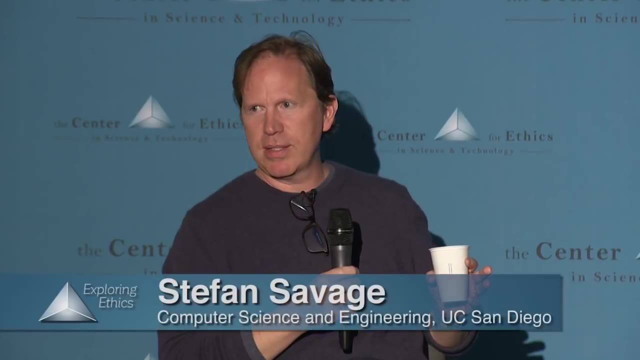 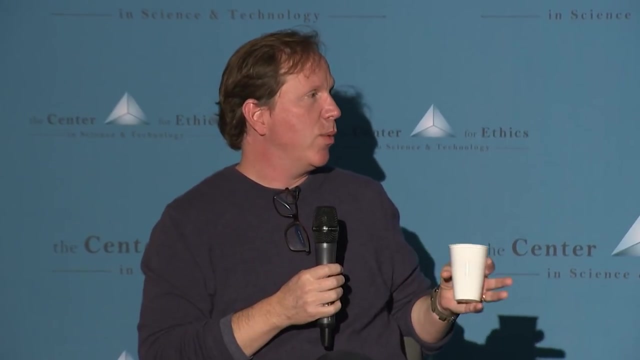 And you didn't somehow prop up some company. that's some rogue company. And this goes to this general question about the ethical issue of giving money to criminal enterprises, who are inherently criminal and up to no good. And is that? Are you making them succeed when they would not? 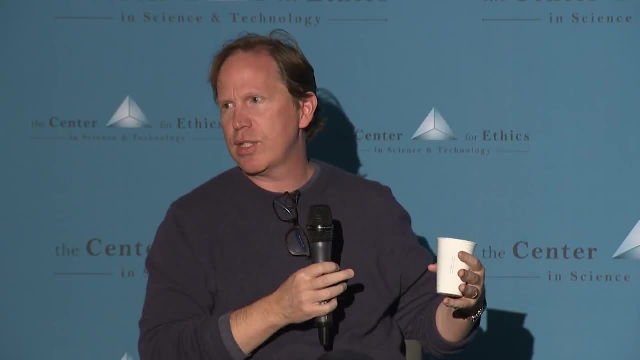 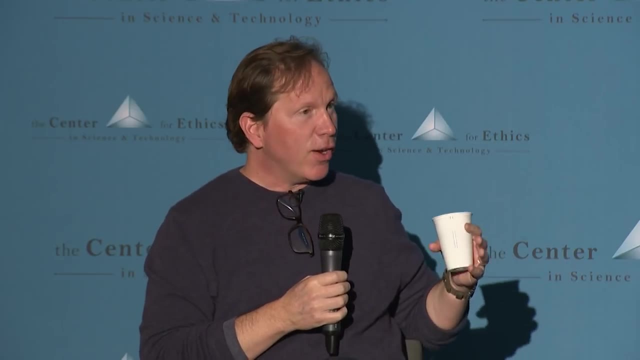 have otherwise. And this is in the alternate world, where you didn't do this work. would we be better off for dint of not having given money to criminals? Now I can say, in these cases, categorically, we were an incredibly tiny fraction. 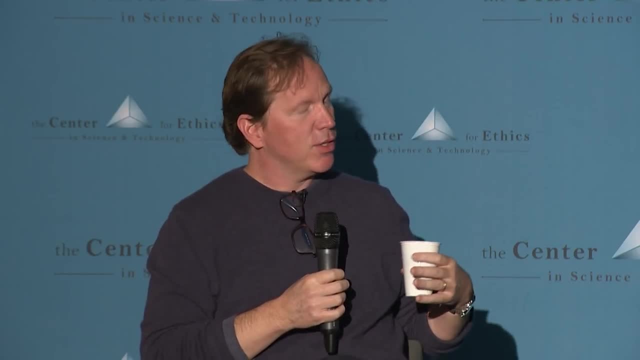 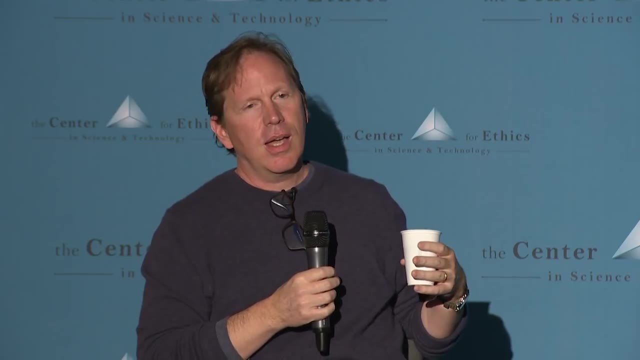 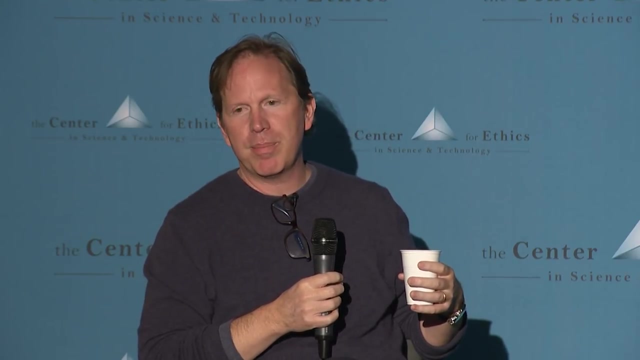 And I can say that categorically because of another piece of research I didn't discuss but has its own ethical issues, which is that the largest counterfeit Russian pharmaceutical organization- And we went to several organizations, most of whom we ended up buying from Because of some, both internal conflicts and conflicts. 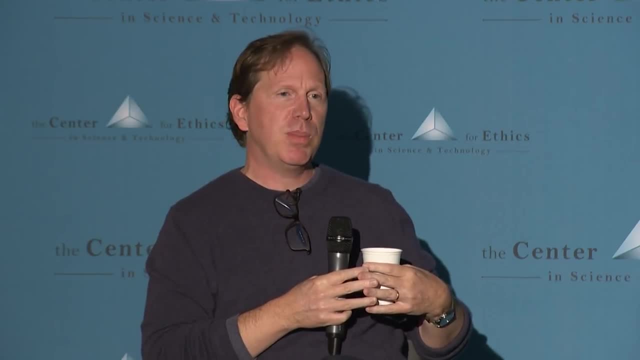 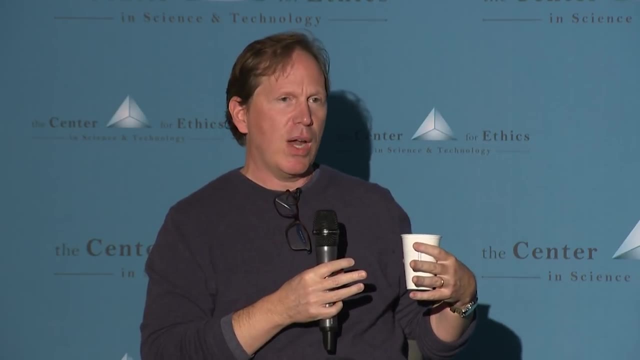 with the Russian state. the FSB, which is the Russian equivalent of the FBI, confiscated some of their computers, imaged their drives and then, through a very complicated chain parts of which I do not entirely understand, the back end server. 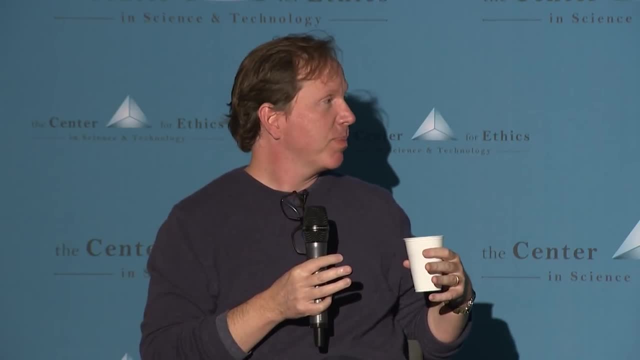 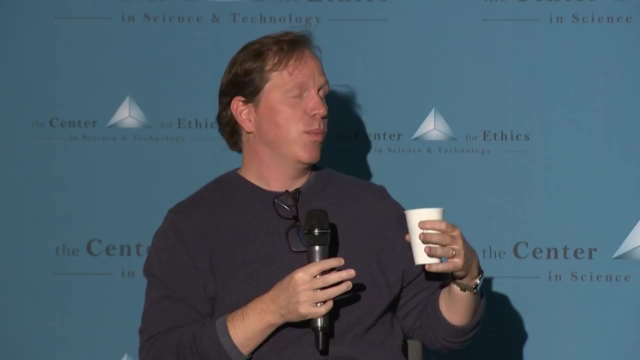 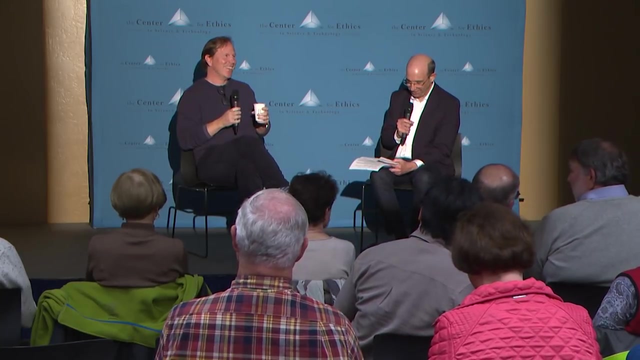 server contents ended up in our lab And so we know every single order that they had And we can identify all of our orders within that, And we were a very small fraction. That's fascinating at many levels and it's good to see how you got that. So somebody. 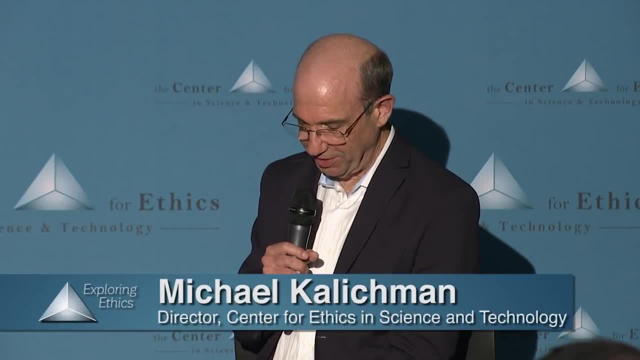 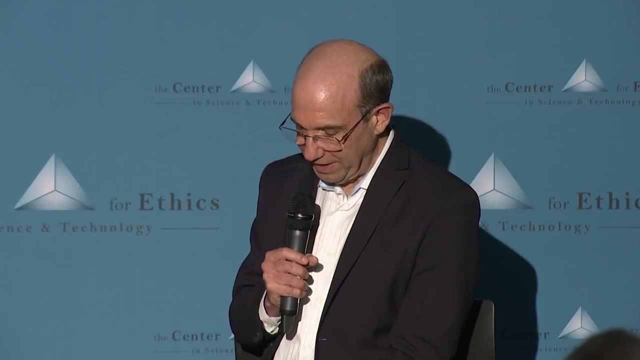 is asking for some very practical, specific question here. Maybe you'll take a stab at answering it. So if, as a result of legitimate participation in internet transactions, you begin to be inundated by unsolicited offers, emails et cetera, would it be unethical for? 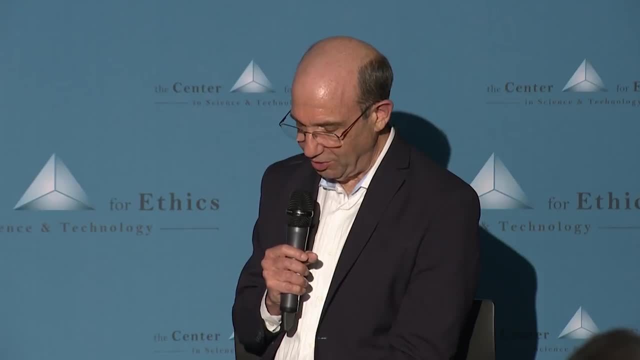 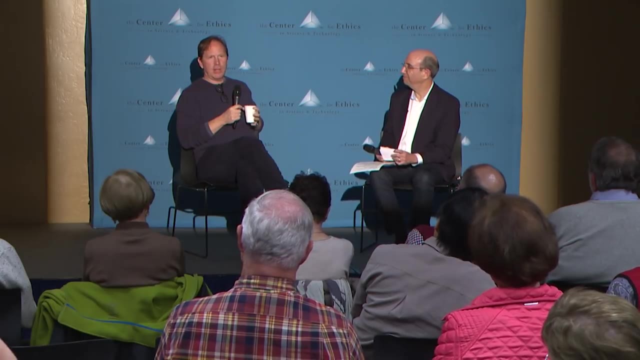 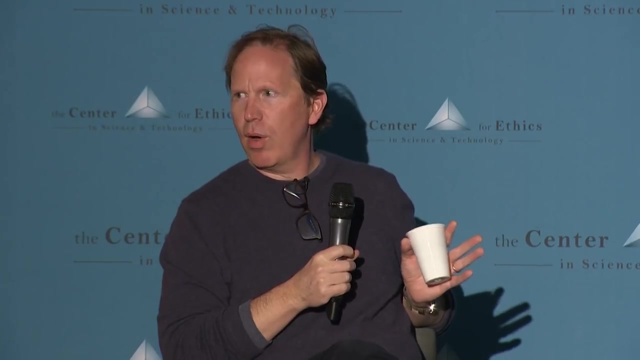 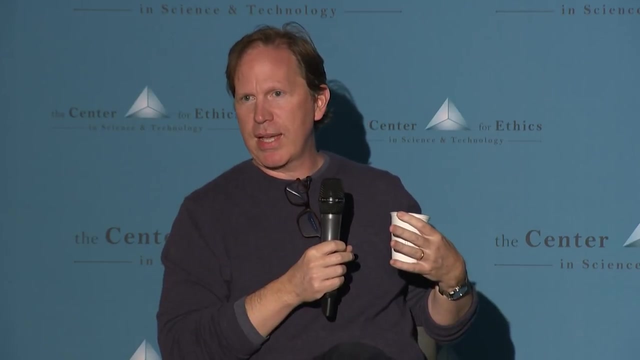 you to subsequently block ads or use a VPN to reduce such spam? I don't think that there is. you have any ethical obligation to desist from using an ad blocker Right. I think you all know that You always have the choice to use an ad blocker, The thing that you need to remember when using. 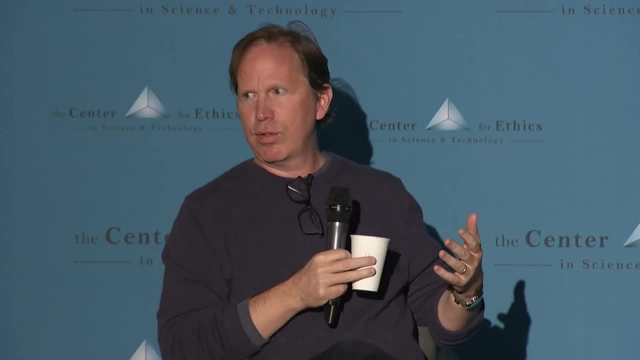 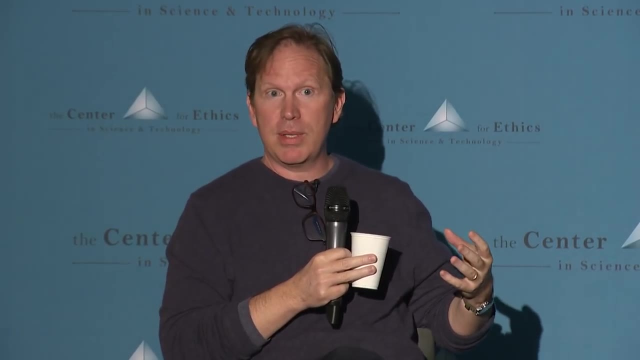 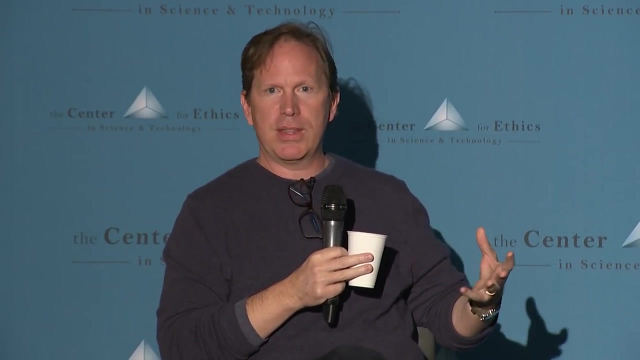 ad blockers is that the services that you use that are free are ultimately being paid for out of advertising. So there is a tragedy of the commons risk that if everyone is very effective at blocking ads, that we will not be able to have these free things, And so 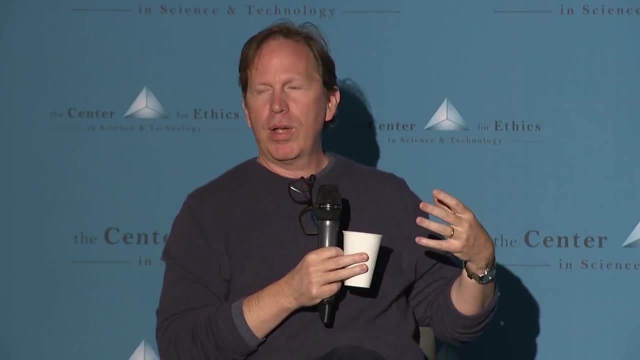 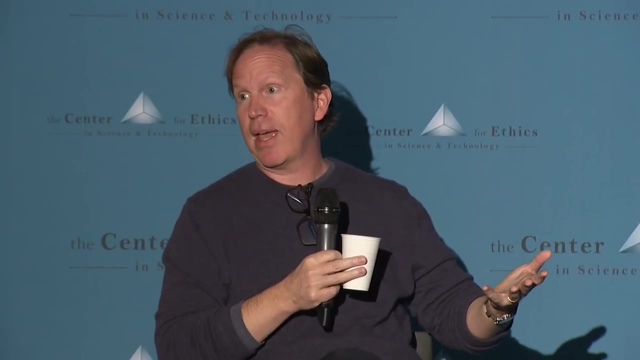 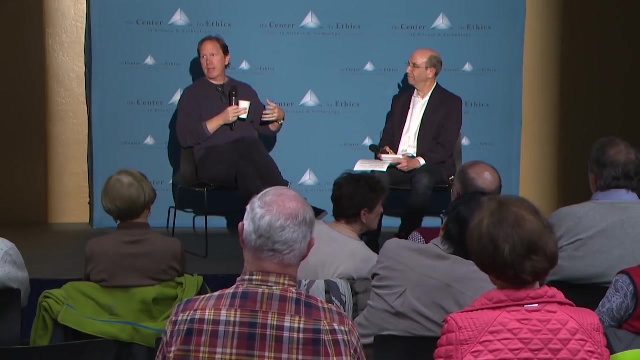 it behooves us to think about. Are we actually willing to come up with another form of payment, like paying direct to have a Gmail account and paying direct to read CNN and paying direct to do that in lieu of advertising, and then we should live our lives according to what we believe And I think. 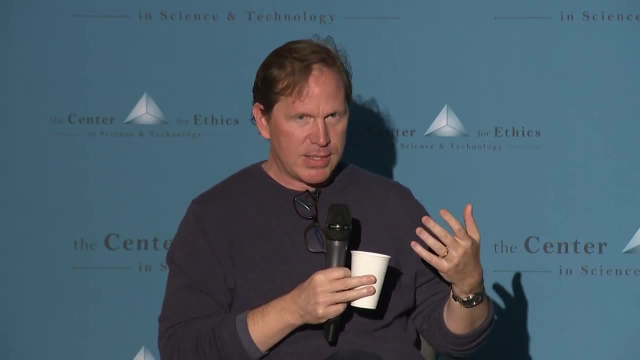 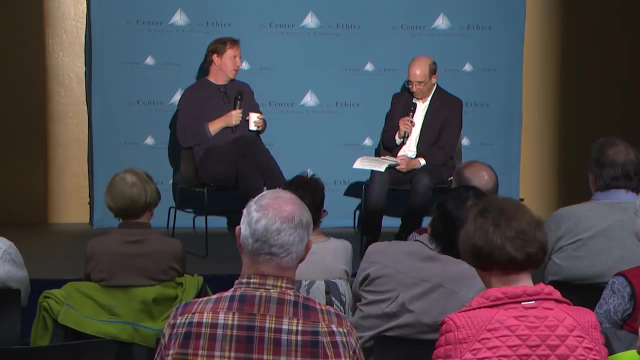 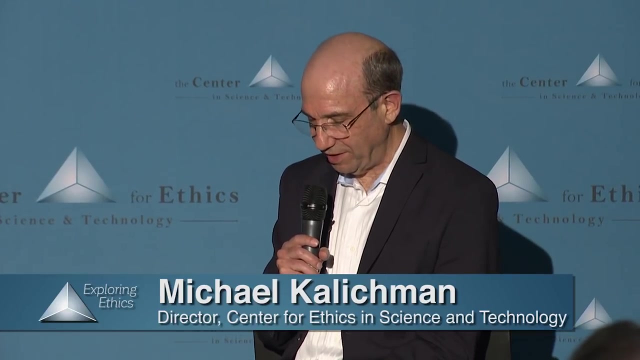 that that's always an ethical thing to do, But it does have an impact. if everyone does it, Yeah, Good. So this person is asking about the process that you go through for these activities, And I suspect it will vary. But they're wondering: at what point would you engage a government? 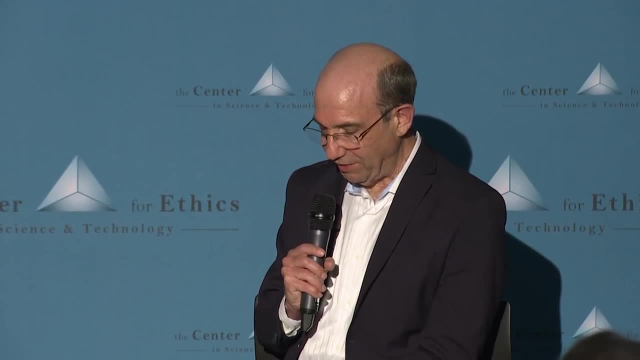 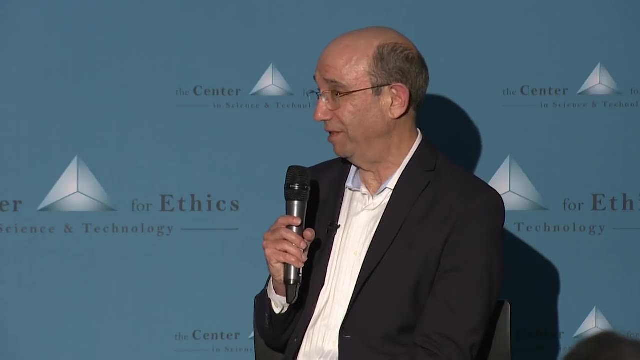 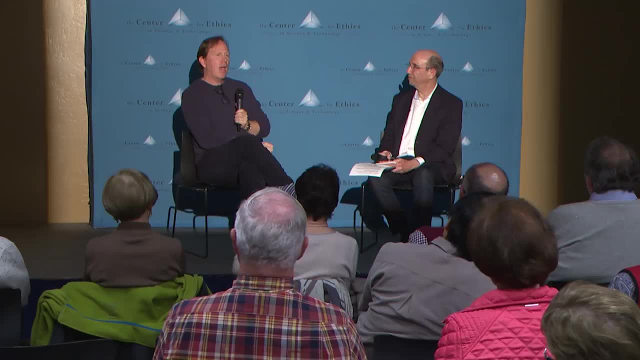 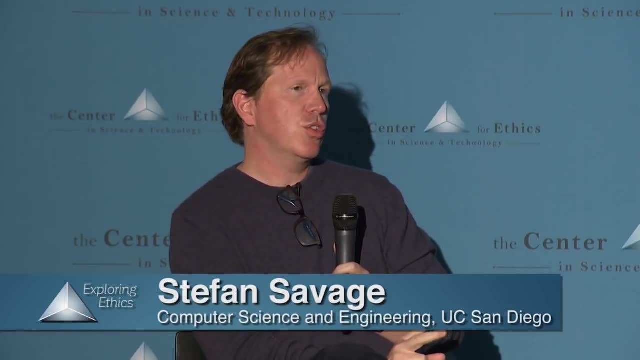 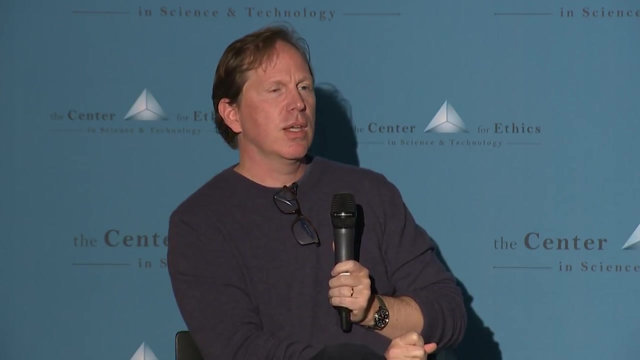 complicated, But it highlights some of the challenges we have in my field. So we did not engage with the automotive industry until we had basically all of our results, And there were really two reasons for that. One is because we wanted our results to be representative of what a 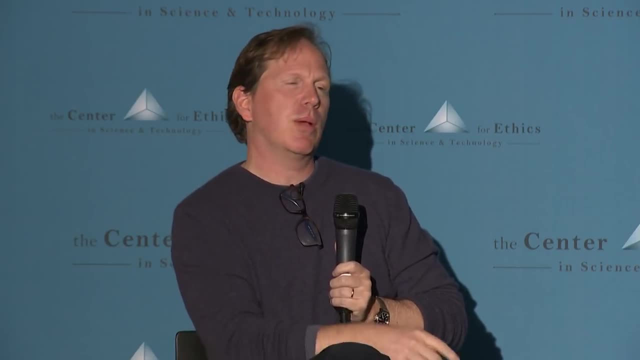 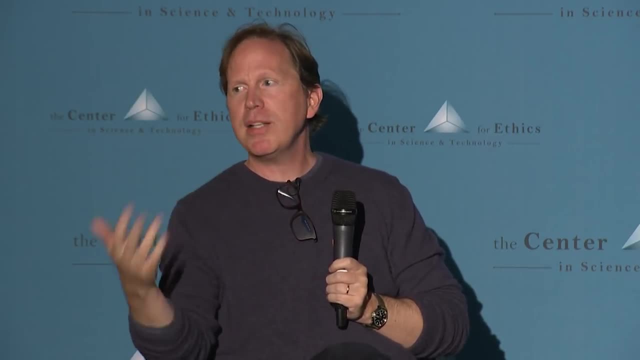 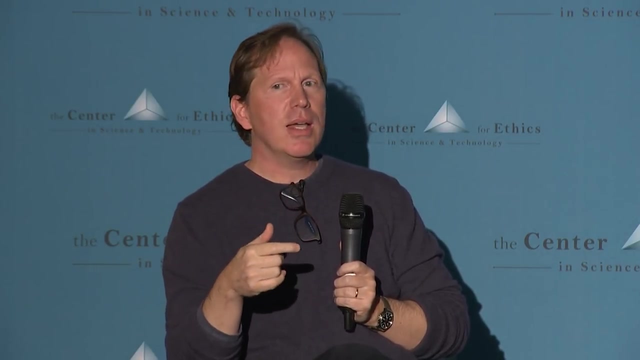 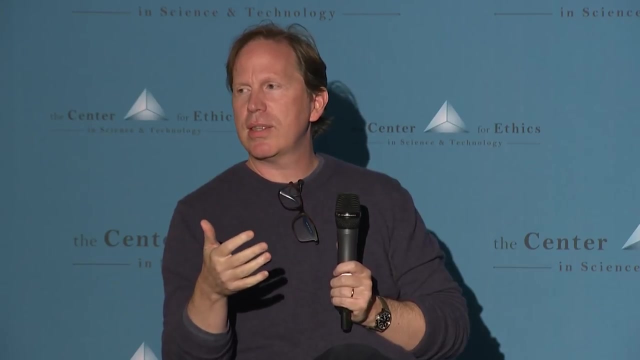 had fully explored. this would be suspect because they'd say: you're sponsored by the auto companies. Why should we trust you? And so we wanted to keep it separate. The other reason is because there are a number of industries in the US that, when you disclose that there, 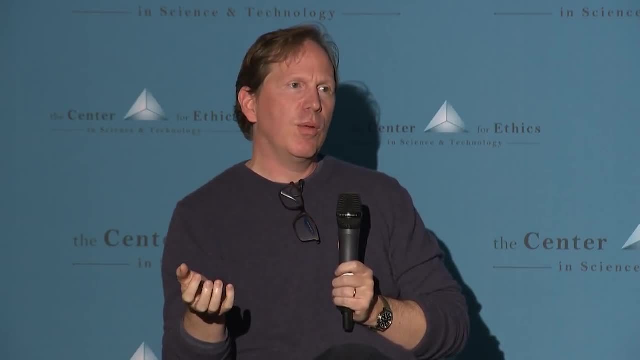 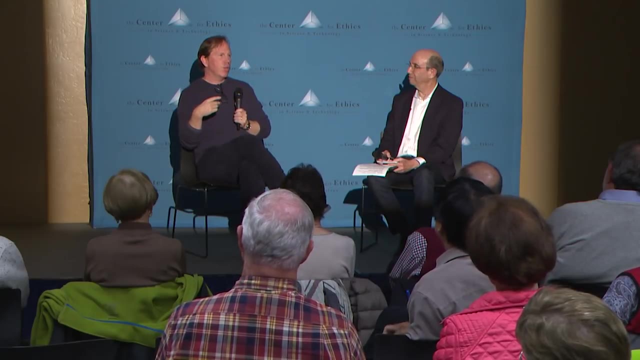 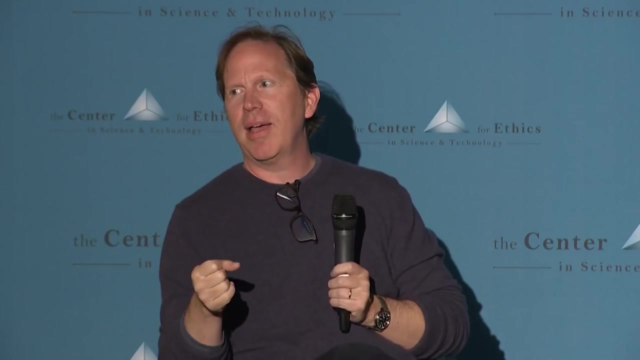 are problems, they will use legal process to stymie you continuing your research, And I know few people who do the kind of work that I do who have not received a cease and desist letter at least once, And so it is much easier to negotiate when you know that. 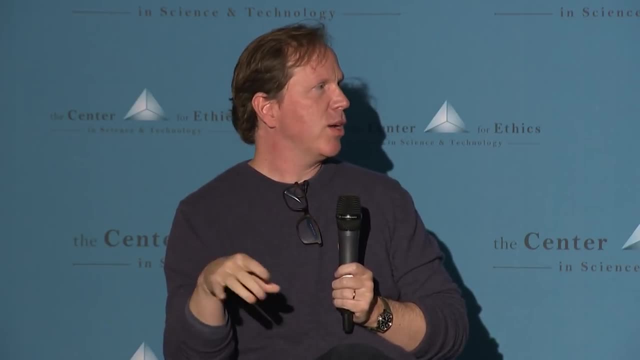 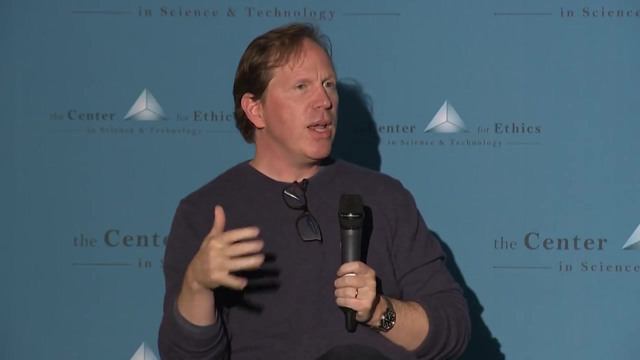 you're going to do it in good faith, Like we never had any intention of naming and shaming or making a big deal. But they don't know that. But we're in a much better position to negotiate an arrangement if we've already done the research, and you know it has you. 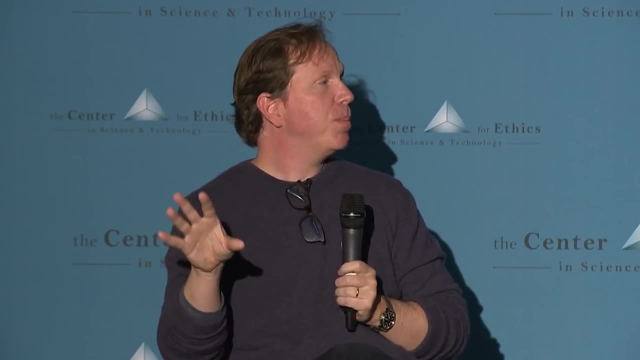 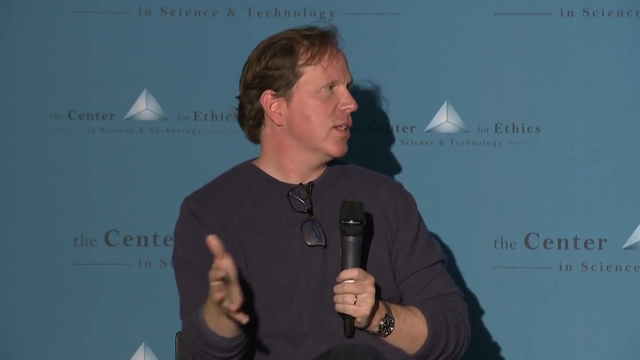 know it has been accepted for publication. And now that's a much bigger deal if they're going to quash a paper that has been accepted for publication. And then we can figure out: okay, how are we going to, how are we going to work with you to best address these issues? 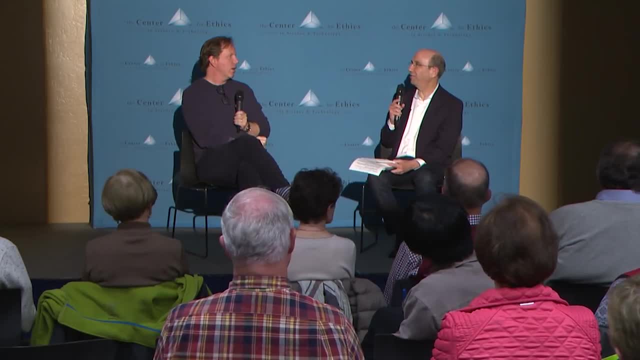 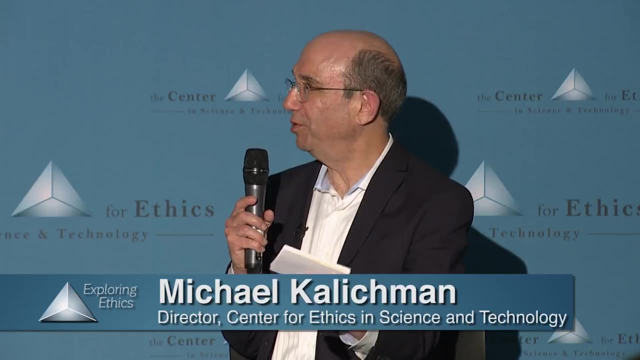 So, given your success, it just occurred to me: I mean, do you now have enough of a track record that you might not have that problem? You could go to the power toothbrush maker that's Bluetooth-based And you could say: I'm going to see if we can take over your toothbrush, And they would 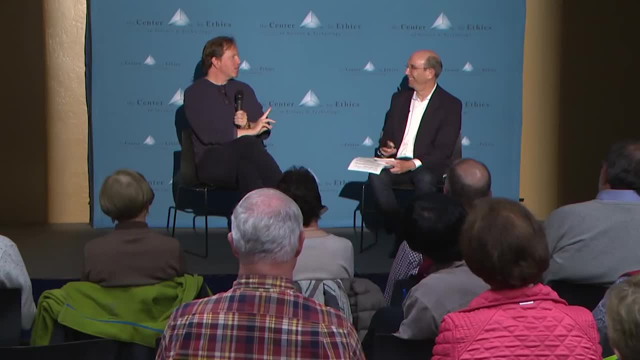 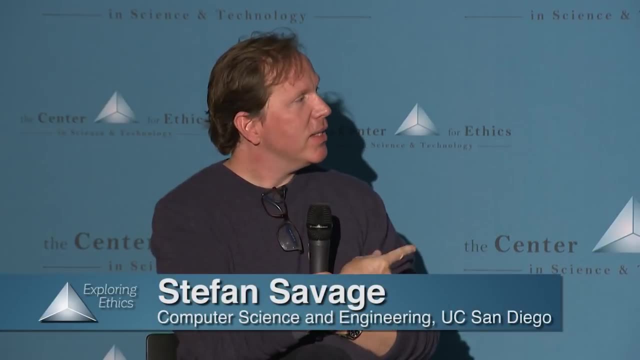 be happy to engage with you because they know you won't. So there are two answers to the question. It depends, All right. So like, and we in fact did this study, We did exactly this study where we went and we took 100 companies. 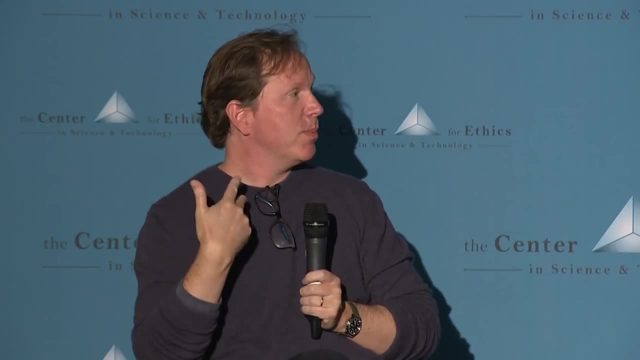 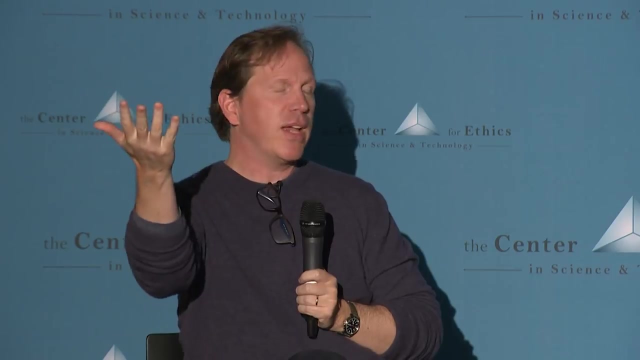 and then we approached them under a variety of different guises- One was me, but then we had independent researchers not affiliated with universities, lesser-known researchers at universities- and said precisely this: Here's your flagship product. We would like to do a security audit of it And we would 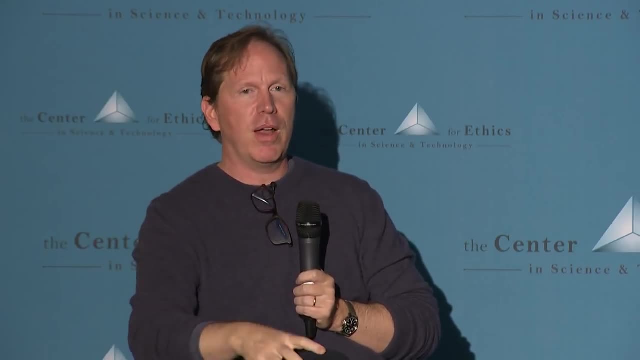 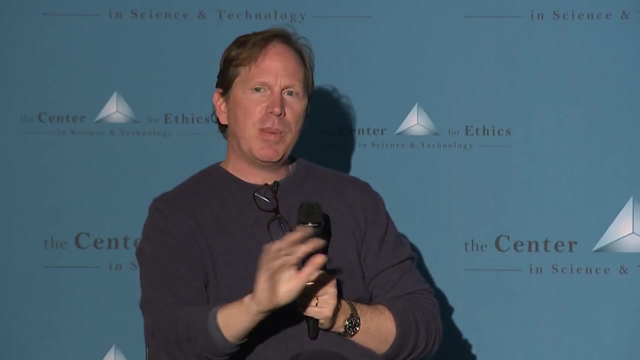 like your approval as a legal safe harbor from violations of any number of laws- DMCA and so forth- And the first thing you find out is that you are in a much better shape if you're a well-known academic researcher than not. And if you are not, then they will. 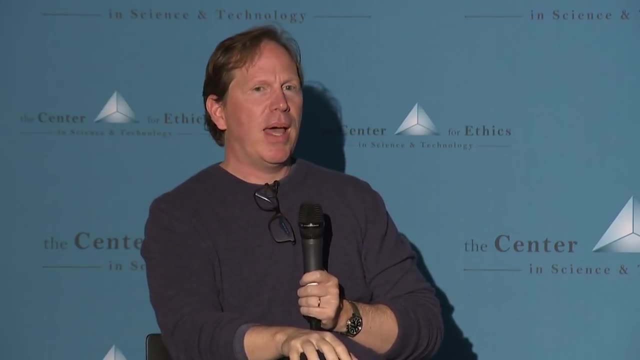 say, go jump off a cliff if they even answer you. But as a university researcher, in particular as a better-known one, you definitely get more engagement because they want to hire your students and so on and so forth. So that's the first thing you find out. And then the 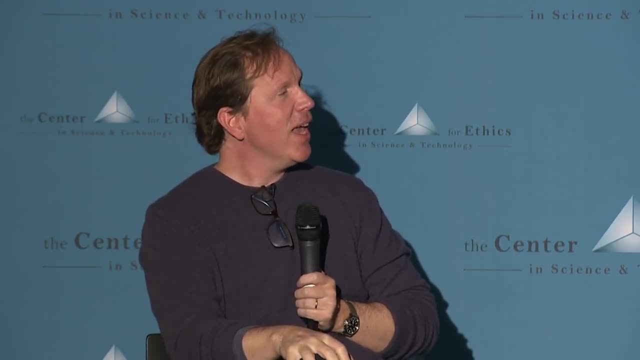 second thing you find out is that I'm a good person, I'm a good person, I'm going to be in a good position, So they're going to be in a good position, and so forth. That doesn't mean that they say yes always. There are quite a few who don't say yes, And it also will. 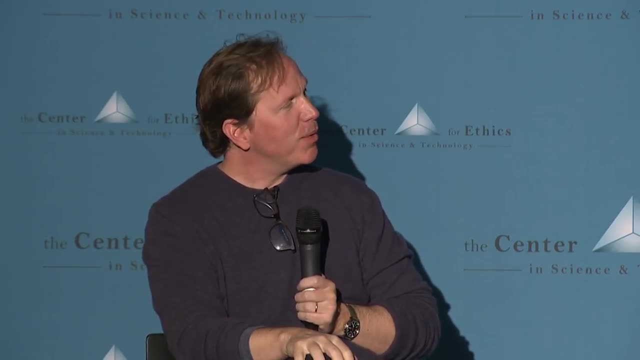 depend on, like the electric toothbrush. I think it's probably a pretty fair game. We do a lot of work in aviation security. Boeing is not showing up with an airplane for us to go and work on. They, I think, would prefer in their ideal world that we would never do. 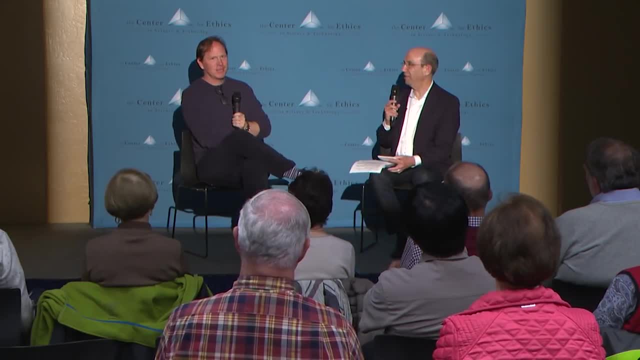 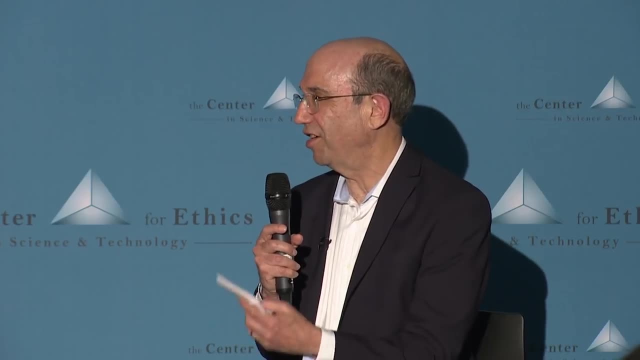 this work. Yeah, so I mean part of that could be the. I mean, if you discover something that allows you, for example, to you know you work out the technology to take over a car or an airplane remotely, you might not have any intention. 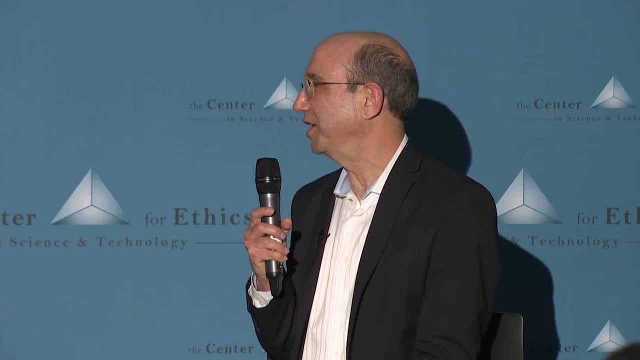 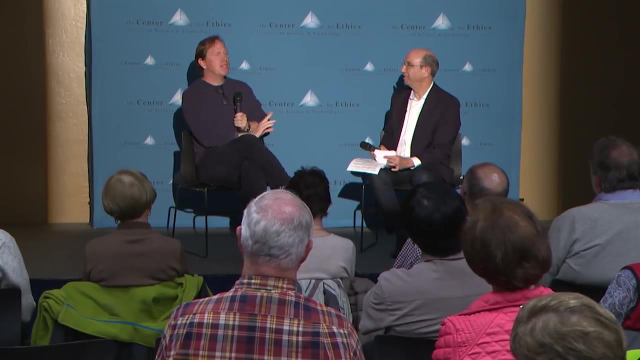 of sharing it, But the question is, how secure is what you're doing? And maybe somebody would be able to get hold of it, So they'd rather not have people looking at that. Actually, in this particular case, I think I am more cynical than you about why they. 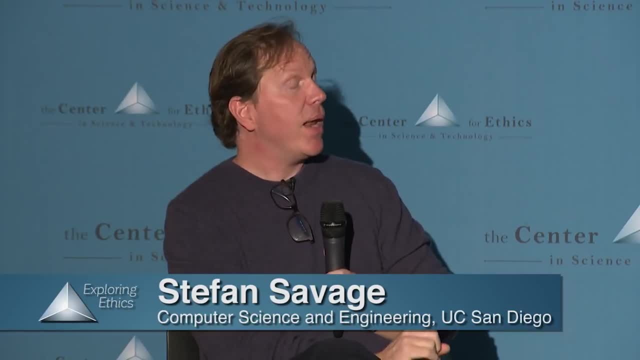 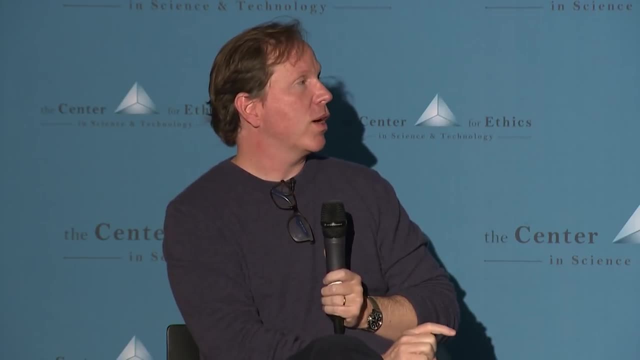 don't want us to, but that's a separate issue, But I do. we actually did spend quite a bit of time in the context of the automotive work, worried very much about the security of what we're doing, Because when we first started contacting government agencies- the places where we thought we would- 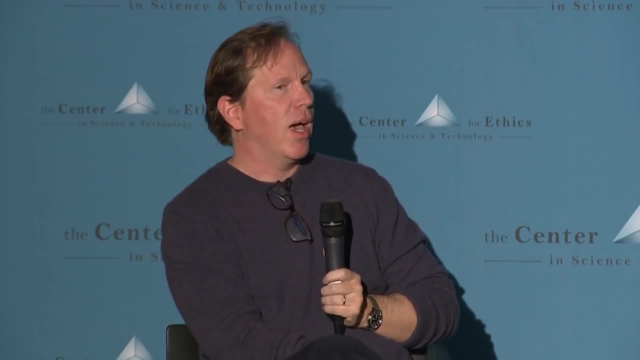 get the most supportive response, which would be like Department of Transportation was not where we got the most interest. We got by far the most interest both from this government and from others on the offensive side who said this is really interesting. We would like to know more. 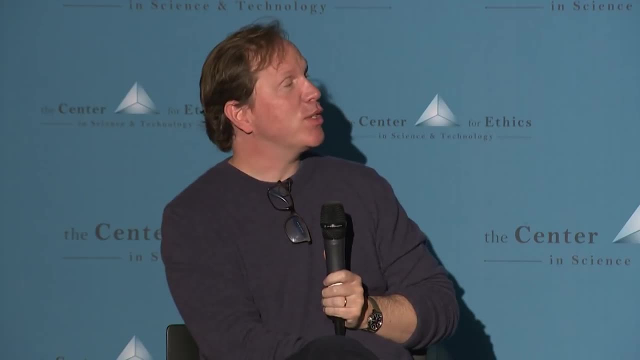 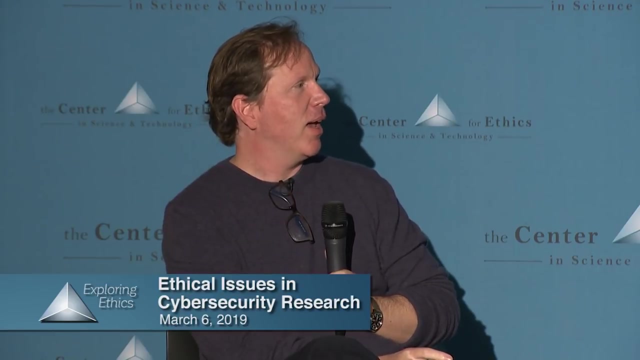 And we didn't contact them, okay, And so we actually went to great lengths to make it very difficult even for ourselves to access the research that we had done, because we were concerned that there was actually substantive. we never wanted what we had done to be used as a weapon. 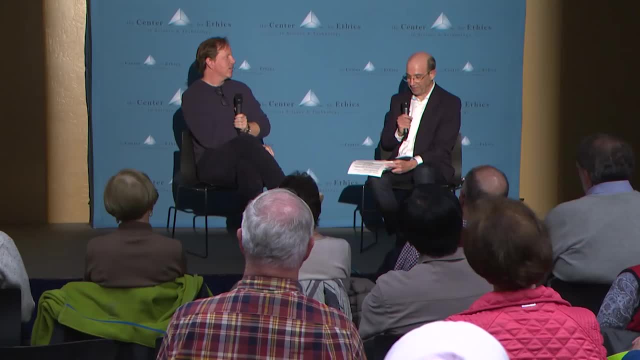 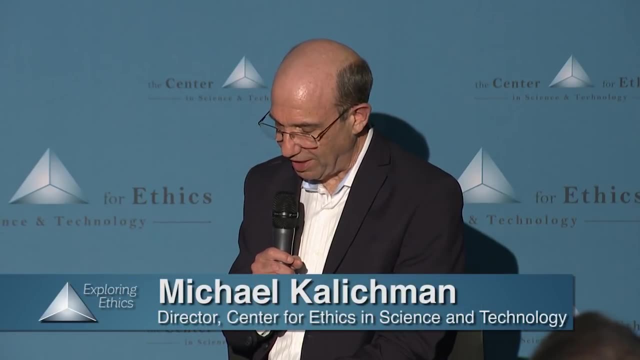 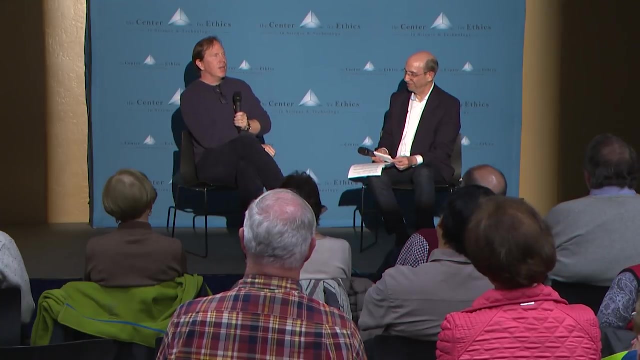 And we knew that there was a lot of interest in that. Yeah, okay, So this. actually, you're going to almost touch on this, but the next question is: do you ever decide not to look into something brought to your attention? If so, what are the factors that you consider? 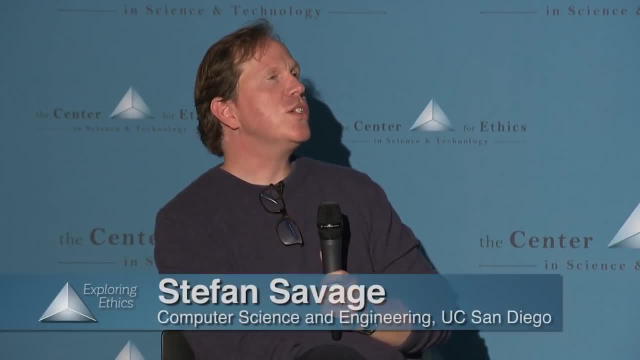 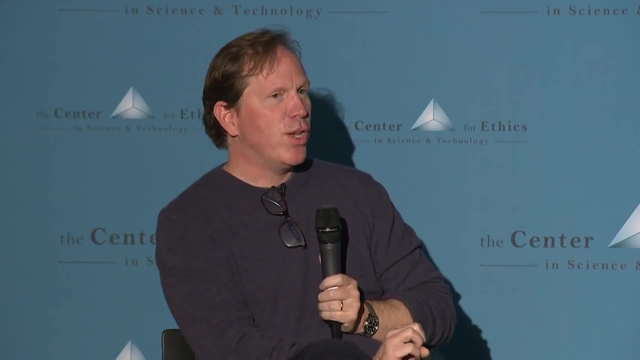 There are questions that we would love to answer that we can't think of an ethical way to answer all right, Where we know perfectly well, Okay, There are a lot of unethical ways to answer them, And so you know that entire like all we, for example, at various points in time, 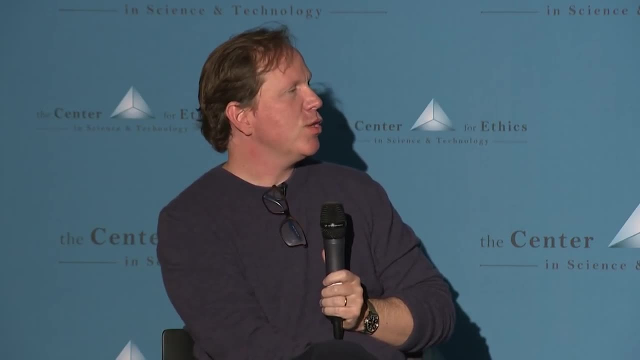 could completely shut down all kinds of botnets, But there's not a legal way for us to do that, And so we neglect, we do not explore that line of research There are. I'm trying to think, though, of something that is closer to what you're I mean, so 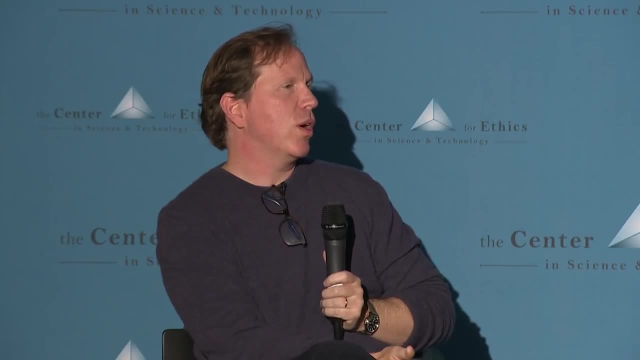 for example, we make a point, not we don't do work on things that are related to any kind of weaponization, because it makes us uncomfortable. I think we have also stayed away, by and large, from research in areas where there is violent. 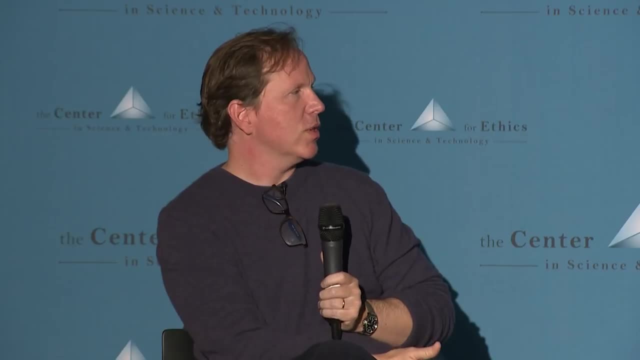 criminal activity, largely because of concerns for students. So we don't want our students to be doing research on something for which the positive outcome of the research would create a call for some criminal organization to be mad at the students. And so those are some examples. 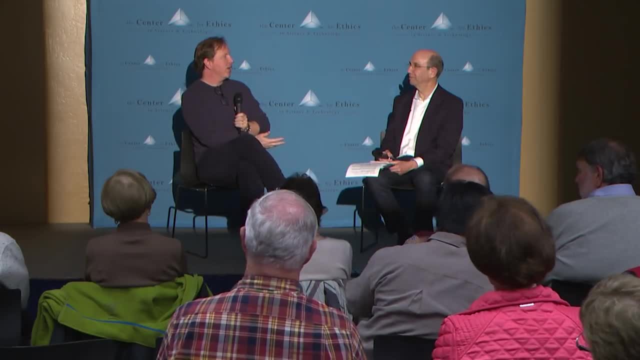 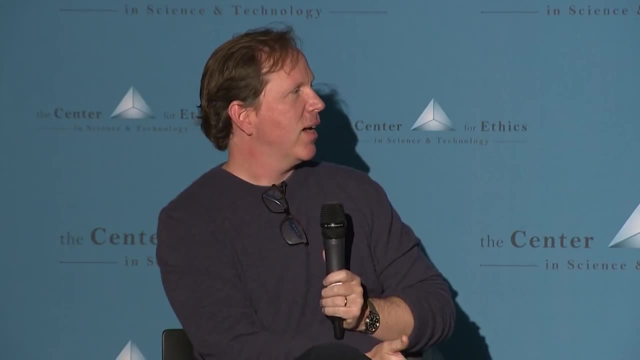 I don't know if I have a general playbook for how we quite a bit- I'll just be absolutely frank- quite a bit of our research is entirely opportunistic. Where you know there are Okay, There will come. you know, you asked previously about how do we engage with companies. 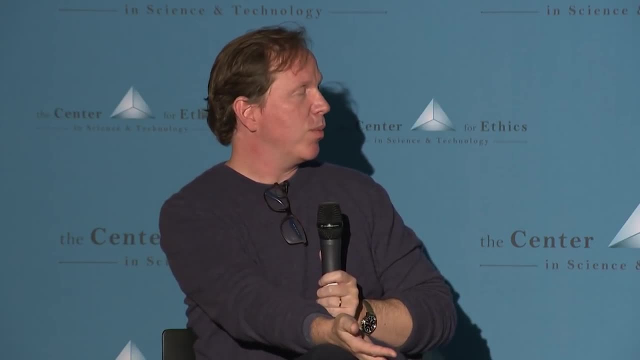 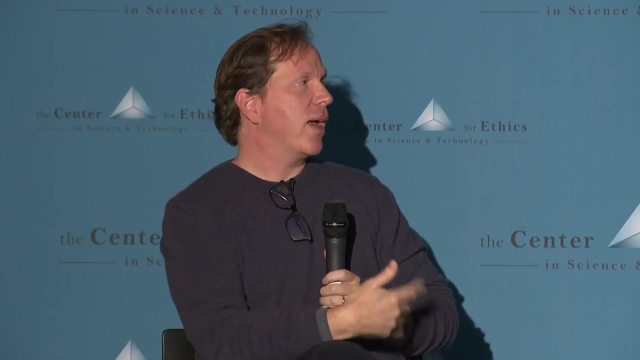 Sometimes it's because we show up to them. here's this thing that we're thinking about and we'd like to do with you. Sometimes we've solved it already and want to tell them about it, But other times they come to us and that's quite common. 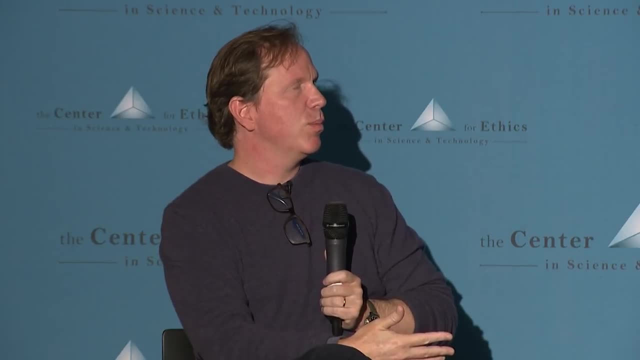 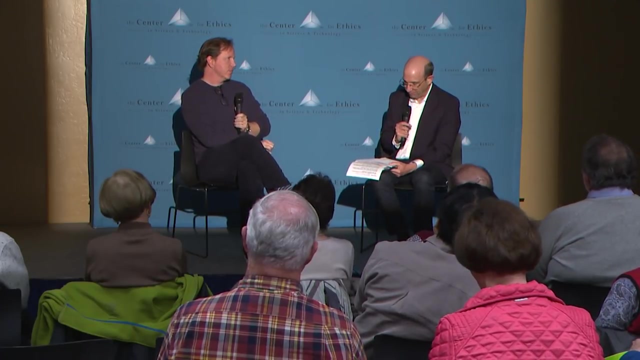 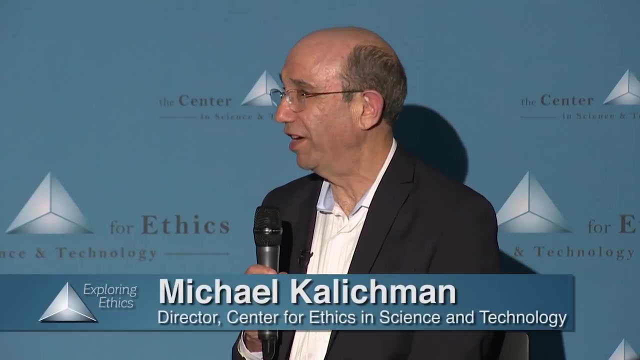 And there are some of those we don't do because you know we don't particularly like the goal. That's on a case-by-case basis, makes a lot of sense. So I know that you are not a policymaker or a lawmaker, but you probably are aware. 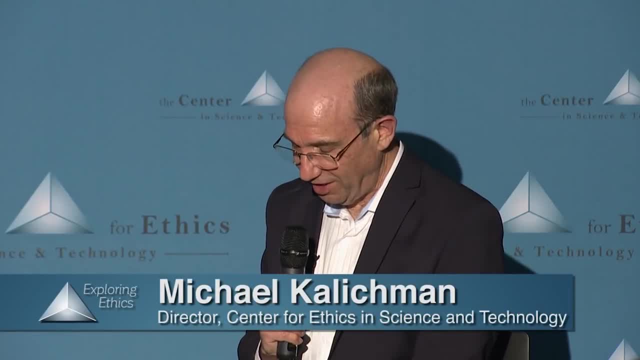 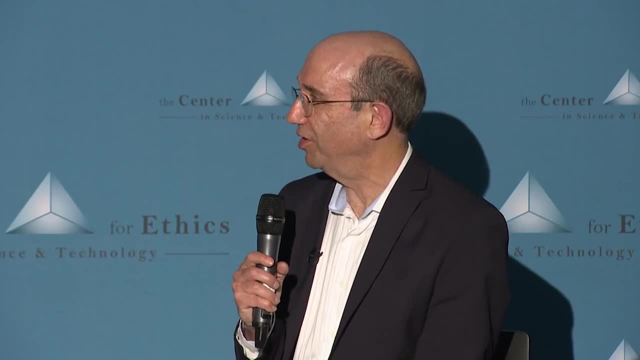 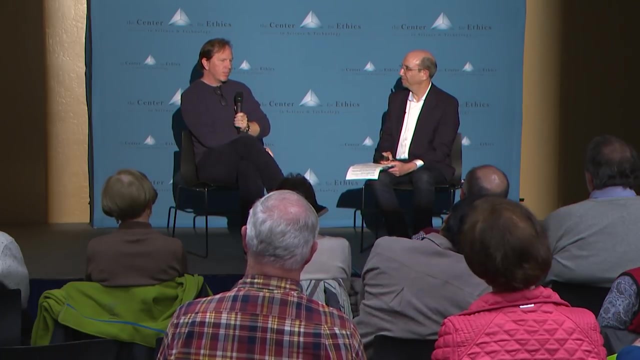 of those policies and laws that affect cybersecurity. So it's a reasonable question: From what you know, how far behind is policy and law in dealing with cybersecurity Are we? Do we have some room, some ground to make up here? This is a very tricky question. 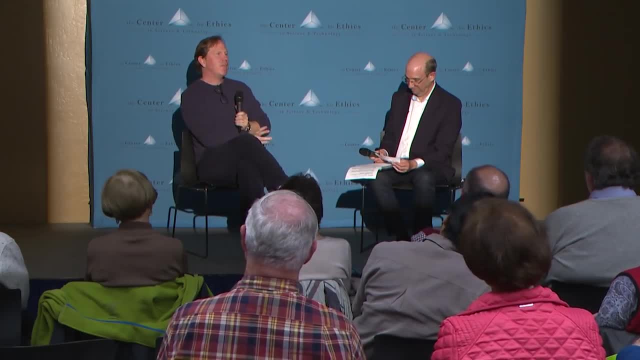 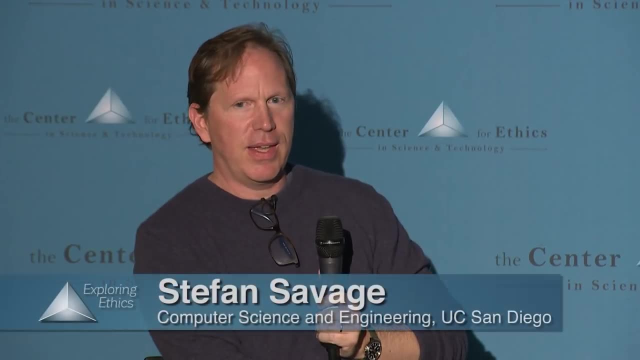 And I used to think it was easy And I'd say, oh, the laws are terrible, I don't know, I don't know, I don't know. And then I spent some time with legislative aides and came to the conclusion: good God. 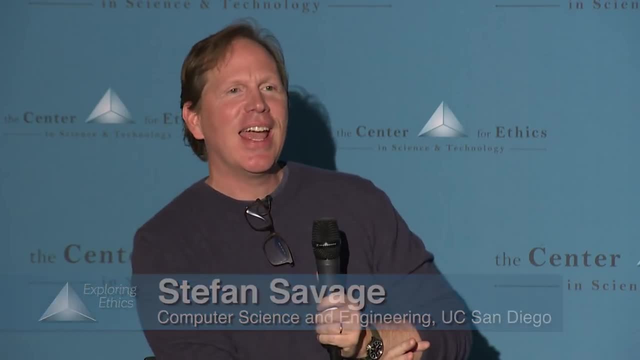 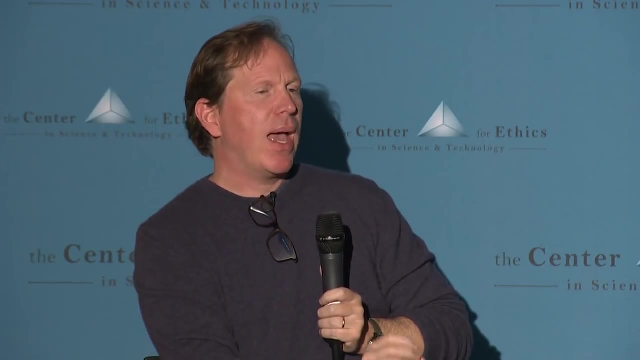 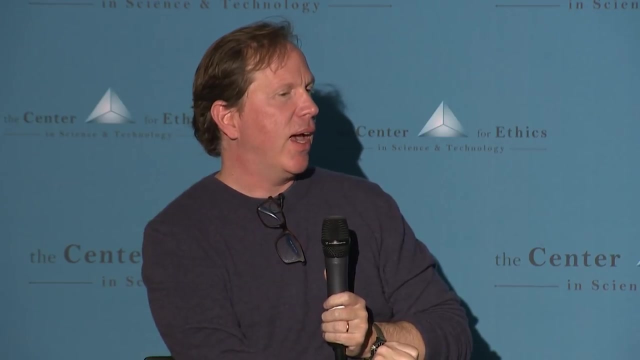 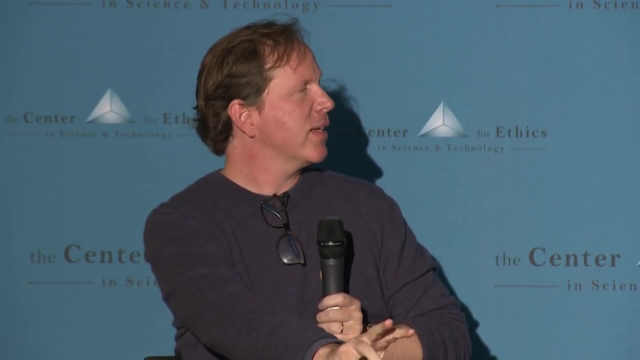 don't let them write any laws. So I think there are different. I'm also not very optimistic about legislation in the current era. I don't think we have a Particularly at the federal level. I don't think we have a coalition of people who are interested in doing the right things. 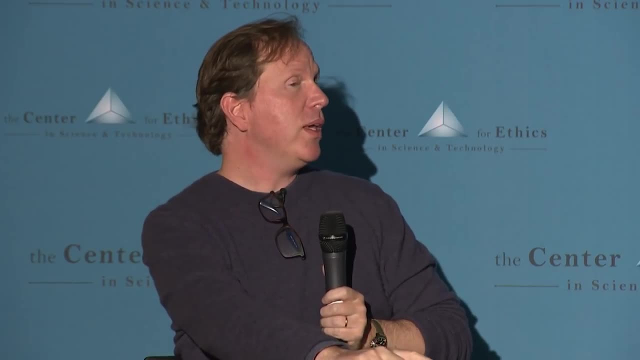 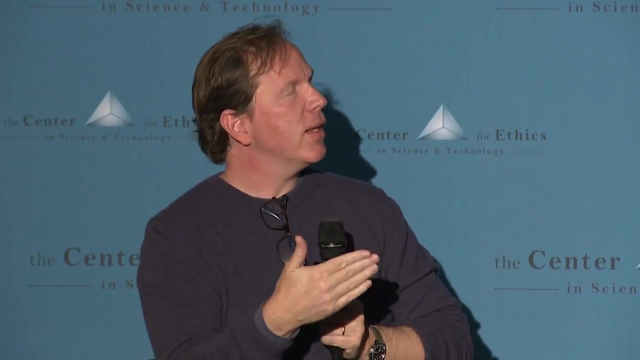 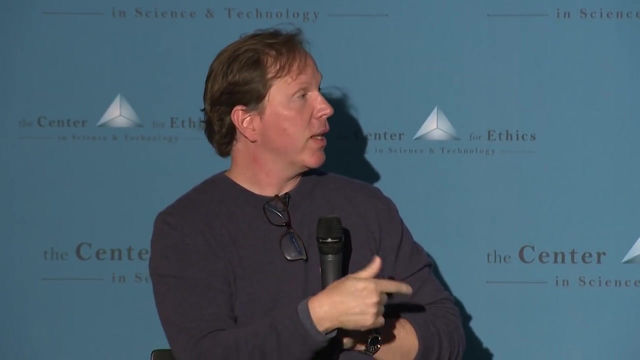 such that law is an effective mechanism. So when we have explored policy options of work that we've done, we've tried to. I think there's an assumption that law is the primary mechanism for enacting policy And a lot of times there's other ways to do it. 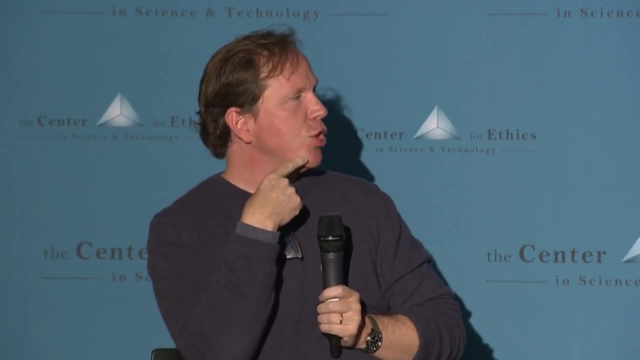 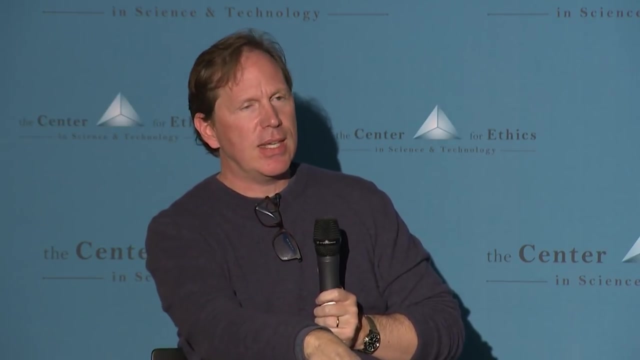 Like this thing that we did with shutting down merchant accounts. that's now a standard technique. Yeah, Yeah, I agree. I think there's a form of legalization that's essential in all of our society, And I understand that there's a legalization of banks, that the standard can be more effective. 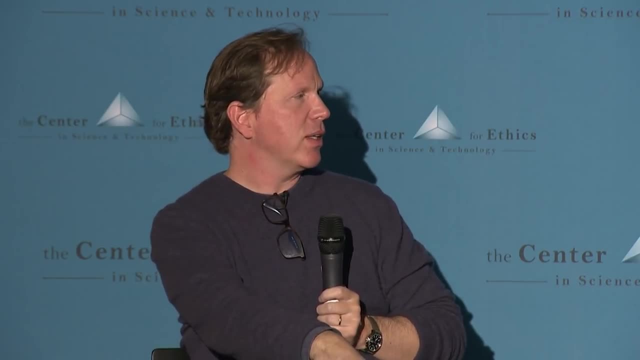 than money can be, but it's also very important to understand what the problem is with, whether they're a large, medium-sized bank or a large, large, large bank that's not easily subject to a certain type of legislation. wanted to ask about the legalization of a bank. The legalization of a bank is not a law. It was a law that the government did not adopted in 1932, but did not involve the creation of any laws. It was the enforcement of existing contract regulations that all credit card companies have with their member companies. 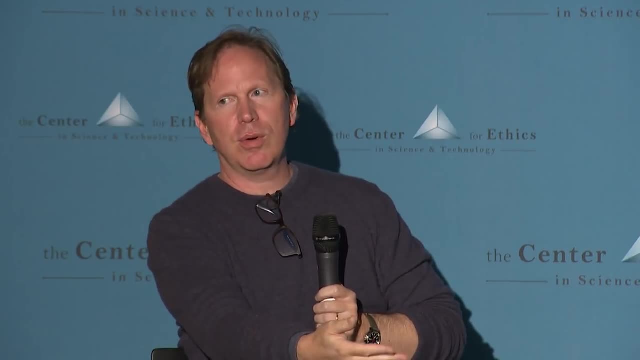 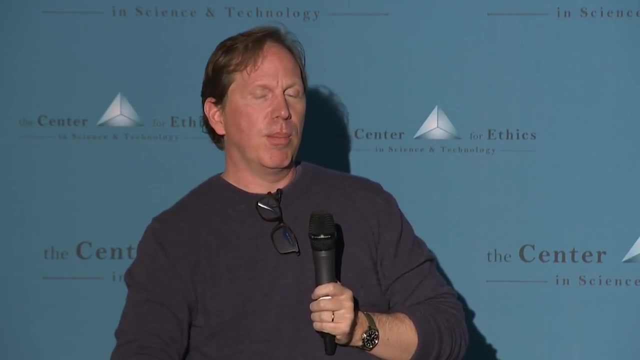 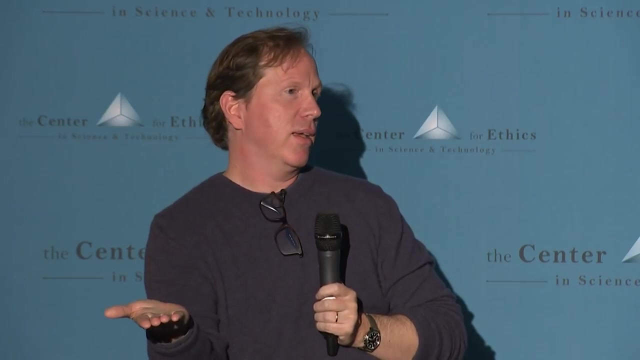 And every bank that is subject to a relationship with Visa and Mastercard agrees that all transactions have to be legal, both in the country in which the merchant operates and in the country in which the purchaser operates, and that, if they don't, that that bank is liable and that Visa 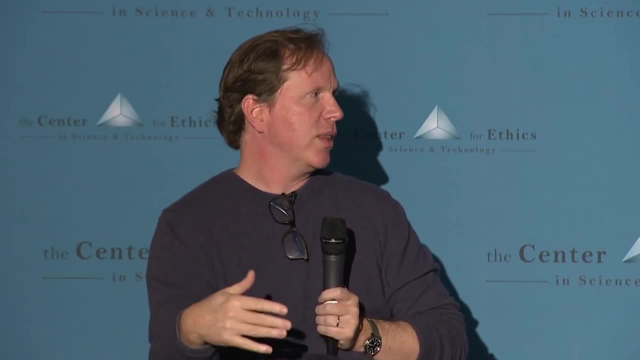 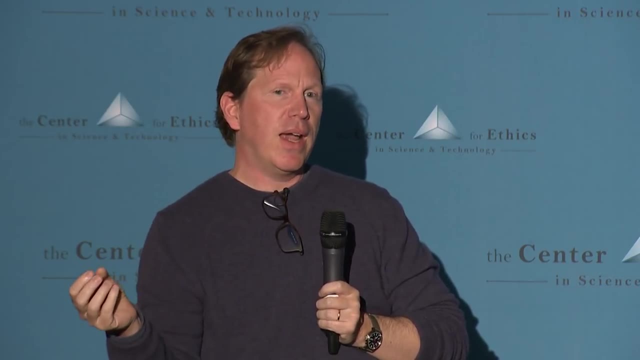 will fine them or shut down their relationship with the association, And so it was just by convincing Visa to enforce their existing rules and then finding the incentives that would get people to hunt down the places where that wasn't happening that got that to happen. Now it could. 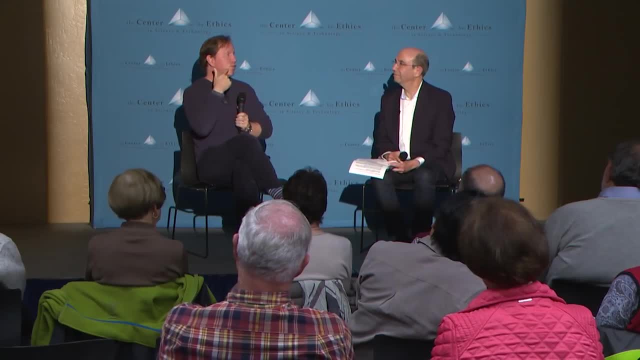 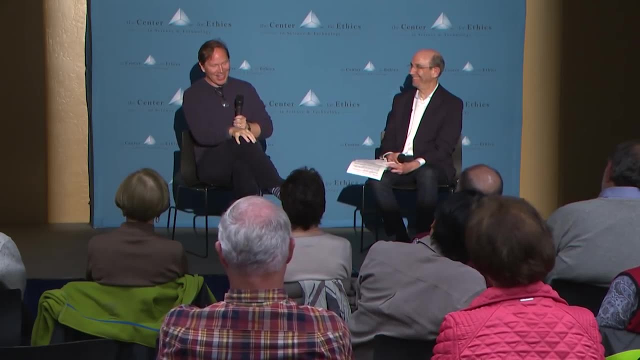 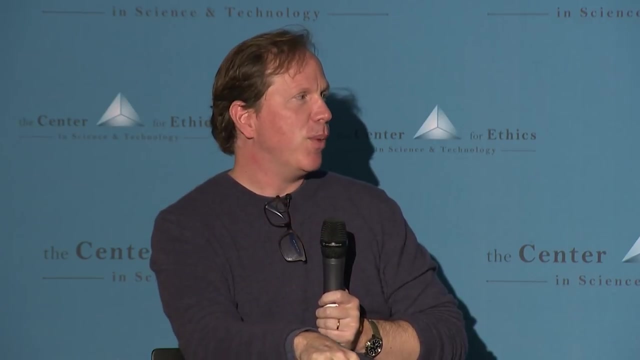 have been done through a law, and I had at least one senator who was very interested in writing a law because, as his staffer put it, he would really like to have written a law, But I don't think that that would actually have led to as effective an outcome. I mean, law is very heavy. 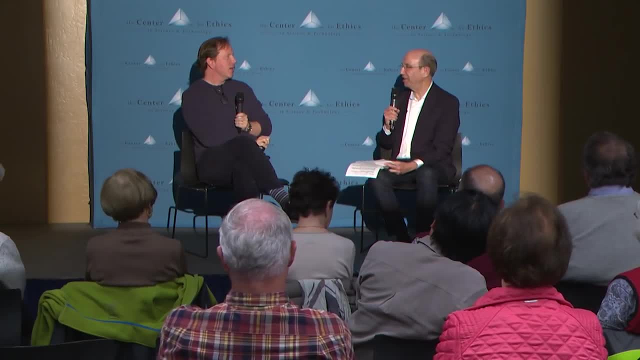 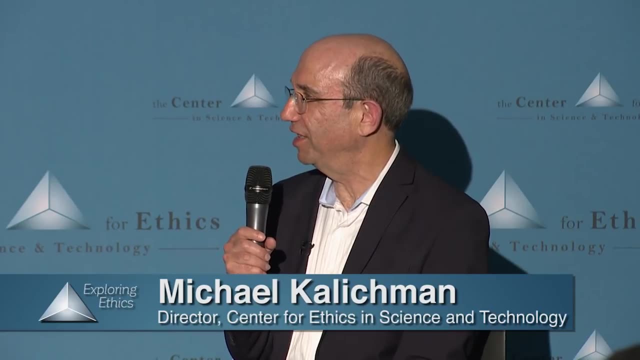 weight. I mean, as you said, that it occurred to me. I mean, the very nature of what we're talking about is so. it's constantly evolving and changing, and law is a very blunt instrument. It might be not. I agree There are some places. 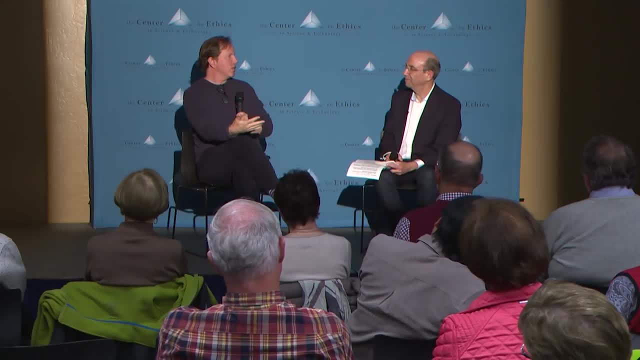 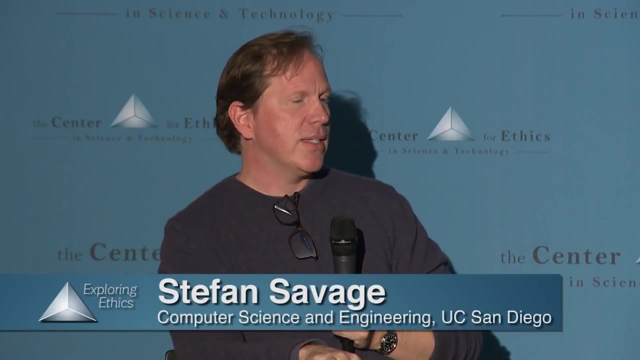 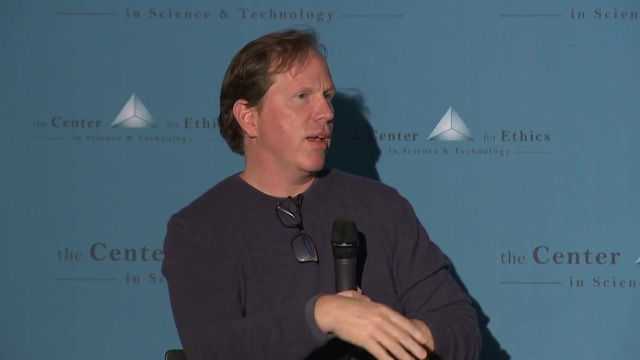 and you have to separate between law and regulation. And so, like I think that there is going to be a realignment at some point, both on the criminal side and on the civil side, in how we deal with electronic information, because there are a few too many problems that we run into We don't have 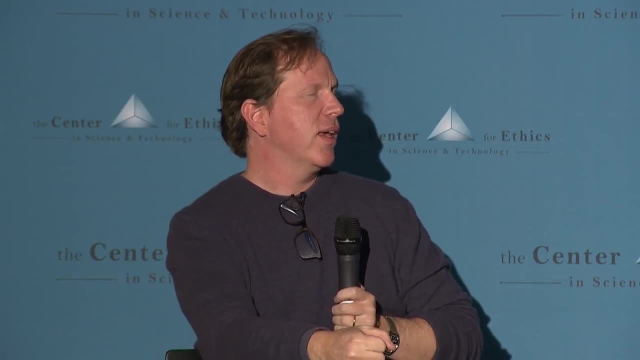 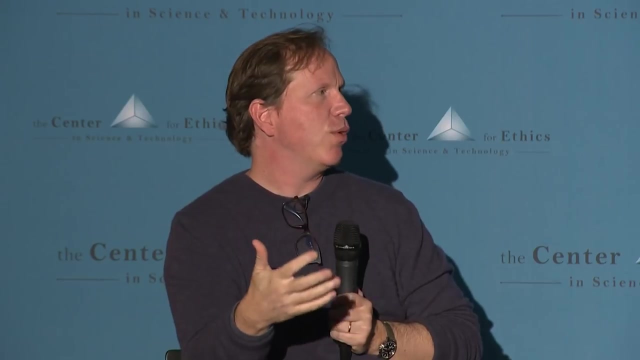 a compelling way to talk about privacy interests under we have a lot of kind of balkanized different efforts to deal with privacy. We don't have a compelling way to talk about privacy in the United States. We don't have a general framework, the way the Europeans have put together. 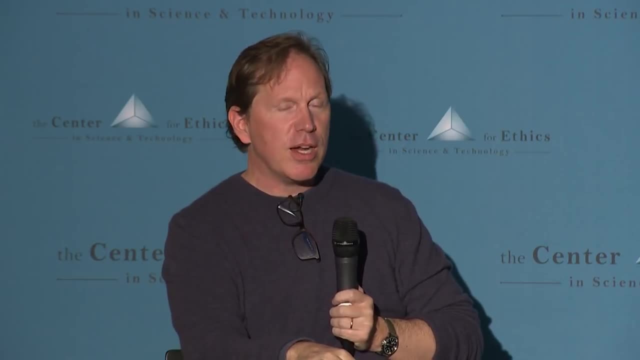 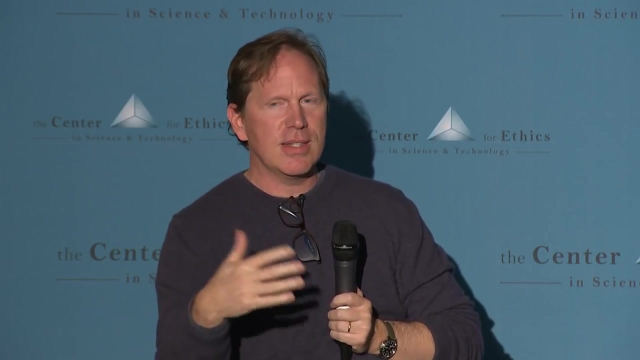 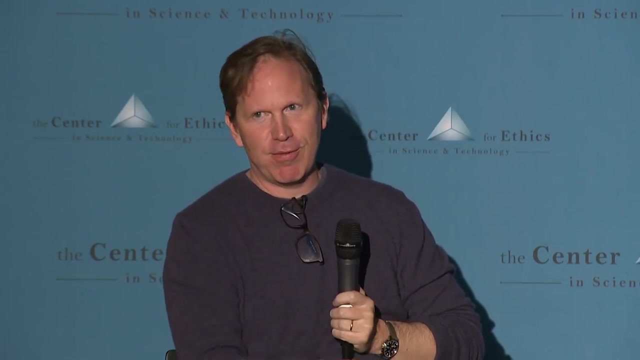 The European framework GDPR is quite heavy weight, however, and presents its own unintended side effects, And so this is not going to be something that happens quickly. So I don't know, I don't have a very nice answer for that question. I apologize to whoever asked it. What I would say: 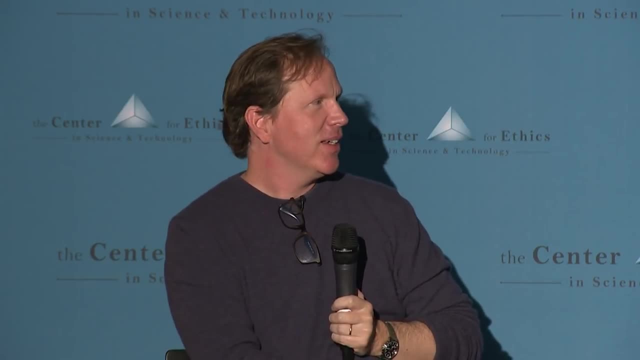 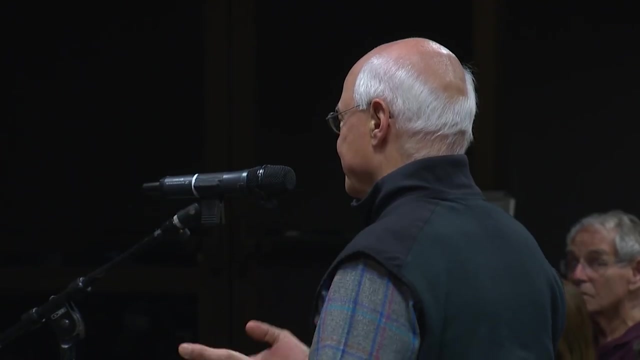 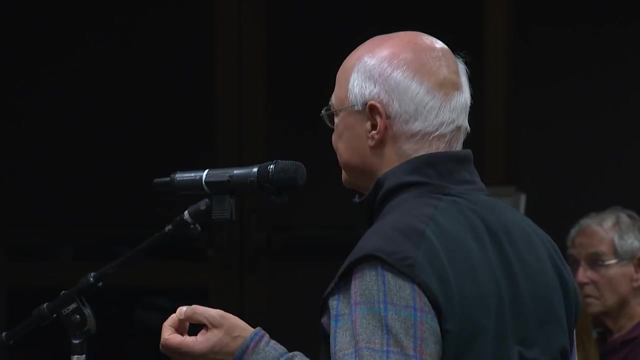 is that it is not simple. It is a very complicated question. Yeah, okay, that's fair enough Question, right? Yeah, a few minutes ago you talked about the difference between controlling taking over a car and taking over an airplane from Boeing, And are there practicalities in this in the sense that 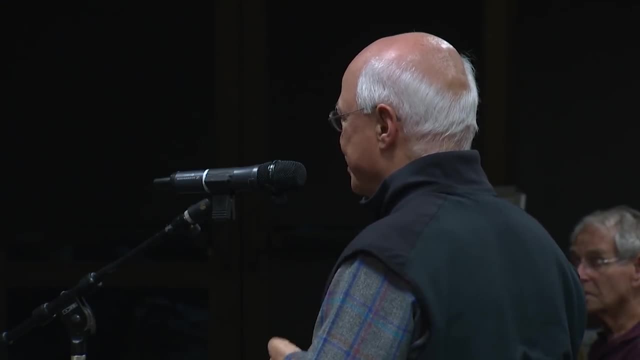 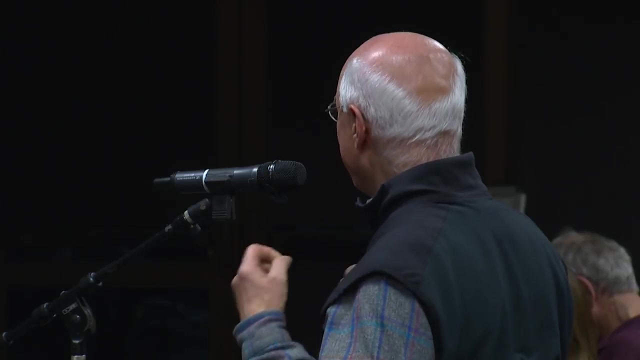 it's one thing to- for a few thousand bucks, I guess, to get the access to a car, an empty parking lot and a few red cones. but A Boeing is probably not going to loan you a plane. You could buy one. 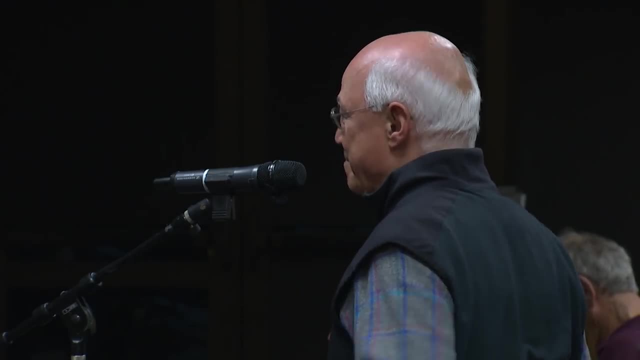 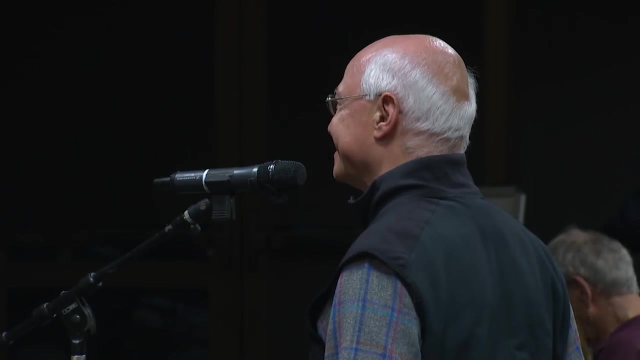 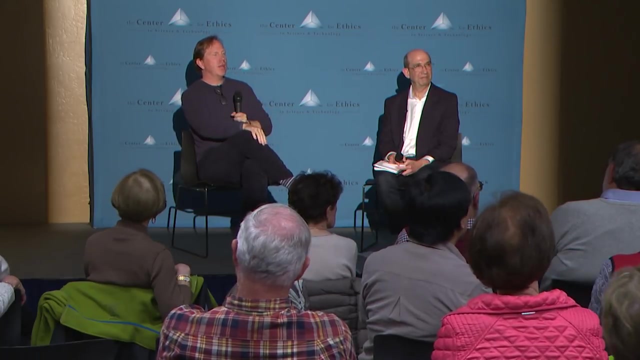 but that would cost many tens of millions of dollars. Yeah, But it's very important. I mean, think about 9-11, how that would have gone if they could- just, you know, take over a computerized plane. I will tell you two things, one of which will- maybe they'll both- make you feel good. The first: 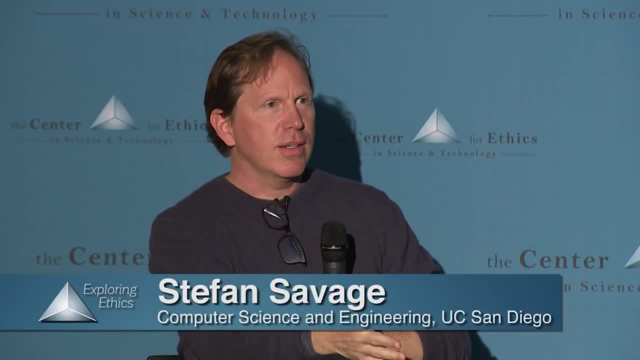 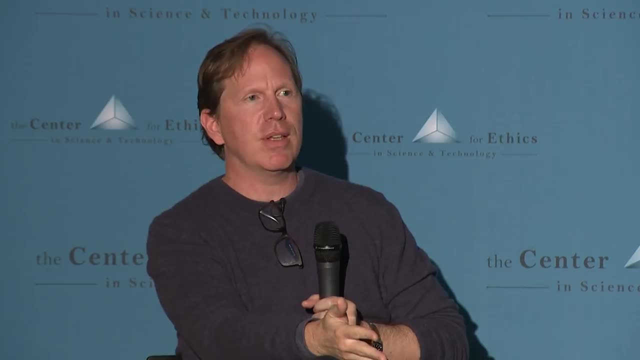 is that it's actually not that difficult, all right, And the reason is the most common transport aircraft in the United States, the 737, it's underlying Avionics. architecture has not changed significantly for 25 years, And so there are a lot of these. 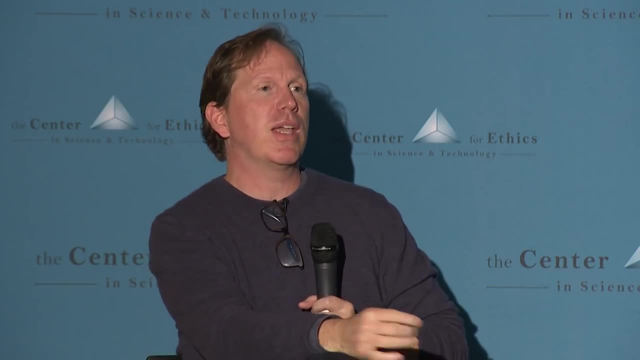 planes that have been decommissioned, And so you can buy the parts that you care about on the third party market quite easily. Now here's the other part, that, if that didn't make you feel good, the situation with planes is much better, all right, And I'll just tell you categorically that planes 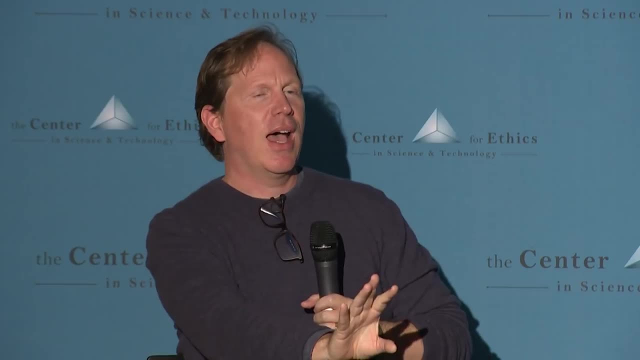 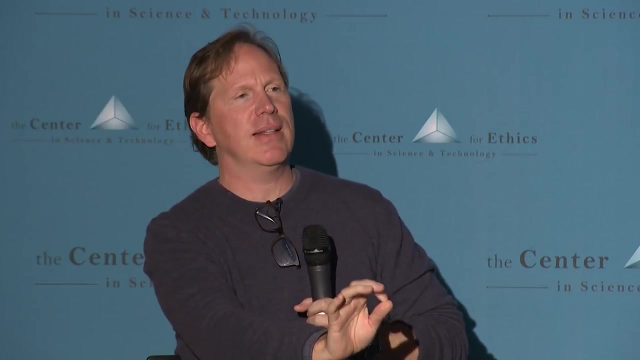 are. the software is incredibly well written And I'm not going to tell you there are no problems, But it is not the kind of thing that you know. a couple of kids in the afternoon will figure out how to do this, And there will. we are unlikely, based on where our research is so far, to have